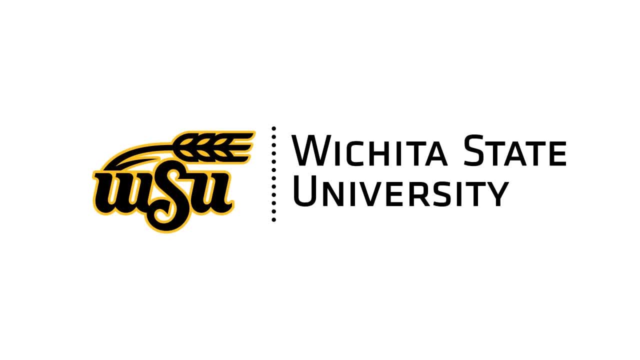 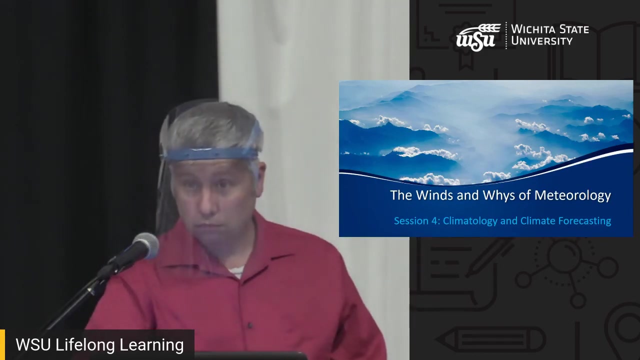 Thank you. All right, everyone. We ready to get going on the last class, Or the last day of this class, I should say, And this is kind of where we wrap all of the three previous weeks together. We talked about kind of instrumentation. 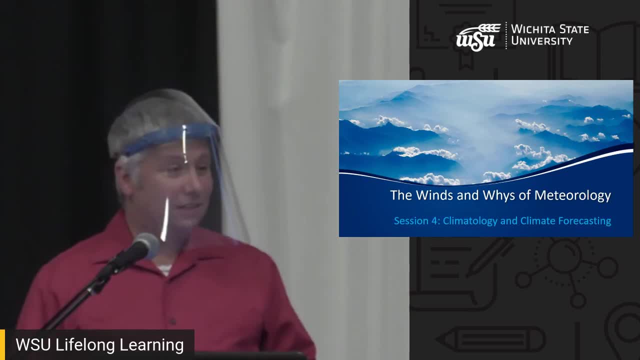 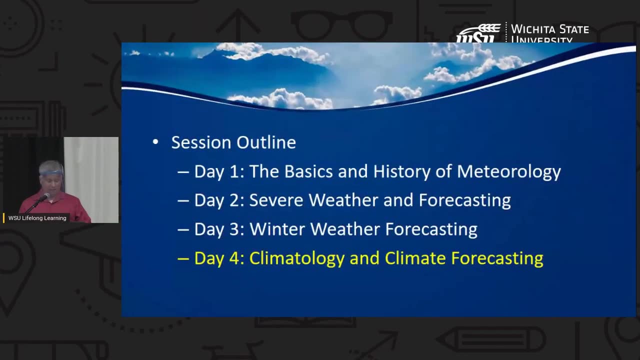 Then we talked about storms, Then we moved into- well, let me double check, I haven't had my caffeine today- Then we talked about winter weather And now we're wrapping up, looking at our climate past and future and forecasting and things like that. 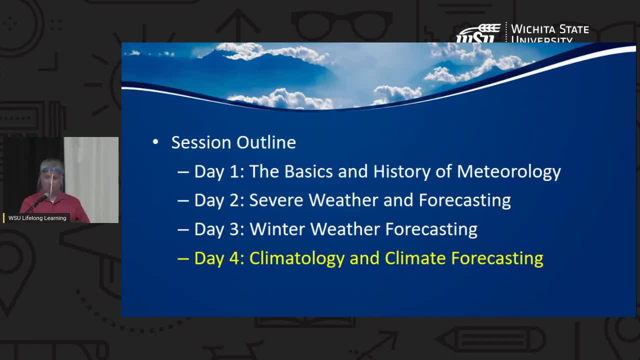 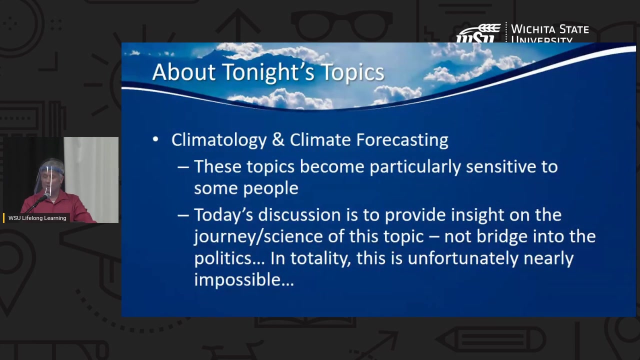 This always tends to be the more, probably one of the more interesting classes, in the sense that it is nearly impossible, unfortunately, in today's world, to agnostically talk about climate without getting involved with personal politics and things like that. But we will do the best that we can. 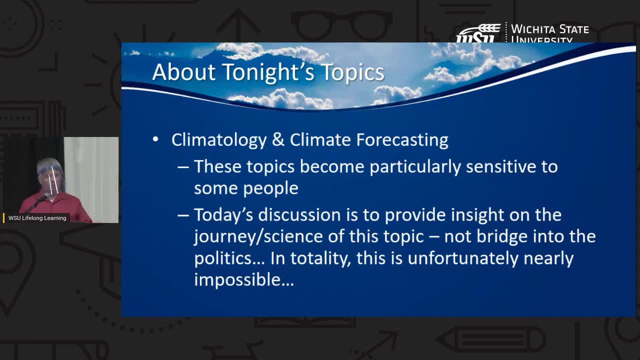 I just raced past my slide on housekeeping By session four. we should all pretty well know that housekeeping, But just in case you've forgotten over the last week- masks on all that good stuff- I will try to remember. and people just throw stuff at me. 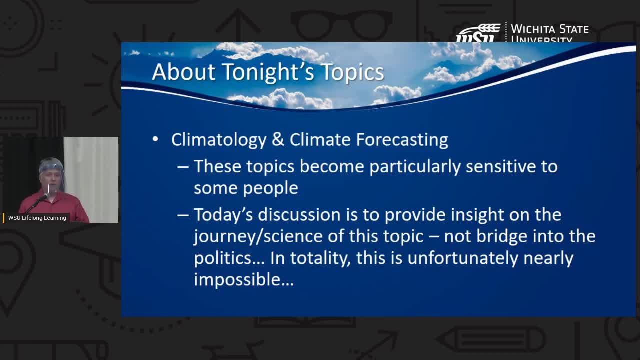 to repeat your questions when you ask them here. Those of you out there watching at home or wherever you are, go ahead and send your questions through via email. We will get to them as we get through the class, This one I explicitly put together to hopefully allow for a lot more question answer. 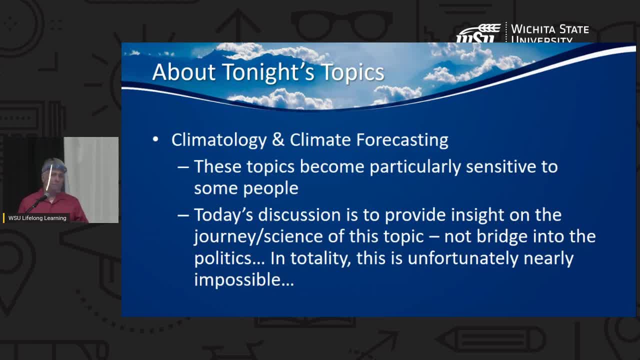 that sort of thing discussion, because that tends to come out in this class a little bit more, because it is such a hot topic And it's also a topic that a lot of us really don't fully know about. So I'm going to go ahead and get started. 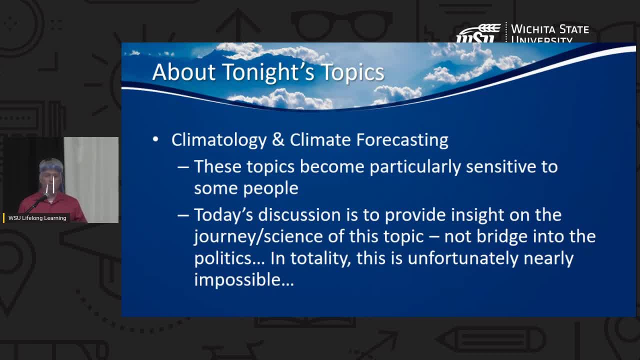 I'm going to go ahead and get started. I'm going to go ahead and get started. I fully understand day to day. We know most of what we know about climate and climate change from talking heads, more than we necessarily know from science. So we're going to get below the surface. 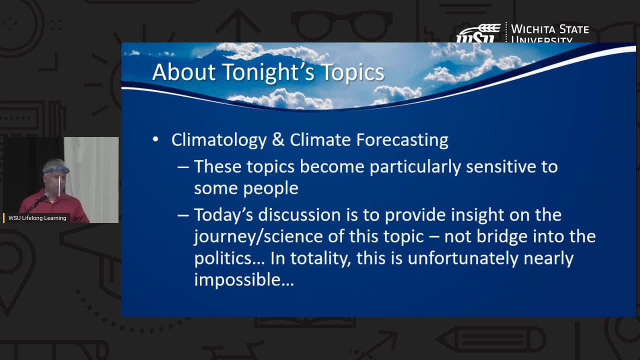 We're going to talk about what climate is. Is it changing, How is it changing, Are we responsible for the changes, And how we can make that argument from multiple directions- pro and con- And so this gets to be a lot of work. 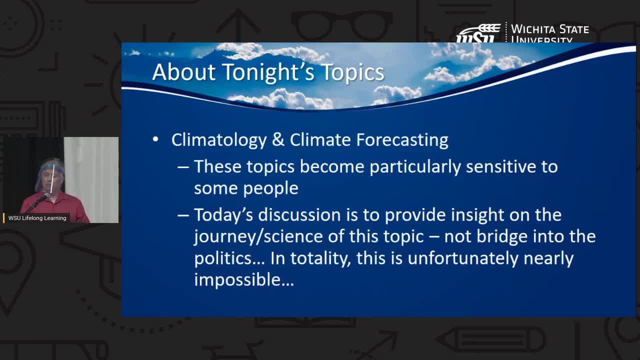 be a really interesting class sometimes, So feel free to ask questions, get involved in the conversation and we'll go from here. I also have a lot more videos in this class than I do in the other ones, because I like to let some other people do the talking for me on this subject. 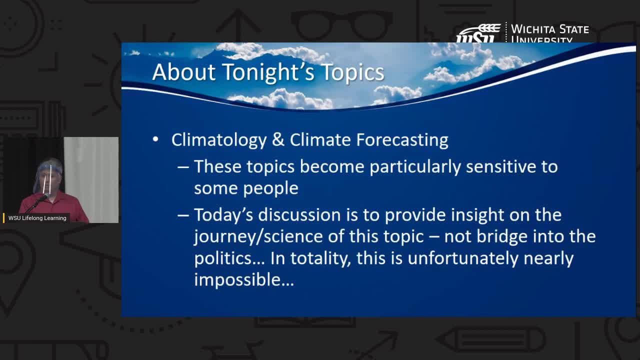 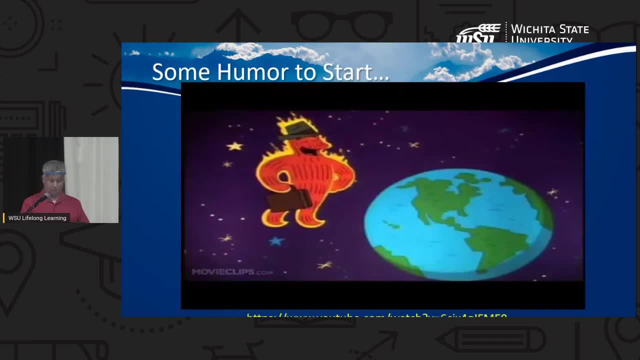 because there are a variety of perspectives that come into the conversation. First, though, oh, ah, okay First, and hopefully it loads my YouTube video, because it said it was supposed to on here. If not, we'll have to go the other way. It's supposed to automatically play it this time. 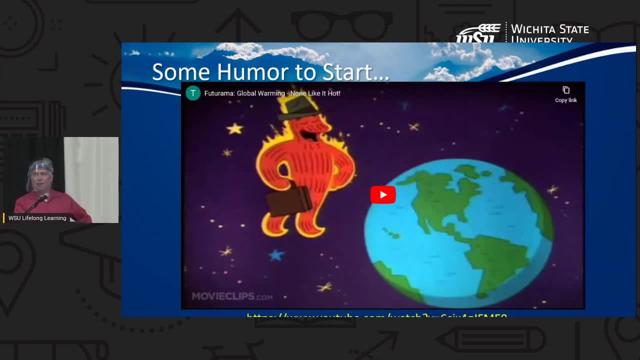 Okay, there we go. All right, just kind of start out with some humor. This is from the show Fearless Futurama which was on in the late 90s into the early 2000s. It was a satirical. 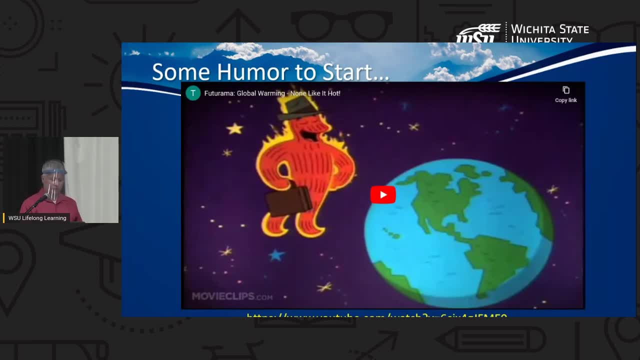 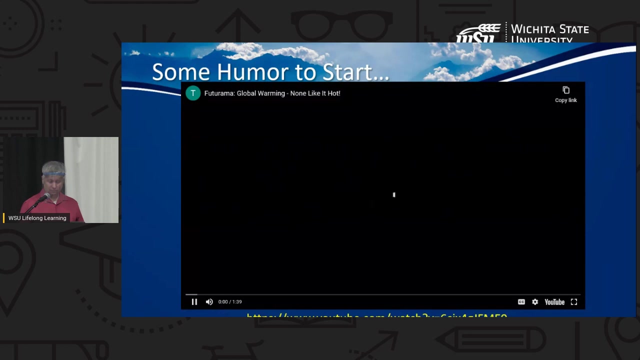 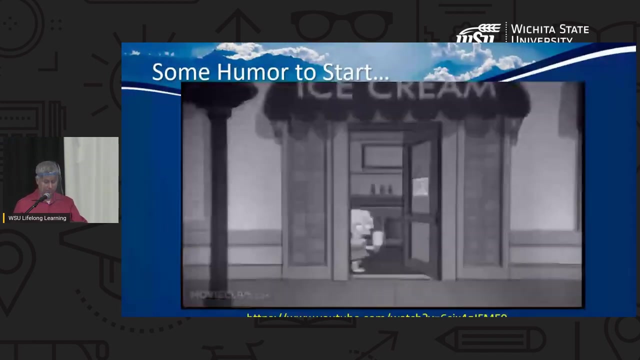 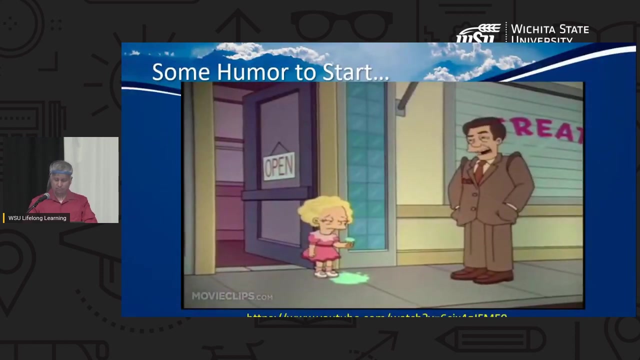 cartoon comedy with a lot of interesting humor to it. This is a satirical but kind of an accurate cartoon way of explaining what global warming is in general. Global warming or none like it hot. You're probably wondering why your ice cream went away. Well, Susie, the culprit isn't foreigners. 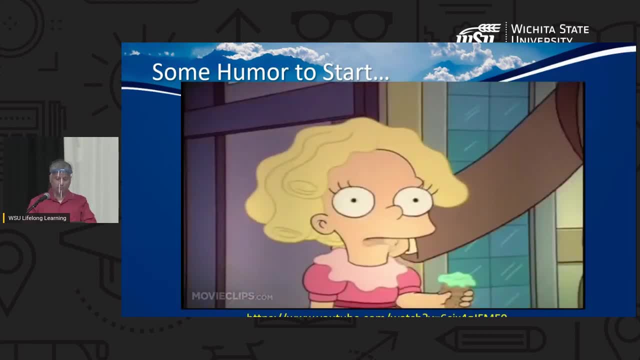 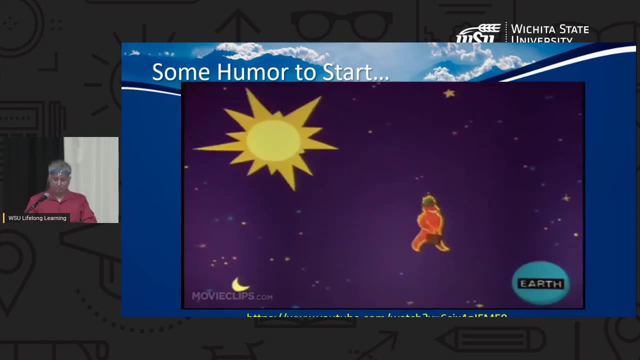 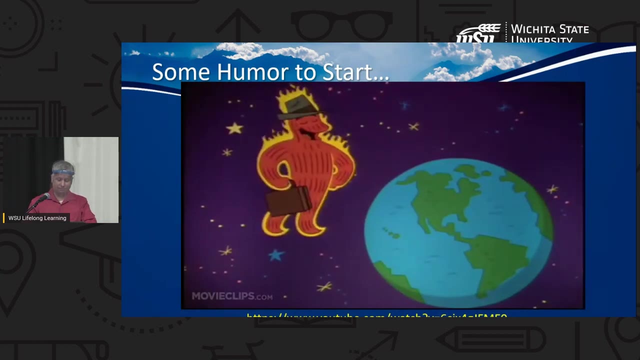 It's global warming, Global waffle. Yeah, Meet Mr Sunbeam. He comes all the way from the sun to visit Earth. Hello Earth, Just popping in to brighten your day. La, la, la, la, la la la. And now I'll be on my way. 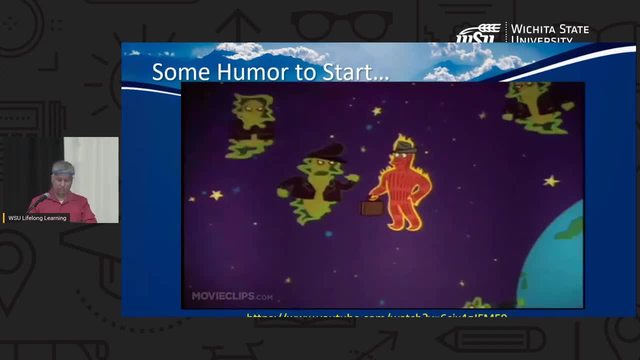 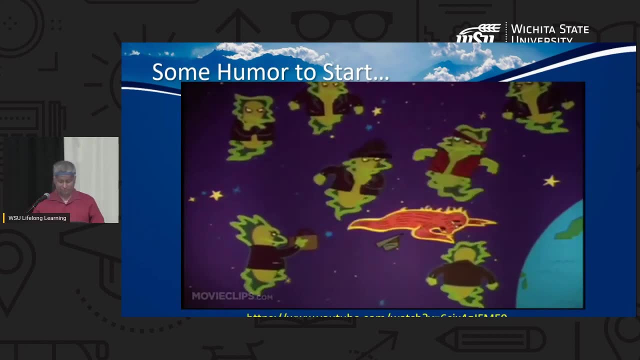 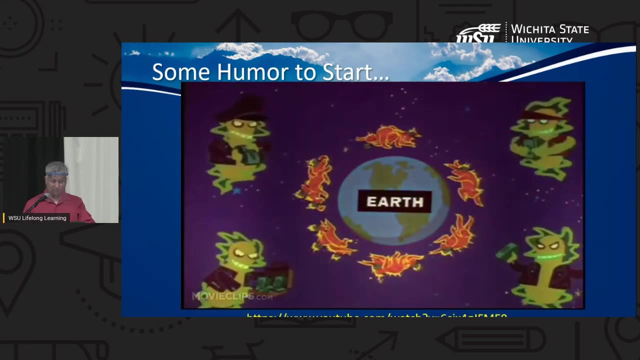 Not so fast. Sunbeam, We're greenhouse gases. You ain't going nowhere. Oh God, it hurts Pretty soon. Earth is chock full of Sunbeams. They're rotting. corpus Corpus is heating our atmosphere. How do we get rid of the greenhouse gases? 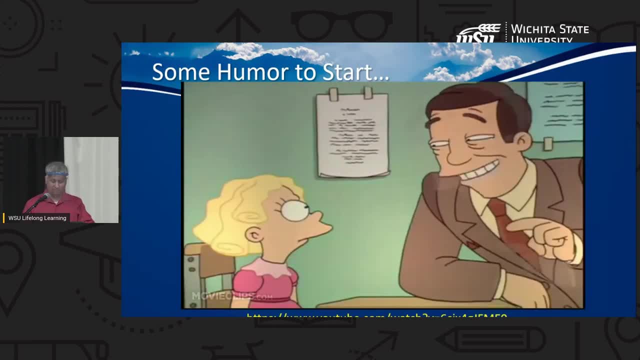 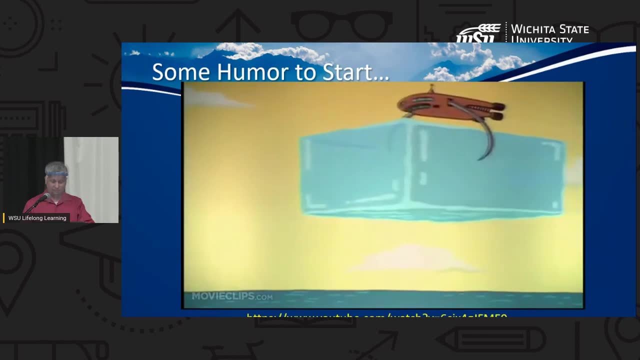 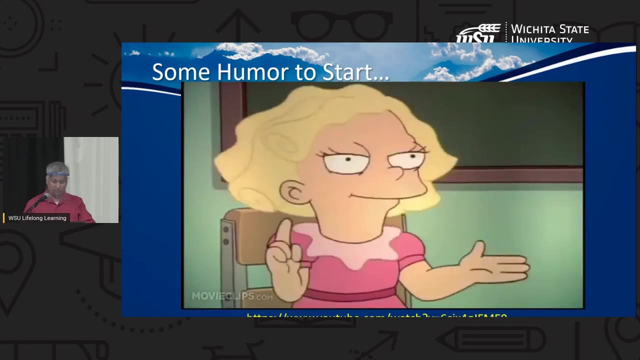 Fortunately, our handsomest politicians came up with a cheap, last-minute way to combat global warming. Ever since 2063, we simply drop a giant ice cube into the ocean every now and then, Just like Daddy puts in his drink every morning, And then he gets mad. 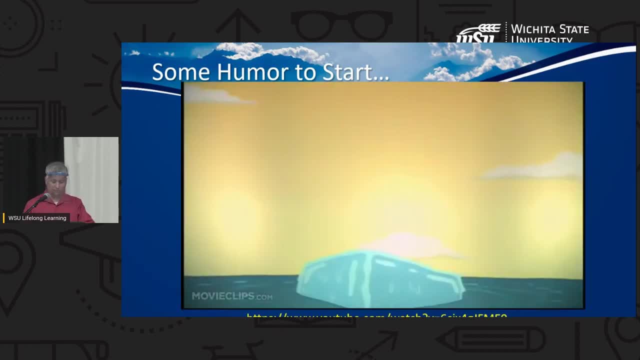 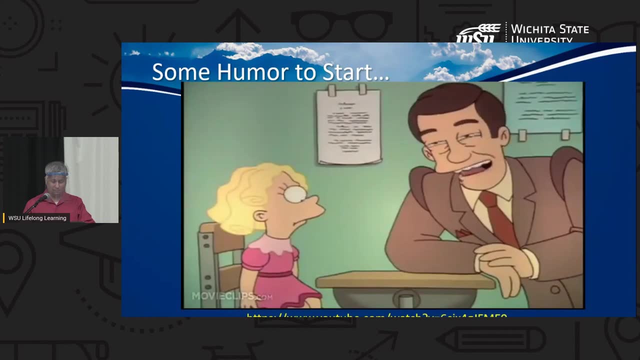 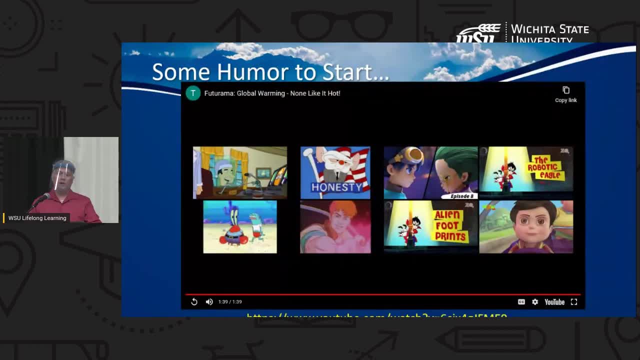 But what that video is illustrating is in basic terms. when we talk about greenhouse effect or global warming, we're talking about global warming. We're talking about the energy from the Sun entering into our atmosphere as it does, And the problem is it comes into the atmosphere, warms the Earth. 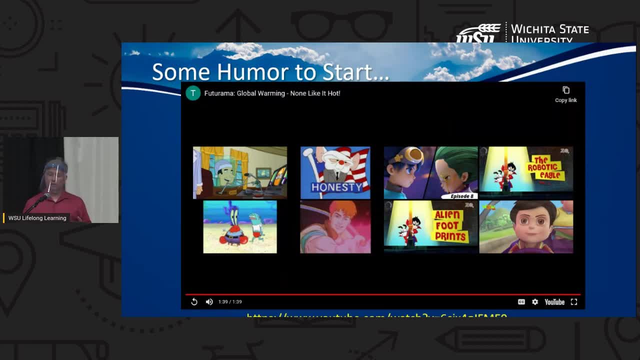 The Earth lets that energy go back into the atmosphere. But there are chemicals in the atmosphere, including carbon dioxide. That's the hot one that you hear about, Although, ironically, carbon dioxide for as much as that's in the conversation there's. 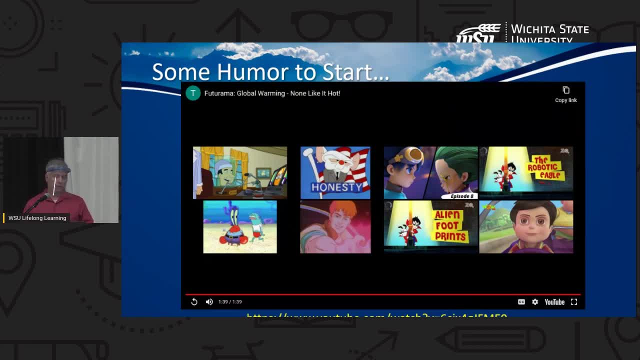 a lot of other chemicals that are far out there. It's really hard to tell. It's really hard to tell. It's really hard to tell far, far greater contributors to being greenhouse gases than CO2.. CO2 is actually one of the more. 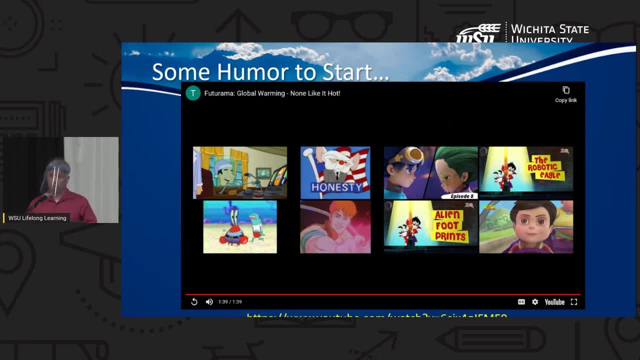 minor ones. Chlorofluorocarbons are very, very dangerous or considered to be very dangerous in terms of trapping in the Earth's energy, And we don't hear a whole lot about those these days because they've been basically banned. They were in a lot of your aerosol cans back in the 20th. 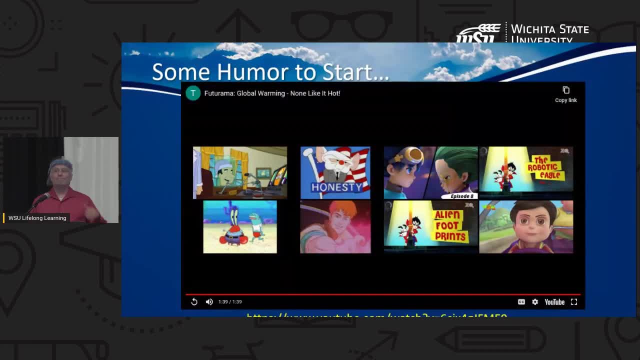 century, but we've since learned that that can cause problems in the upper atmosphere, And so those chemicals have been banned largely, And in recent years the chlorofluorocarbons in the upper atmosphere are now starting to trend downward. It'll take probably about another hundred. 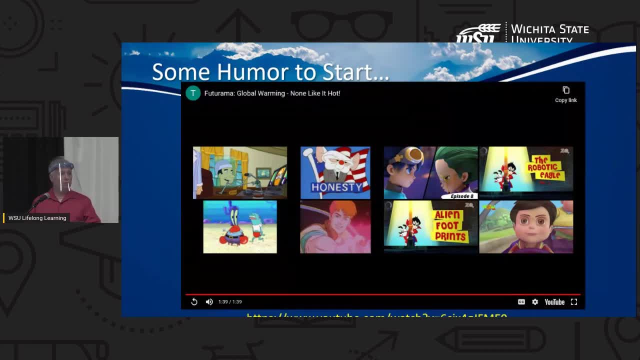 a hundred years for them to be banned, And so those chemicals have been banned largely. It's been 150 years of not having those in the atmosphere before it fully comes out of the atmosphere. But basically that's what we're talking about when we're talking about 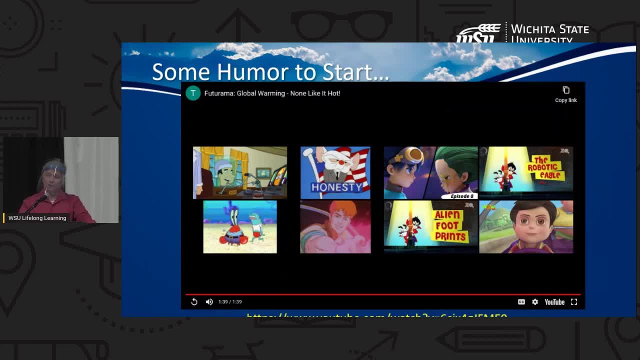 the greenhouse effect, the idea of going into a greenhouse where the sunlight and the radiation from the sun comes in and gets trapped and isn't as easily able to get out as it comes in, And really at the core of when we're talking about climate change and issues along those lines. this is where a lot of that concept is starting. 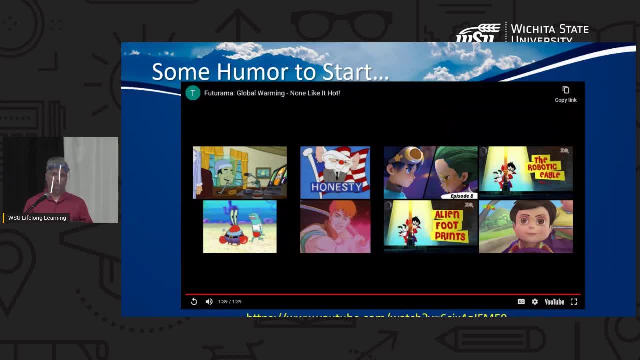 from, But in terms of how it affects the atmosphere and how it will affect the atmosphere, well, that's where it gets a lot more murky, as we encountered in earlier subjects in this class. So let's look at the two sides of this story on climate change. 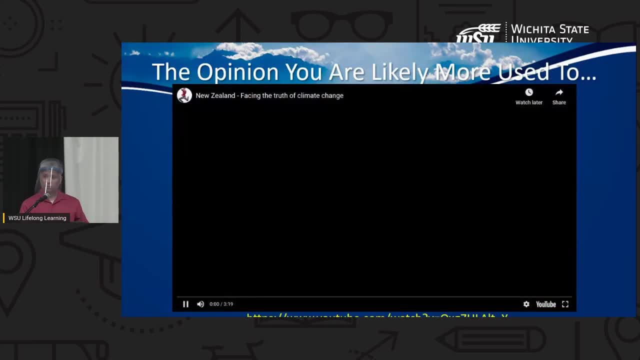 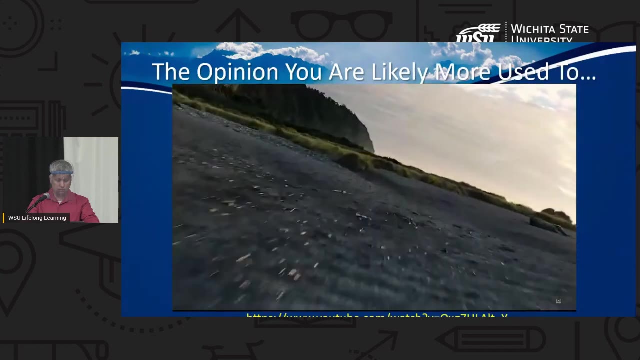 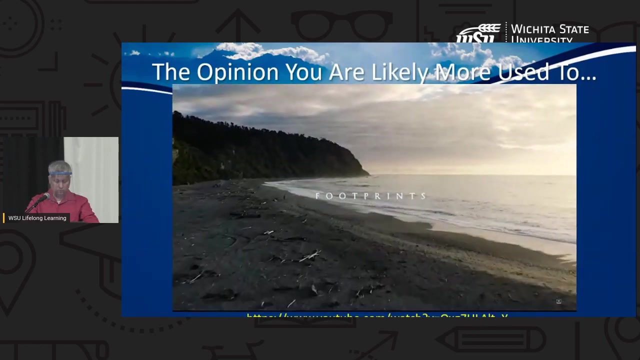 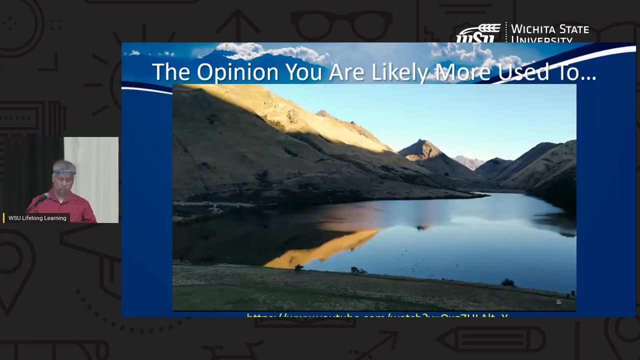 This is probably more of the opinion that you're used to watching the media and things like that. It's actually a really well-produced video. Higher temperatures are already rising in the United States and we're seeing a lot more of them. The temperatures are already happening. They will increase deaths, Food and waterborne. 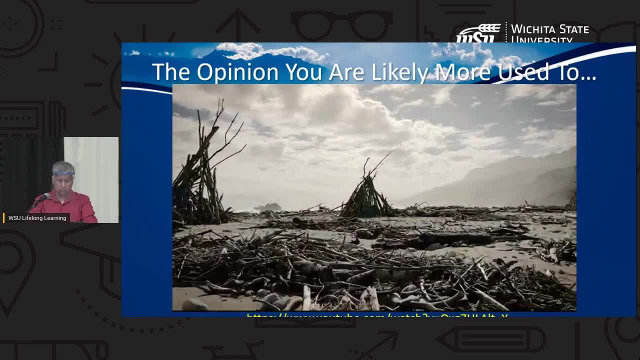 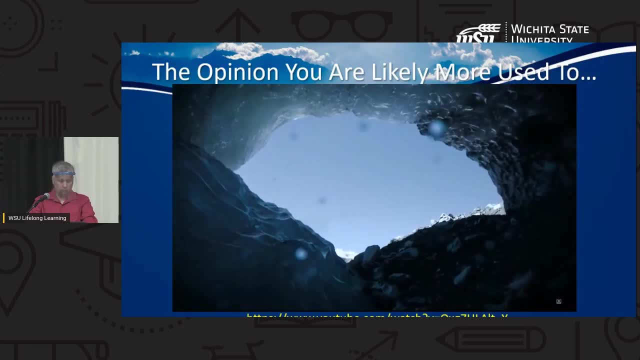 illnesses will spread. Wildfires, as we've just seen, will increase. Floods, as we've just seen after hurricanes, will be more frequent. Asthma and allergies will be worse. Crop production will decline because of high temperatures and drought. 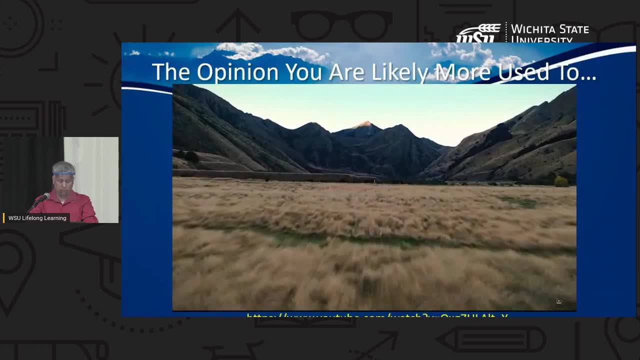 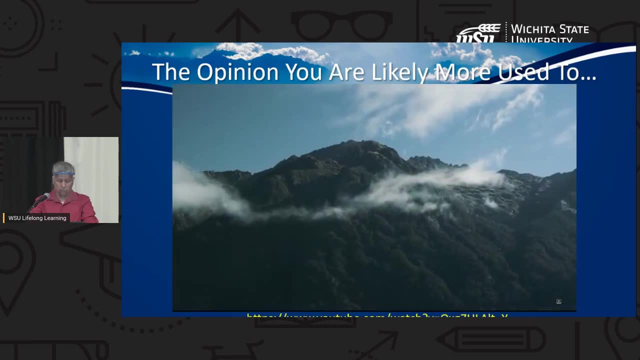 I've got an experiment for you: Safety glasses on. By the end of this century, if emissions keep rising, the average temperature on Earth could go up another 4 to 8 degrees, And that's a lot of degrees. What I'm saying is the planet's on fire. 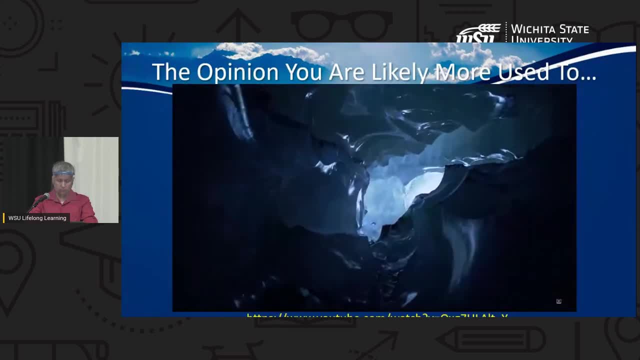 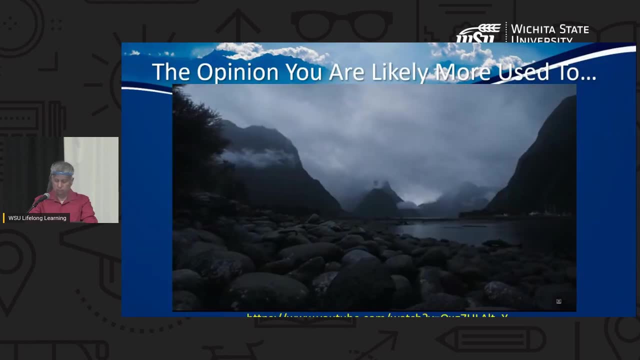 A new panel says governments around the world must take rapid action to curb rising temperatures. We're also seeing rising sea levels due to accelerating melting of polar ice. NASA recently found a glacier on Antarctica's western coast has contributed to about 4% of the world's. 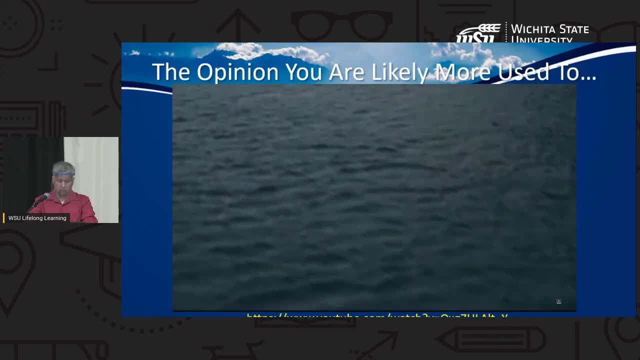 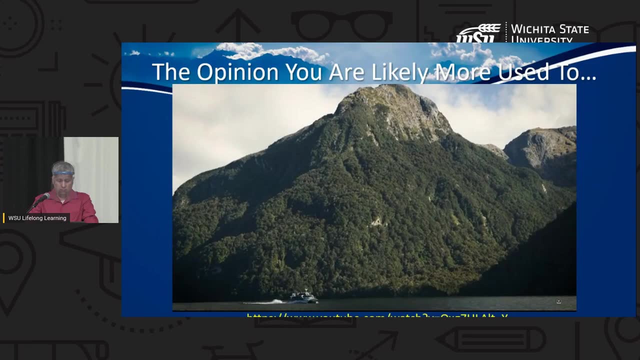 rising sea levels. It makes me feel frustrated because again you can say: I don't believe in gravity, but if you step off the cliff you're going down. So we can say: I don't believe climate is changing, but it's based on science. that's over 150. 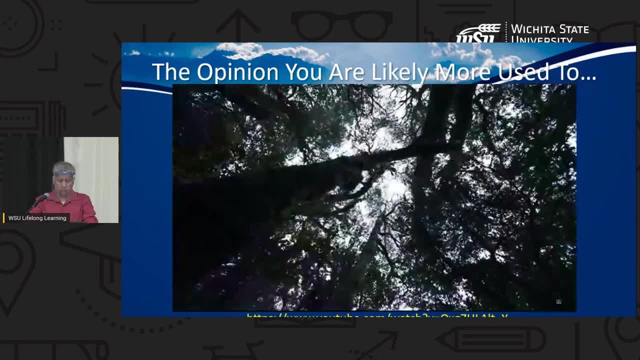 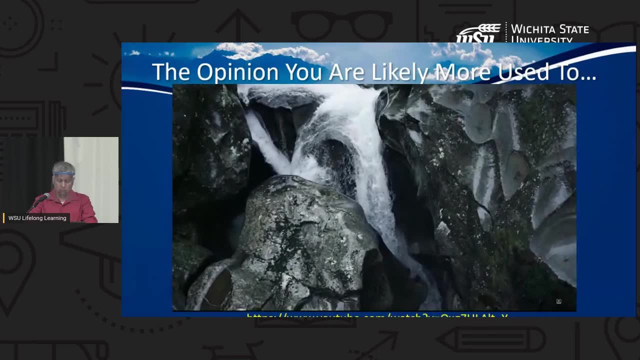 years old, And if we're making decisions that don't just affect us, but that affect hundreds of millions of people, based on flawed or faulty information, the result is not going to be good. Just this Saturday, sensors in Hawaii recorded new carbon dioxide levels, And you know how. 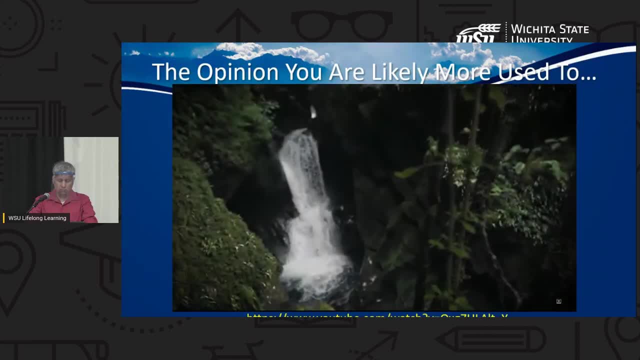 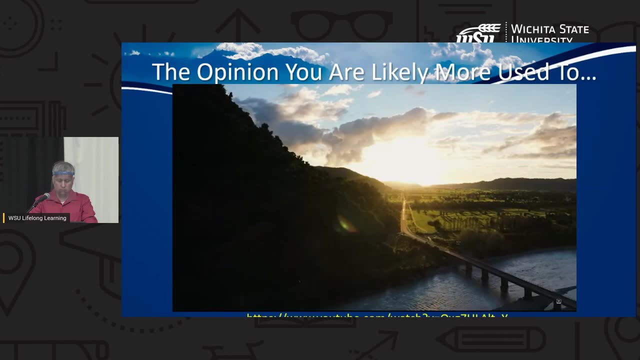 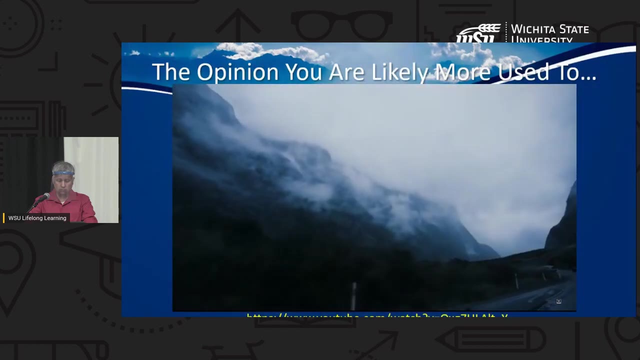 long it's been since it has been this bad- Three million years. We're already seeing the consequences of this new era of climate change. First, there's rising temperatures. A recent NOAA report found that 2018 was the fourth year of this year ever recorded on planet Earth. 2016 was the fourth year of this year. 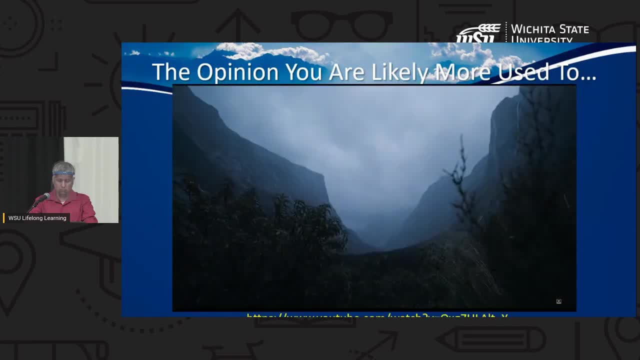 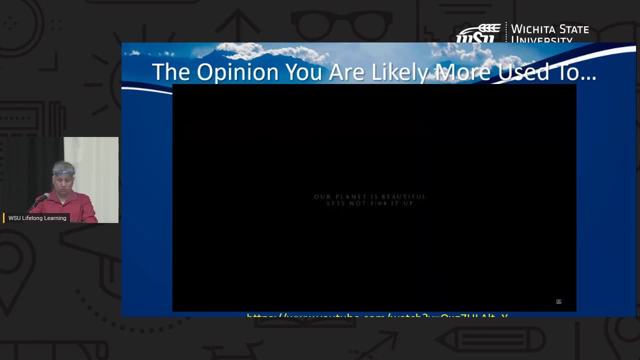 ever recorded on planet Earth. No, of course not. Nothing's for you idiots. We're also seeing rising sea levels due to accelerating melting of polar ice. NASA recently found a glacier on Antarctica's western coast. has contributed to about 4% of the world's. 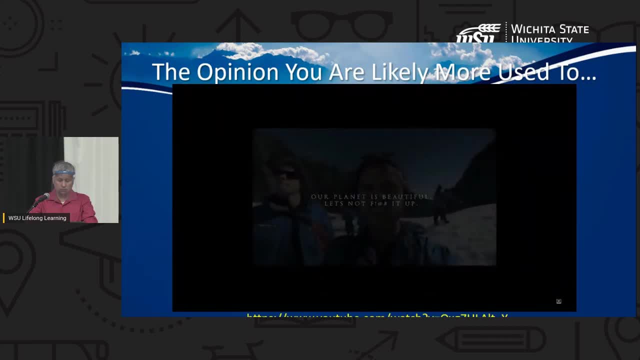 rising sea levels. This is an actual crisis. The one thing that's like super sad that our tour guide was kind of saying is that, like within 20 years from now, Within 20 years from now, due to climate change, we won't be able to climb this Like there. 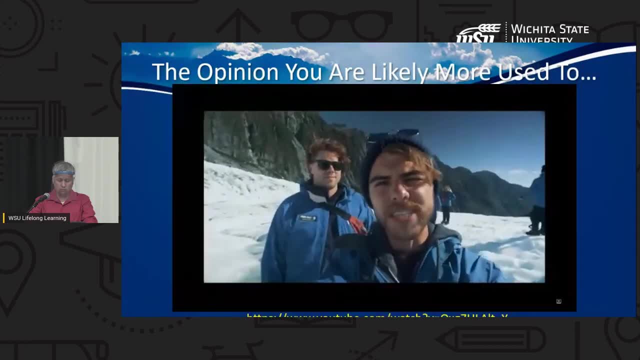 will be no way to come up here because it'll be way too unstable. And then within the last- I think it's like within 60 years- like most of this will be gone. Yeah, A hundred years, it'll be completely gone. 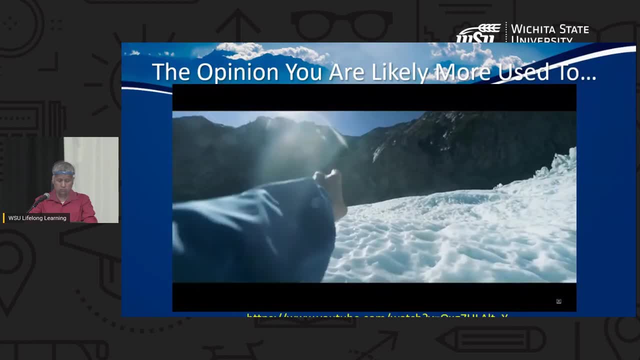 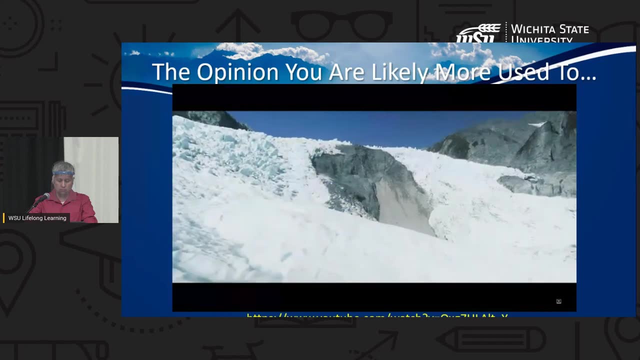 So there used to be snow all along this area, And then this used to be filled with it as well, And then over time, just I don't know. It's a bit of a sad reality that we sort of have to be a little bit more. 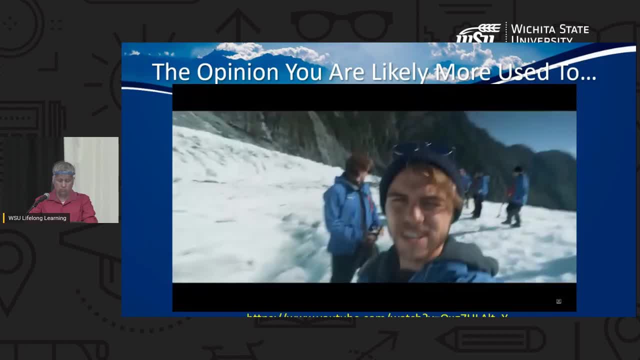 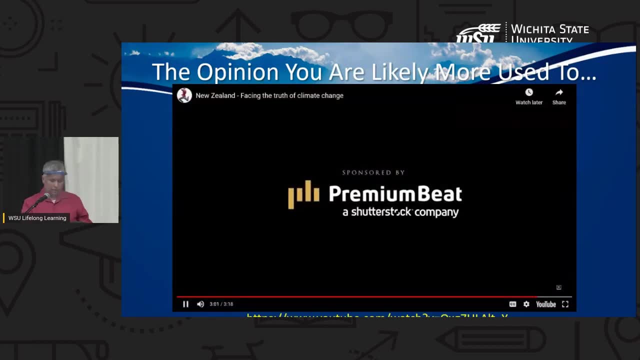 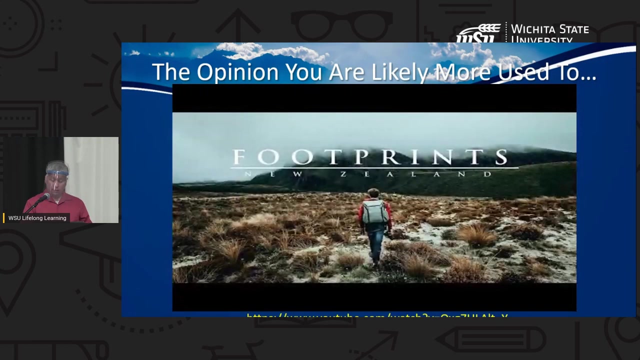 conscious of the footprint that we make, Not only within the snow, but as we travel and what we do. Okay, So that's kind of the more common viewpoint that you're going to see, especially in much of the media, But that's not the only side of the story, necessarily. 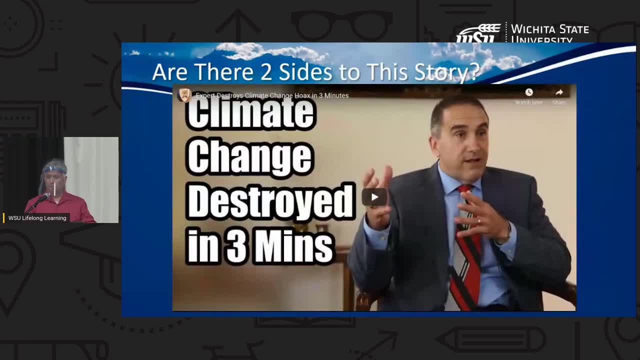 I know, actually, within the professional meteorology as well as climate change, you would think that everybody is all in one camp, except for maybe one or two people. I can tell you from at least my experience in this industry, that's not the case Now, are they? 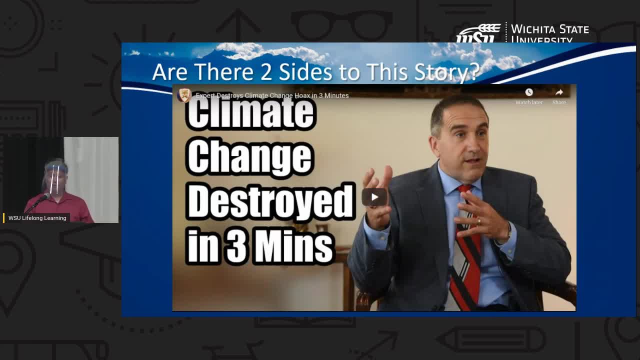 all to one side or all to the other side? No, It's a very mixed bag because, like you may have picked up earlier on in this class, there's a lot that we don't actually know about what's going on in the atmosphere, And we are learning more and more every day, especially as computing. 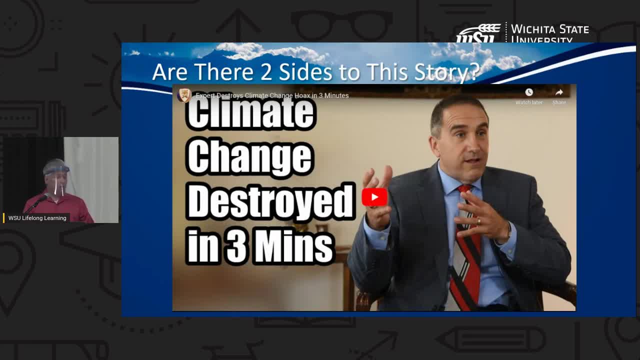 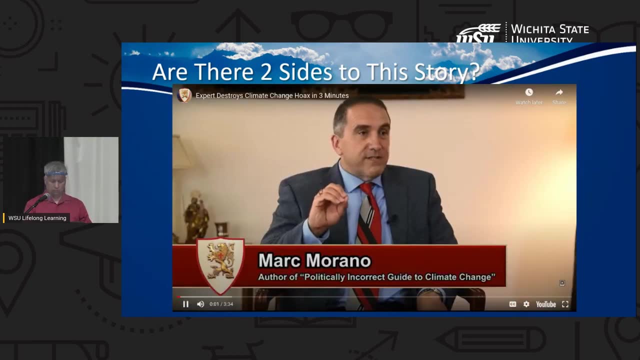 power gets better and better, So let's listen. This is another three-minute video, kind of on the other side of the story here. Medieval warm period was from 900 to about 1300 AD, And yet the Roman warming period around the 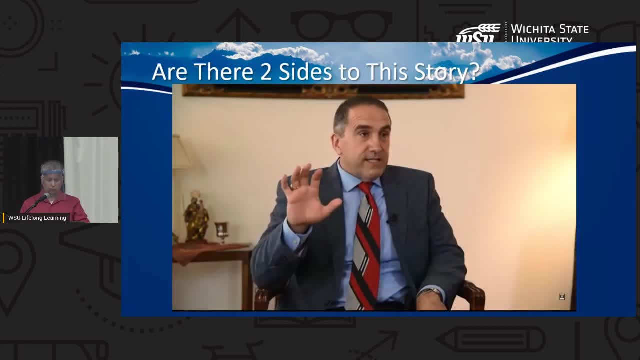 0 AD. Peer-reviewed studies, geologic records and all the studies have shown that we have actually cooled since the Roman warming period and likely since the medieval warming period to current. In other words, we were up here warming the Roman warming period, then we cooled a little bit. 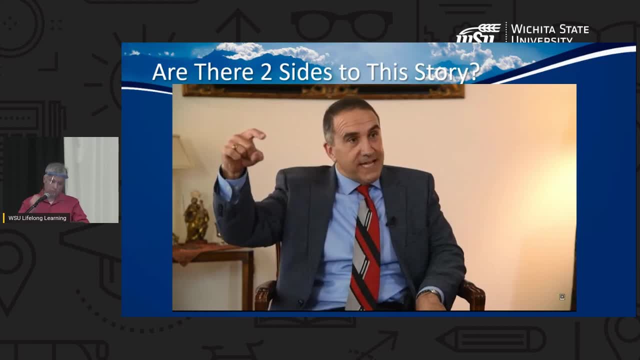 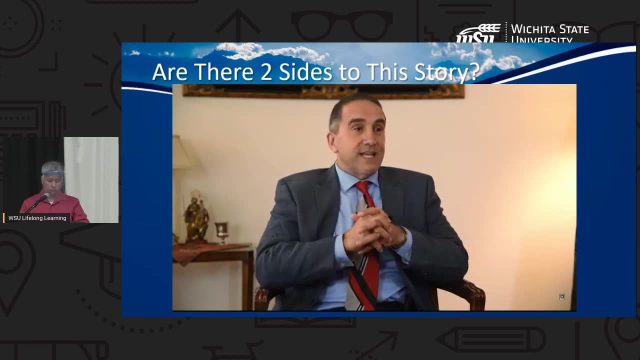 then we warmed in the medieval warm period, then we went to a little ice age and now we're back up, Not quite where we were in the medieval warm period. The first United Nations climate report- 1990, showed a massive medieval warm period in the 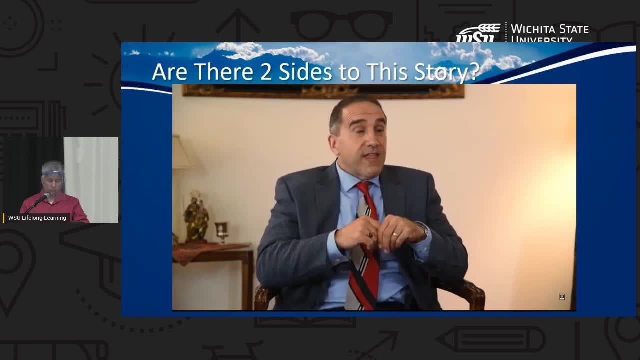 medieval warm period and then it goes down and we still weren't at that same temperature. That was untenable. So what happened? We actually had the scientists testify in the United States Senate. He got a call from a colleague who said we have to get rid of the medieval warm period. 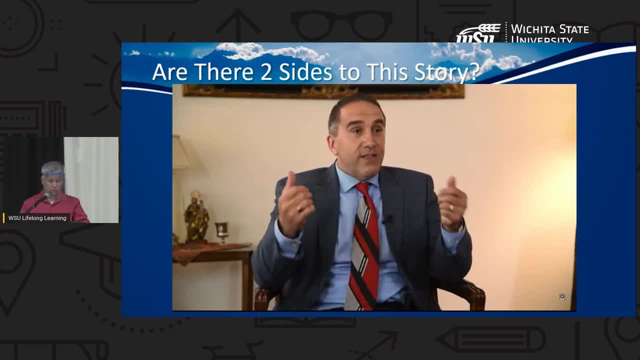 These were UN-affiliated academic scientists. Guess what? By year 2000,. they got rid of the medieval warm period, They erased it. They went back and they said: you know, we've looked at everything and it no longer existed. They showed a flat line. and then the 20th century: a big hockey stick. 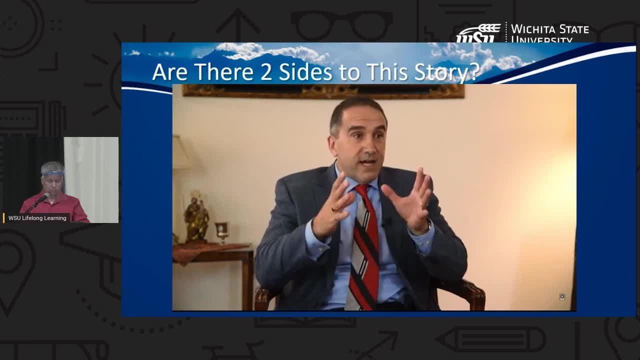 That's what they did. And then I have a whole chapter devoted into my book on the con. that was erasing the past, But they've done it before. Skeptics, climate skeptics- made hay out of the eight, almost 20-year pause in global warming. What does the federal government do? NOAA scientists Tired of this. 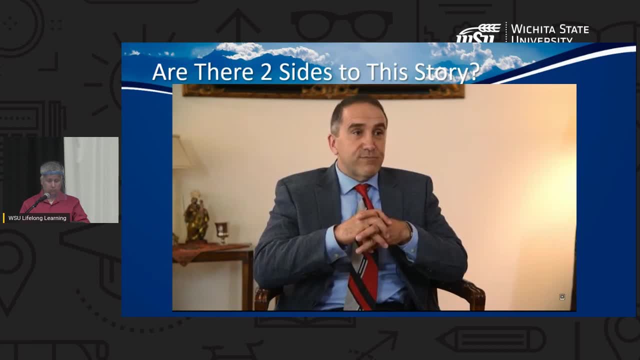 They're sick of it. They have satellite data land. The temperature's not going up. They're frustrated, They're angry. It's ruining Right before the UN-Paris agreement in November 2006-15, in 2015,. NOAA. 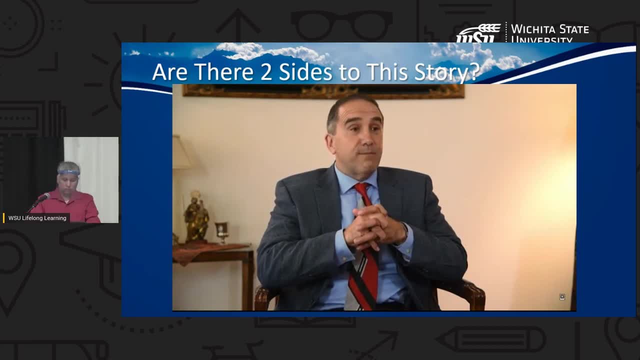 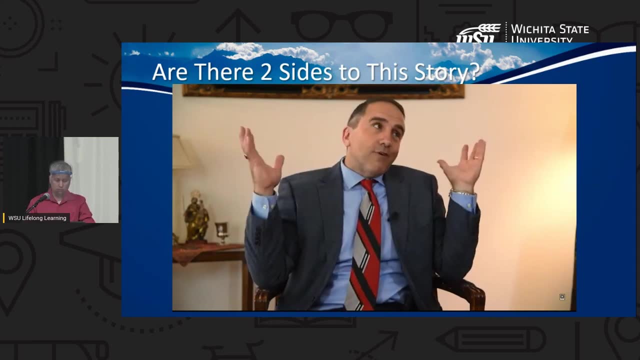 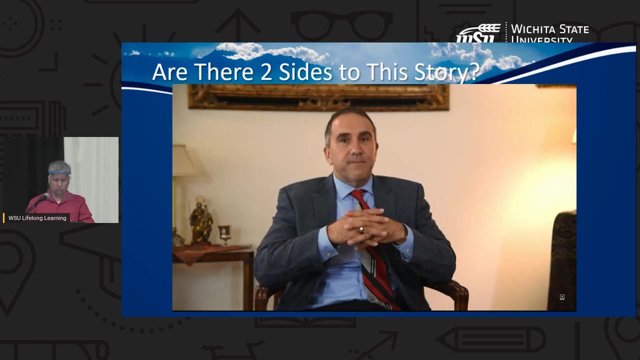 a federal agency scientist comes out. They called it the pause buster study. They said: you know what? We've redone the numbers. We've looked at the past, We did it wrong. And here's the new data: There was no global warming pause. My favorite quote to sum this up the whole climate debate is: 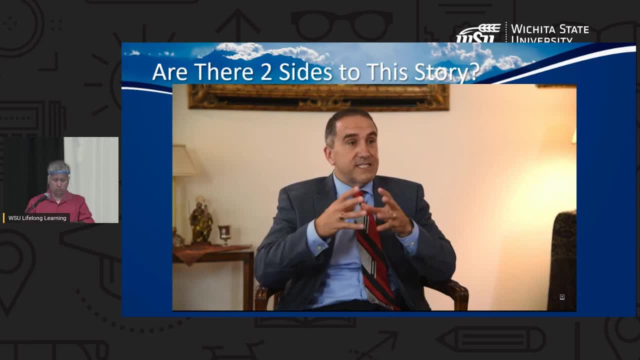 there are literally hundreds of factors that influence the climate. Carbon dioxide is not the control knob, The idea that humans can tweak one variable among hundreds of factors, from tilt of the Earth's axis, to water vapor, to methane, to clouds, to volcanoes, to ocean cycles, et cetera- One selected factor, the human contribution. 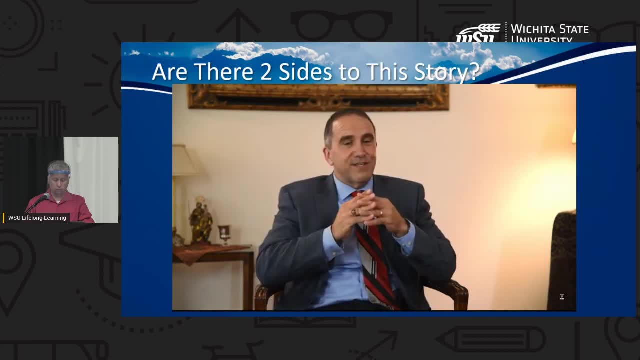 to CO2, which is microscopic of the whole CO2,, natural CO2, and think we can come out and control the climate with that. The scientists called it scientific nonsense. And that's the bottom line. If we face the climate catastrophe, you would not want to centrally plan, You would not want to empower the United Nations. 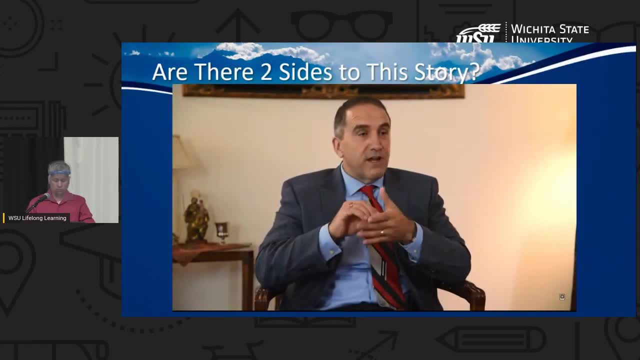 You would not want to stifle technology. You would not want government picking winners and losers in energy technology. You would want to unleash the free market system, The day someone could walk into Walmart and buy- you know- alternative energy. if you can go in and buy a wind- not a windmill but a solar panel- put it on your roof. 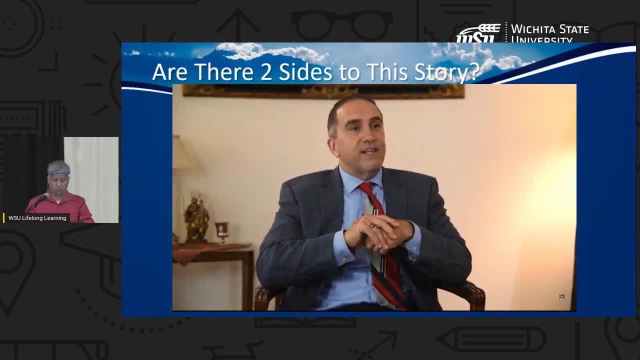 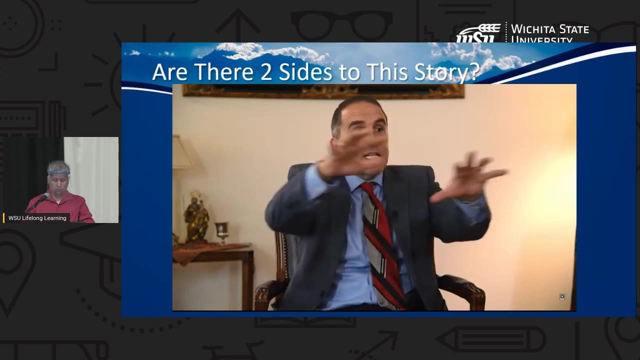 get off the grid. that's the day you don't have to worry about any fossil fuel debate or anything going on. But you'd want people to be wealthier, more prosperous, technological advancements, And none of that is what they're proposing. The Green New Deal is all about masterminding everything. 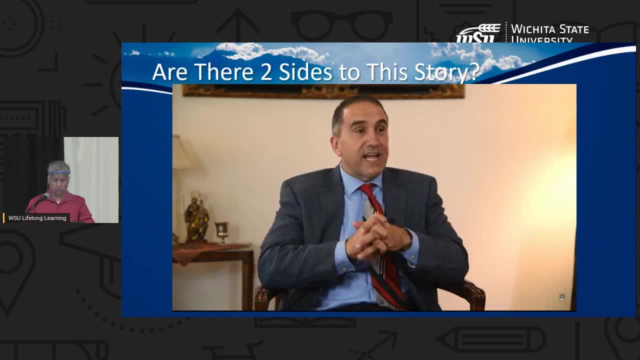 and central planning. And that's what's frightening is that if we actually faced it, their solutions would be the exact wrong way to go. Thank God we don't face it, But if we did, not only would they have no impact on the climate. 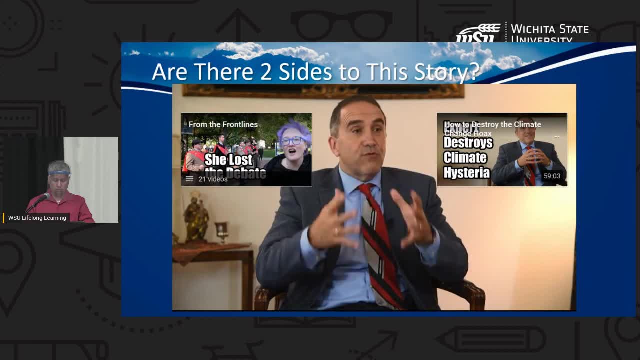 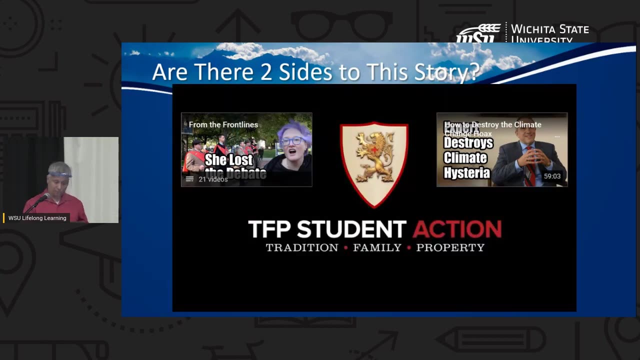 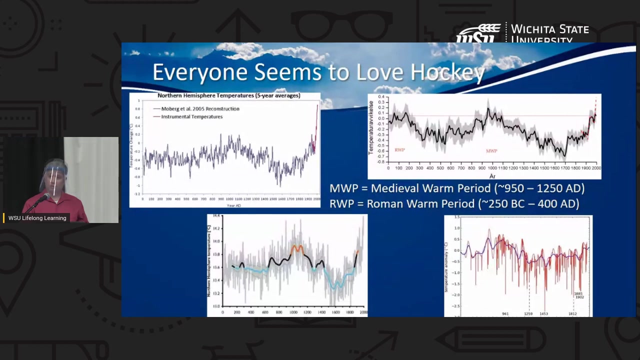 but it would take us down a completely dark, anti-human road of crushing development, seniors, poor people, fixed income, paying much more percentage of their income for energy to do absolutely nothing for the climate. So we have two pretty big extremes there. Any thoughts? questions right now. 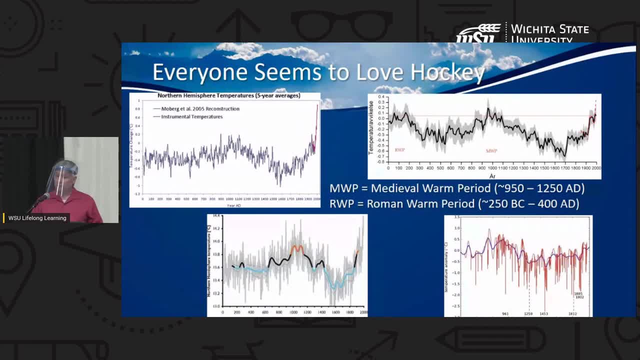 OK, if anything comes up, feel free to jump into this discussion. One of the things that came up in that last video in particular was this discussion of the hockey stick diagram. Who here has heard of that before? or you've watched TV anything on climate change, global warming? 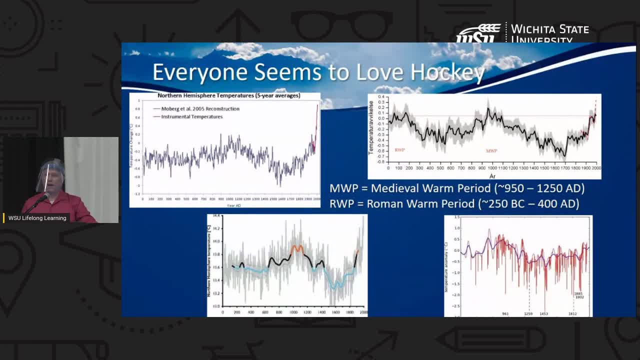 you've probably heard a little bit about it, The idea of the hockey stick diagram, and really it's this one right here that truly kind of fits. that is the idea that things were really fairly flat through much of the modern era since. well, on here it goes from 0 AD to present day. 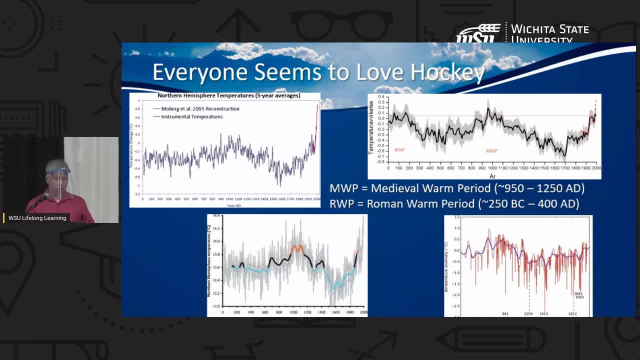 So you've got 2,000 years on here and, yeah, it went up and down a little bit and then it just massively spiked right at the end. And so, oh my gosh, what's going on here? right at the end. 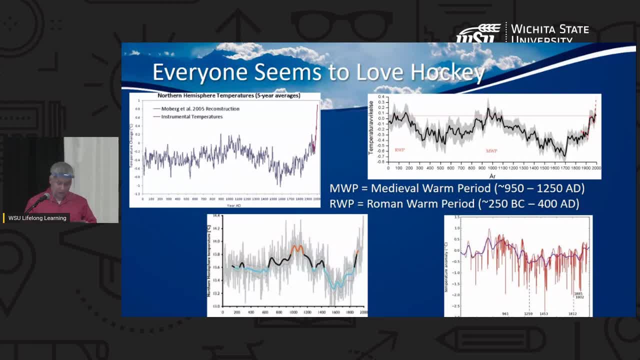 But each of these four diagrams- and I know, especially on your little printed printed slides it's not as easy to see- but all four of these images are the same data, plotted, the same information, and yet they all look very, very drastically different and tell different tales. 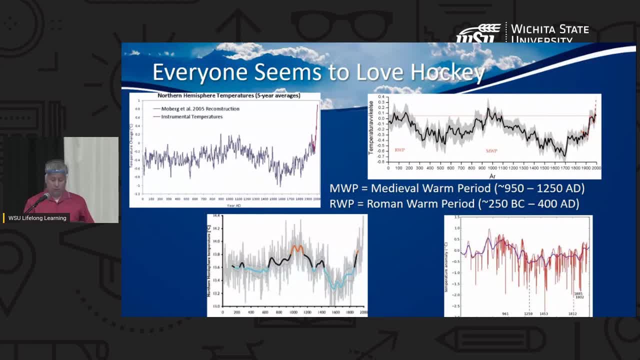 Oh yeah, and not on your slides, but what I put on here, just for clarification, that on here: MWP, MWP, RWP. that was brought up in that second video as well. the medieval warm period and the Roman warm period. 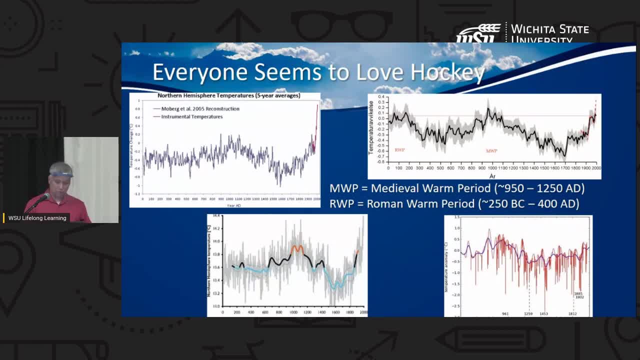 Notice how those are reflected on this one versus this one and here and there. I mean you've got four diagrams that are all trying to show the same data and trying to take make assumptions on that data. I mean you've got four diagrams that are all trying to show the same data. 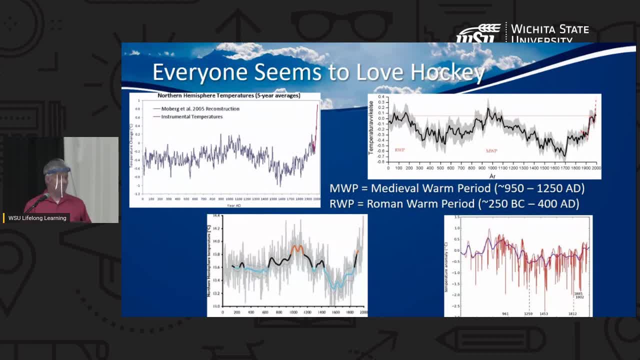 and coming up with four very different results. Because here we should be panicking right now. Oh my God, Temperature going through the roof, Although in spite of this big spike, it's really, relatively speaking, in terms of overall temperature, still a fairly small spike. 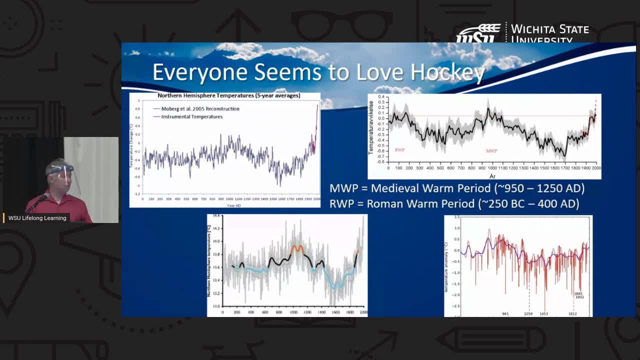 but it is a rapid change in a short period of time. and when we are scientists observing things, we see anomalies, and those are what we focus in on, because that's what we do as scientists. But if you come over here, another study, another peer-reviewed and journal-published study. 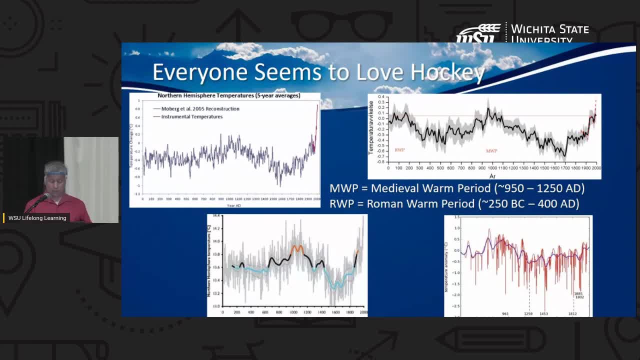 shows this Roman warm period around. really, it started a little bit before 0 AD and continued, they say, roughly to about 400 AD, where it was warmer, and then in the Middle Ages, about 1500 years later. 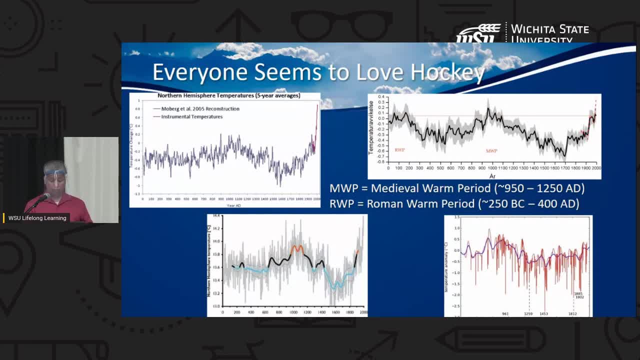 it got warm again. and then we're another thousand years later, it's getting warm again. You look at that. then you're like, well, I don't know, maybe we're just in a normal cycle right now, And then you've got over here another one that doesn't so much elevate the Roman warm period. 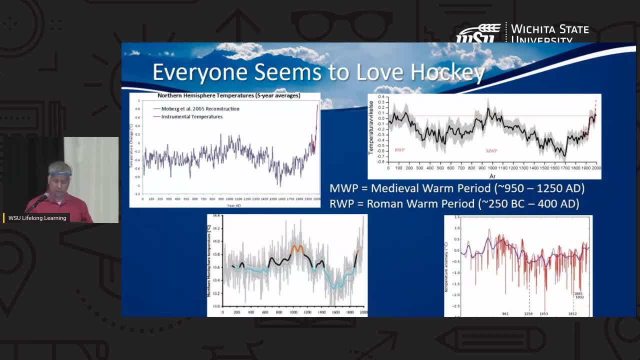 but definitely shows a huge spike in the medieval warm period. I think this is more along the lines of the diagram of the research that that second guy was referring to in his video, that we're still kind of climbing out of the Little Ice Age. 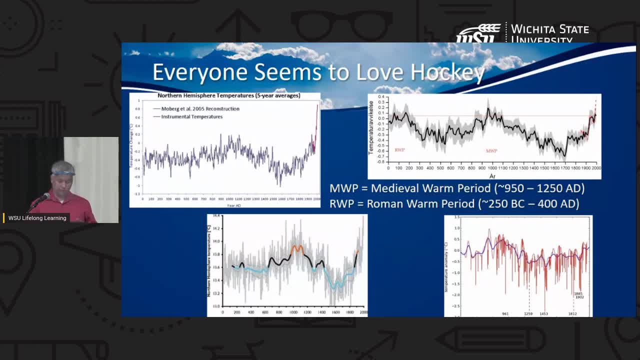 which was in and around about 1500 to 1700 AD. So what I'm getting at in all of this- and it's something that I try to tell my full semester meteorology classes too- is in academia we should never squash scholastic thought and debate and research. 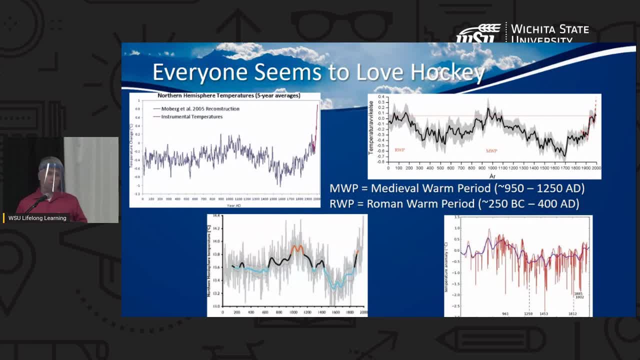 One of the things I mean, if I'm going to step up on my soapbox- which I will do a couple of times today- and say, if you've got, and this is what I've found in life, this is what I find in science. 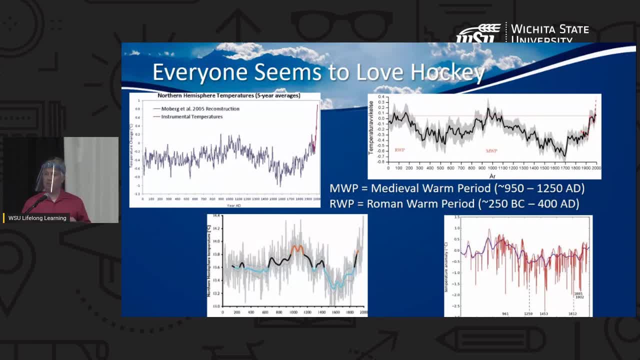 if you have a bunch of people stepping up on a box and saying something is settled, that's something you should be afraid of. We have settled science in so many areas over the course of human history that have turned on their heads. 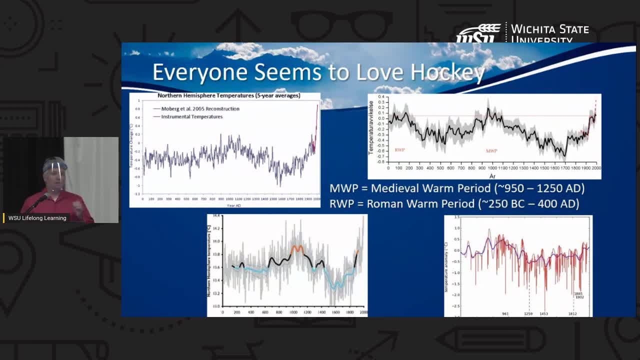 and been proven wrong later. Finding an outcome should always be challenged, No matter how many people come to the same conclusion. never stop asking questions. That's why, in a lot of respects, you're all here. You want to learn more. 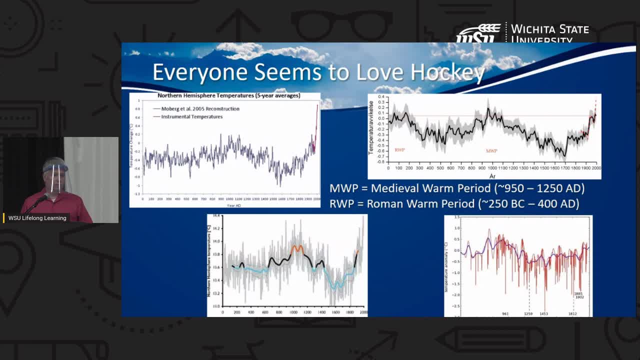 You want to understand more And I can't tell you right now if this is right. I can't tell you if this is right. These are different conclusions and we're going to get into this a little bit as we go forward in this class period. 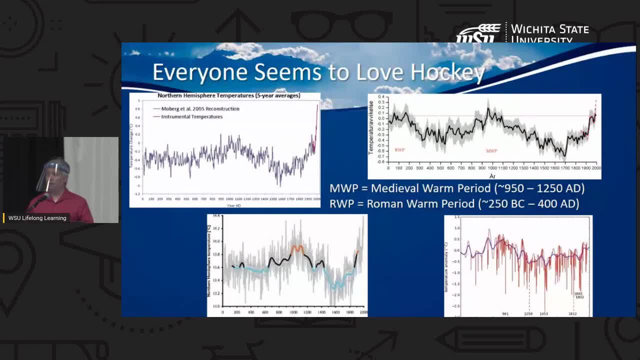 These are different conclusions that different scientists have come up with based upon the data that they have gathered and the assumptions they have made based upon that data. Remember- and I'm stealing a little bit of my thunder for later on- how short the period of history we have of actual hard numbers. 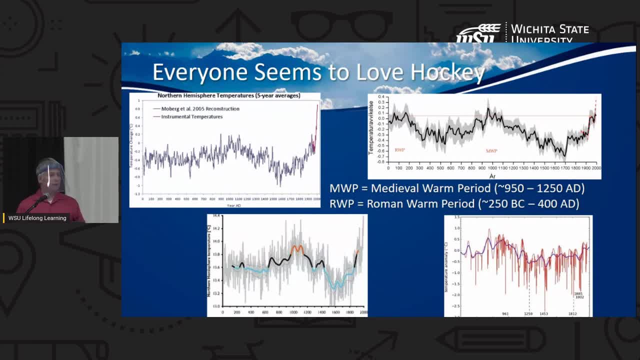 actual, real data that we can take reliably across the entire planet at a specific time. If we go back and look at just our remote sensing from our satellites, that goes back 50 years And even over that course of 50 years. the most accurate data across the planet is really in about the last 20 years. 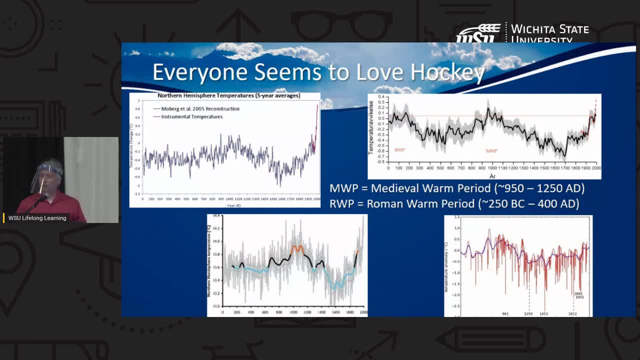 in this century, When we go further than about 150 years into the past, we have to start making a lot of assumptions, And some of those assumptions are very good assumptions, but they are still assumptions and they are still limited data. This is where it's important to think in terms of accuracy and precision. 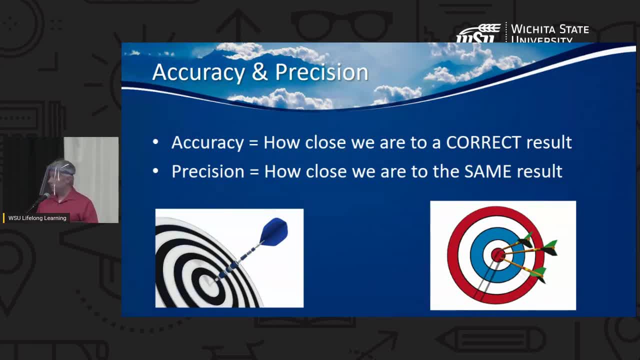 when we're looking at these things. Accuracy is how close we are to the actual right answer, And then precision is how close are we to the same result. Now, accuracy is pretty hard for us to determine when we actually don't have an instrumentation device. 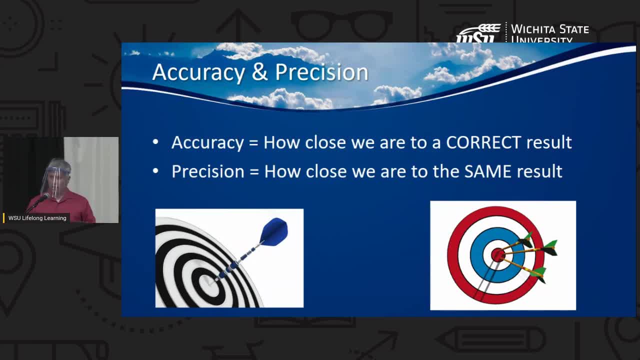 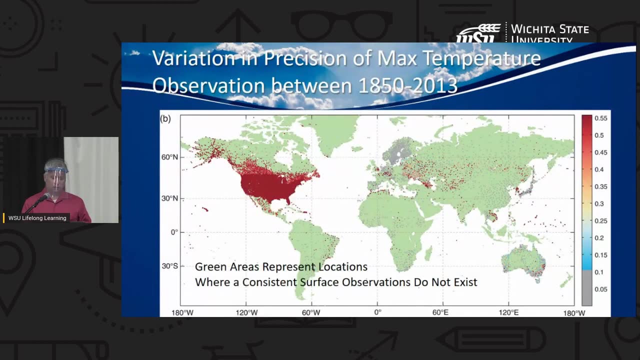 available to us a thousand years ago, And so we have to make some assumptions. Precision again talks about how close we are to the same result, And when we look on this next slide, precision is very hard to come up with. when this is looking at. 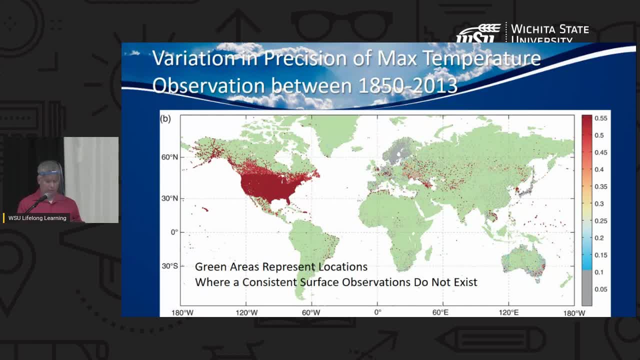 and this is kind of a confusing way that they've displayed it on here. but what they are getting at in this image is what we are seeing is where our consistent temperature observations are available and being tracked consistently, versus where they are not being tracked consistently. 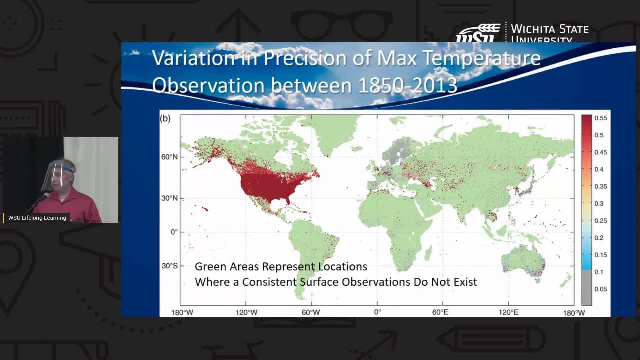 This goes from 1850 to 2013.. So this is covering up until seven years ago over that period of time. So even today, look at all of these areas of green- There are no instruments at those locations. There is nothing tracking the weather. 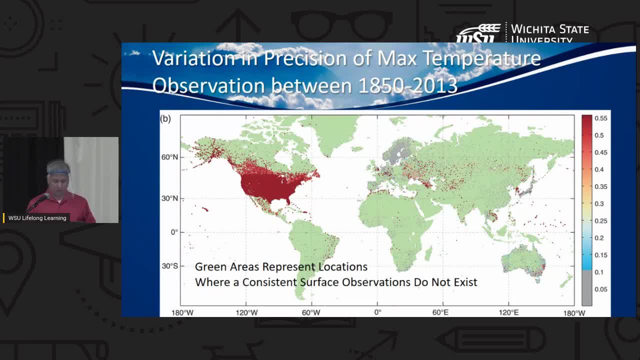 Greenland. here you've got just a few surface observations. consistently You've got a better network across a little bit better of a network, although a younger network- across Asia and Russia. But there's a lot of green on here, That green. 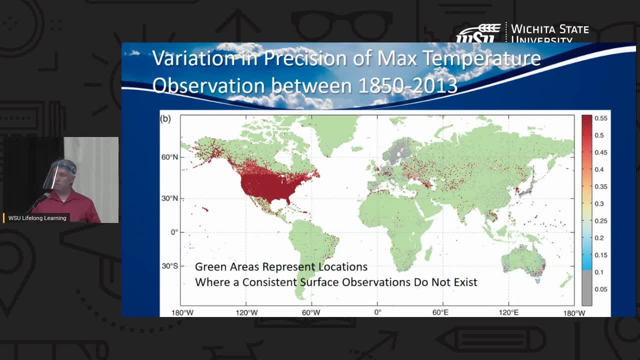 those are places that we're not actually taking consistent surface observations with modern technology. And that's actually a pretty amazing thing, even for me, looking at a graphic like this, because we think how advanced we are and how much we know and how much we're learning. 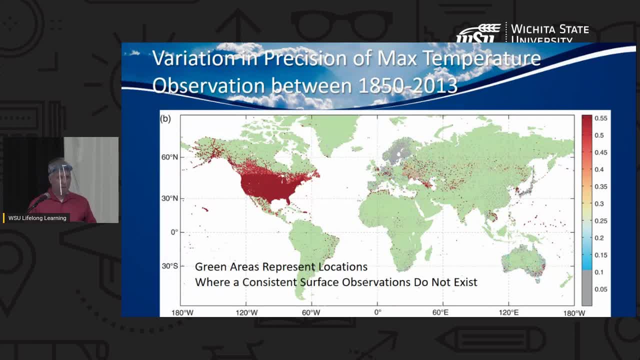 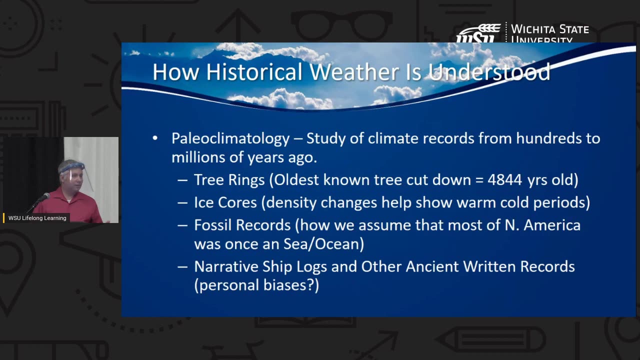 And all of those things are very true. But all this green tells us there's a lot we don't know. So let's go into. how in the world do we figure out what the climate was before we had instrumentation, before we had ways to actually measure that? 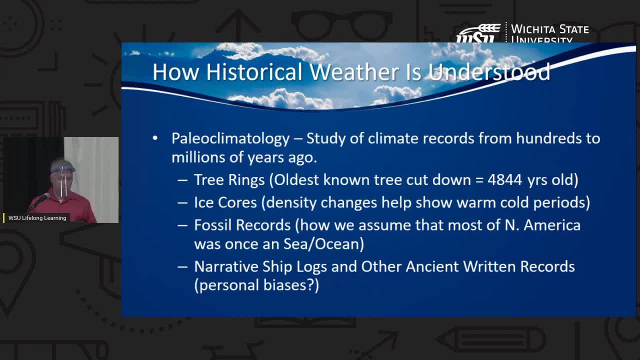 you know, we actually measure that it is 92 degrees outside right now, or whatever it is. Well, we had to infer that information And we do that in part through what's called paleoclimatology, which is really we're grabbing things that can help us ascertain. 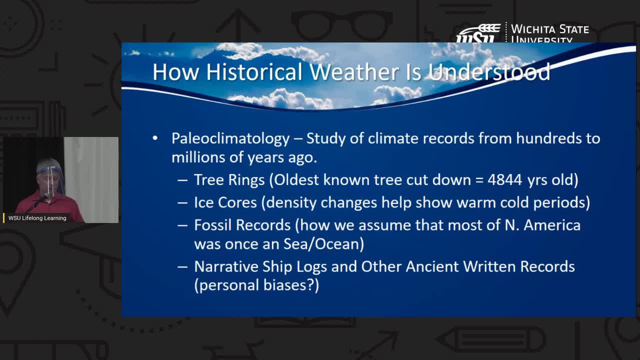 how the weather was like in a previous time, in which we don't actually have physical measurements available. Some of the records that we can get come from tree rings. Those are great, except for the fact that trees die and they disintegrate, everything like that. 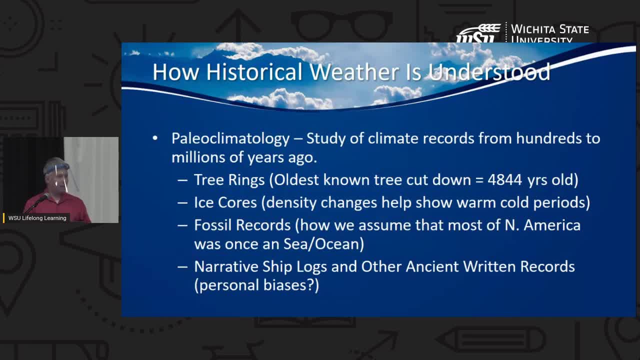 And so really our tree rings can only go back about 4,800 years. We've got ice cores. They do last longer, especially in polar regions, But again, ice cores aren't really useful observation points near the equatorial regions, So we can get good pictures near the poles. 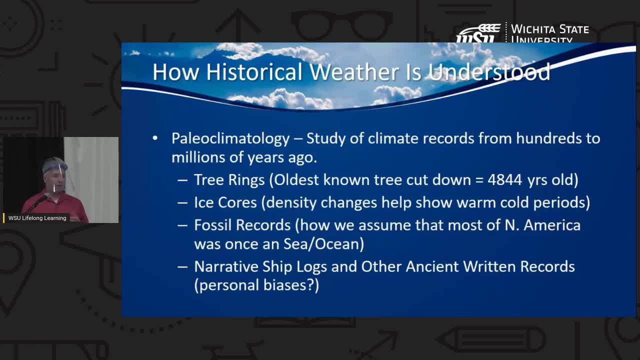 when we're drawing out an ice core, but it doesn't tell us exact temperatures and it doesn't give us our mid-latitudes and it doesn't give us our equatorial regions in terms of how the climate has evolved with time. Now, an ice core, 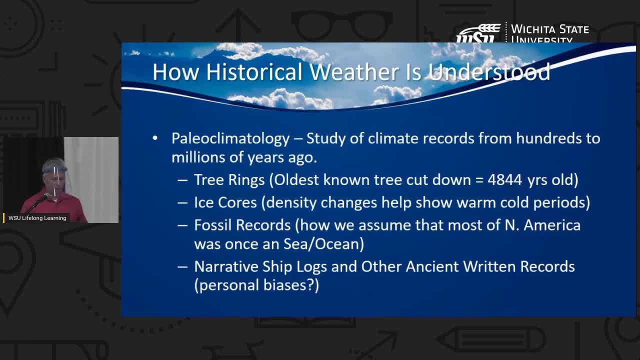 and I wish I had a picture of it. I didn't put one in here. Basically, what happens is they just take this ginormous drill and go into the ice in the polar regions and they pull out literally kind of a cylinder of ice. 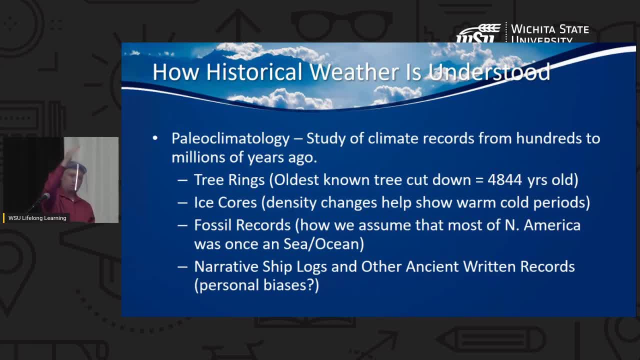 And they just they pull it out in chunks of X number of meters and based upon the density of the ice, how it's melted and refrozen, they can determine in a general sense warmer periods versus cooler periods at that location. Now it gets even crazier than that. 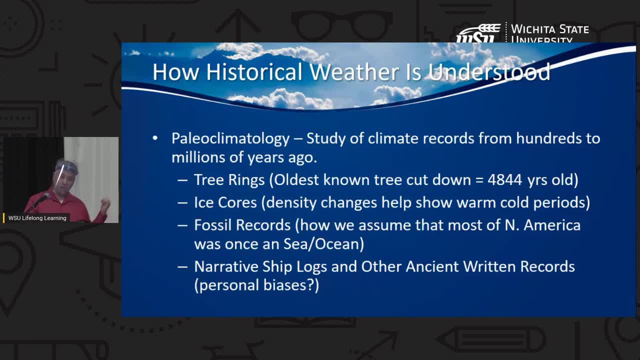 because then they also have to make some assumptions if they go real far back as to the movement of land masses, But that's, we won't even go there, because that even gets more crazy with the fossil record, Which can go back tens of thousands. 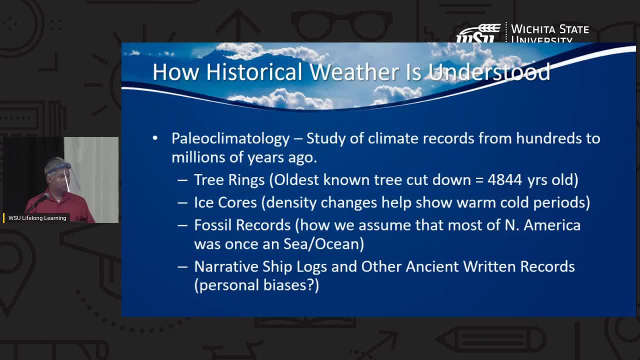 if not hundreds of thousands of years. So we look at the fossil records to assume- well, for example, this is how we know- that most of North America was at one point a sea or an ocean. If you go back far enough, we would be underwater here in Wichita, Kansas. 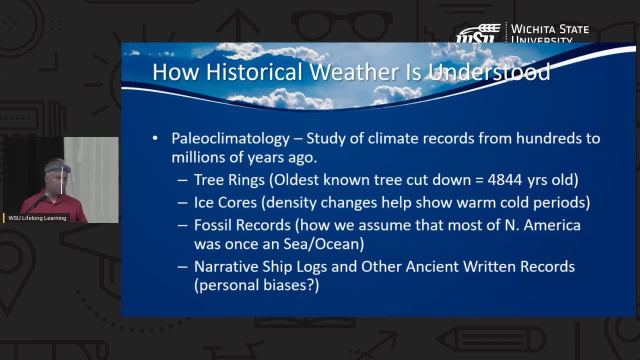 There was a great oceanic body that pretty much went through the center part of the United States at one point, or the mass that would be the United States, And then- and we know this backing up, we know this because we've collected- 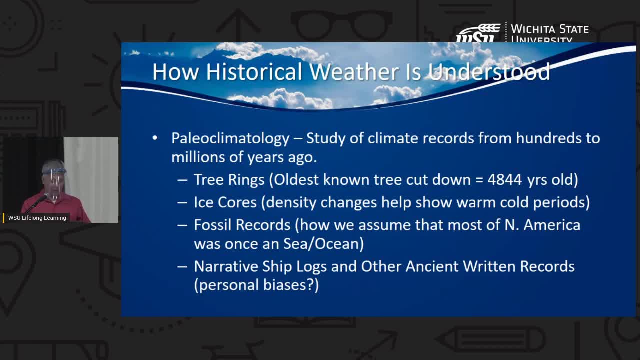 oceanic fossils across the central plains, And so that's how we know that there was more water available to us at one point. And then, lastly, in this area this is certainly not totally comprehensive, but we also look at what is available. 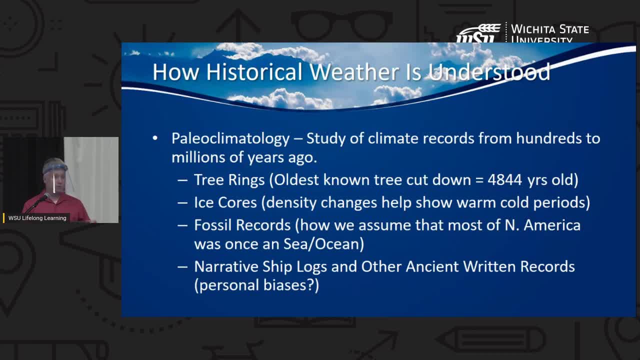 in terms of ship logs, which are generally some of the better kept logs available to us in terms of shipping goods, and your ship captains, even back hundreds of years, kept very thorough logs on how the weather was, what the conditions were as they were sailing. 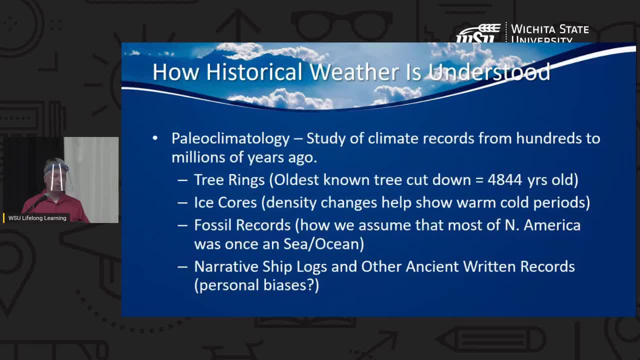 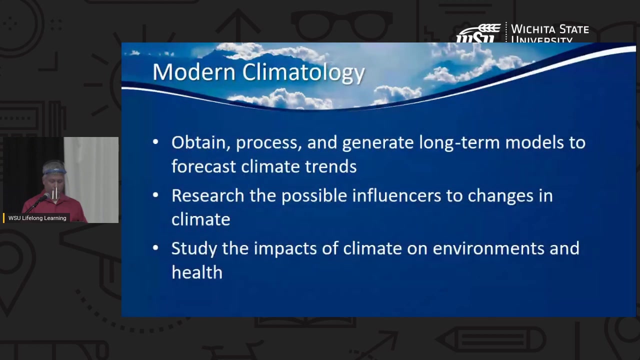 There's also ancient written records. It's part of how we're how we're able to ascertain the Roman warm period, because we have some limited records from Romans, or what we believe were Romans of that time, that indicate that it was a warm period of time in history. 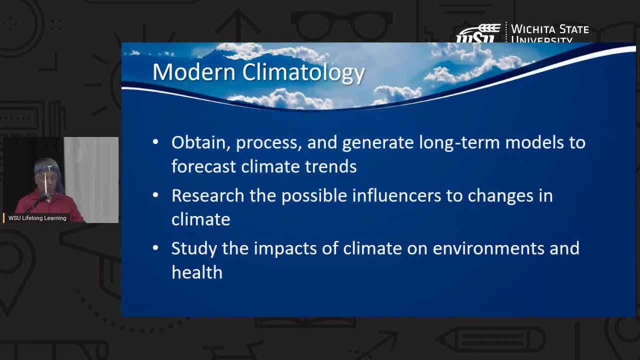 Now moving on to more modern climatology. what we do, you know: we obtain a process and we generate our long-term models to help forecast climate trends. These forecasts can be anywhere from a few months to several decades. There are, and that's. 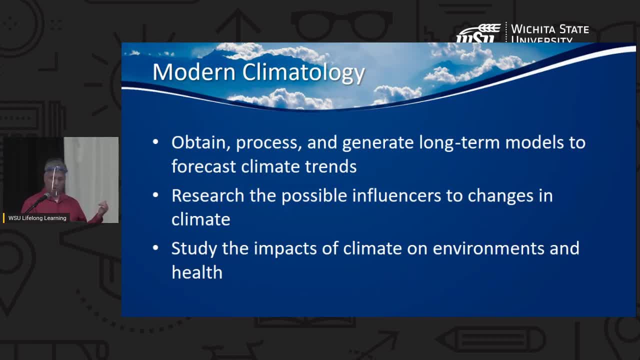 that's where you get some of those models that say, like what, what was mentioned in that first- well technically second- video where you had the one announcer talking about? oh yeah, if we don't do anything, it's going to be another four to eight degrees warmer by the end of the. 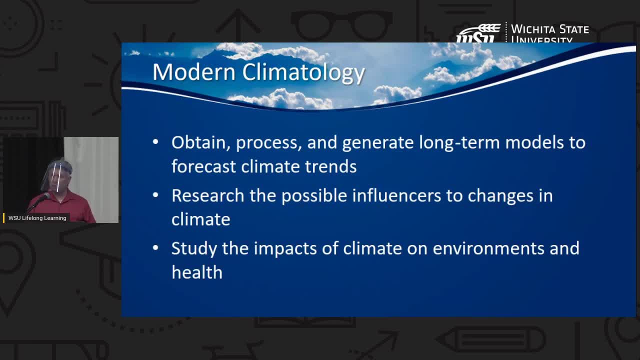 the the century. Well, that's coming out of somebody's model that they've processed, And they process that based upon a lot of different data, some very similar to what we do in meteorology, And then some making assumptions based upon the atmospheric chemistry. 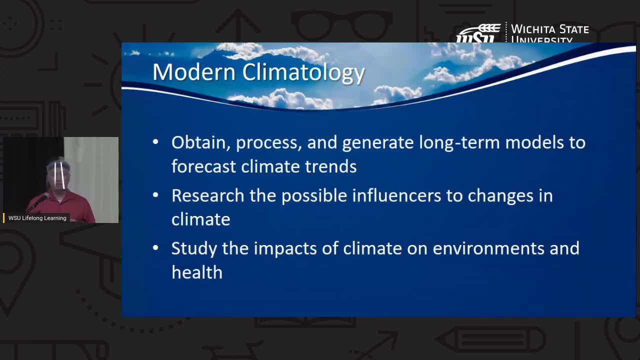 that's going on and where it's expected to continue. Many of those models take into account what the what industry has been and how much pollutants have been put into the air, how much carbon dioxide, how much other chlorofluorocarbons make it up into the atmosphere. 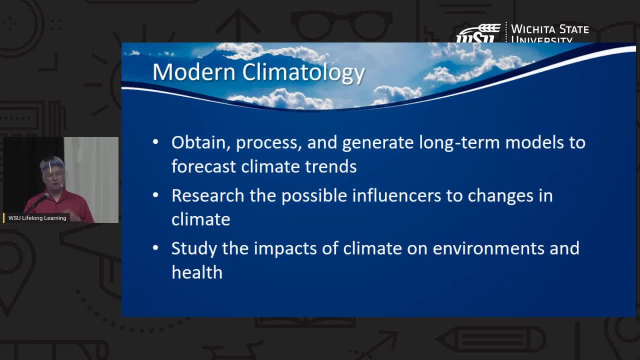 And they make assumptions based upon that as to how much energy is going to be trapped into the atmosphere and continue to warm the the atmosphere as well as warming the oceans, which is something that we haven't touched on too much, But there's a 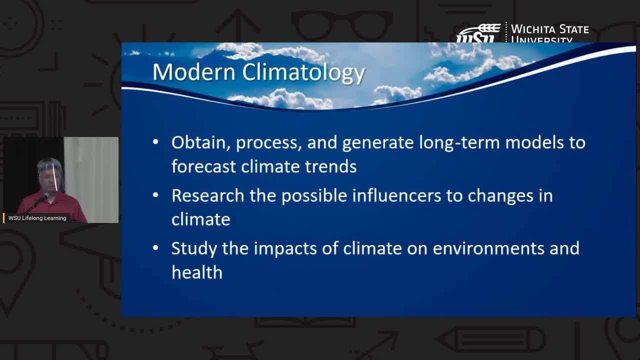 a lot of heat, not a lot of temperature, but a lot of heat that can be trapped in our ocean bodies, And so that's also part of the numerical modeling that is done with climatology, because they are making assumptions based upon how much of that heat that does. 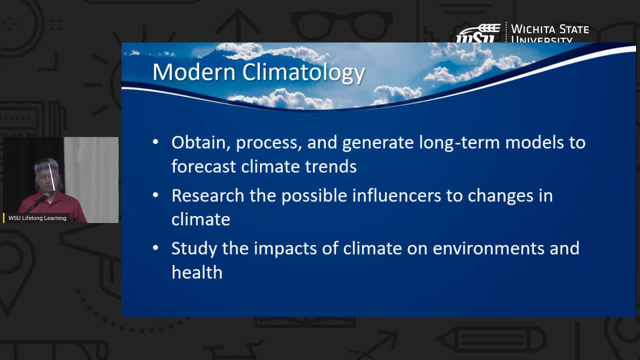 come in gets trapped by our oceans And some of those changes, because the oceans are so big, are very hard to notice. We do know that there is some change in in oceanic temperature, But it's the oceans help serve as a heat sink for the atmosphere. 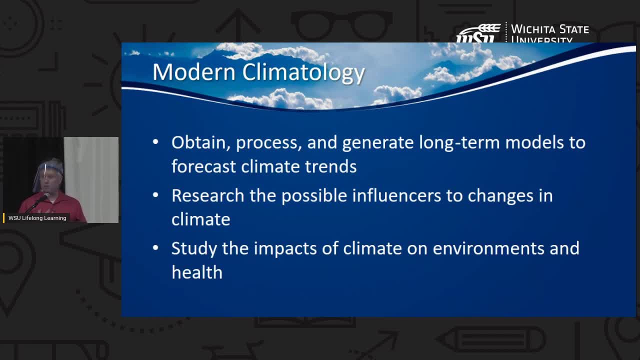 So our oceans kind of do a little bit of protecting of us from additional warming that might actually happen. So climatologists also research the possible influencers to changes in the climate And they also do some studies of impacts or potential impacts on environment and health. 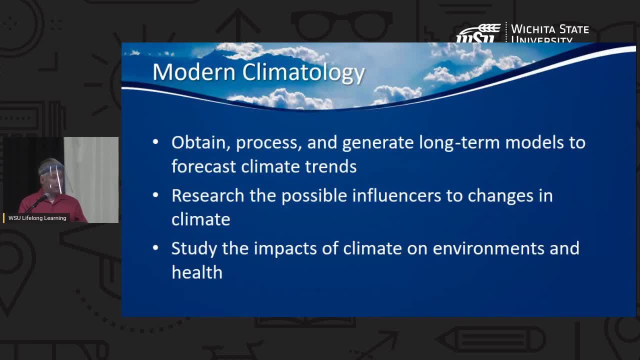 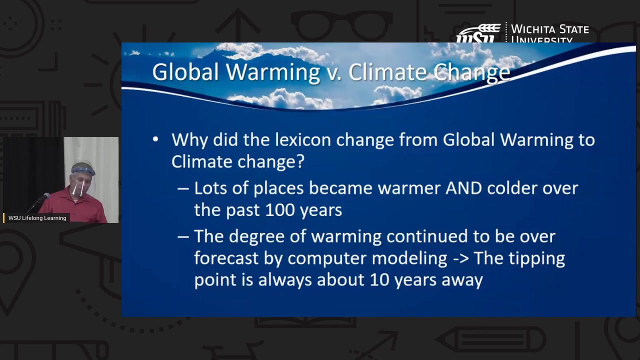 You know, certainly in highly polluted parts of the world there is a higher incidence of respiratory illnesses and things of that nature, And so climate climatologists also do some studies as it relates to that. So global warming versus climate change. 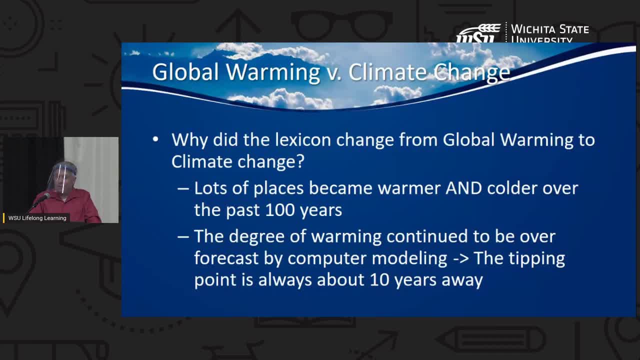 It was for a long time, especially when I was a young kid. You never heard the talk of climate change. It was never climate change, It was always global warming when I was a kid, If you went back even a little bit further- 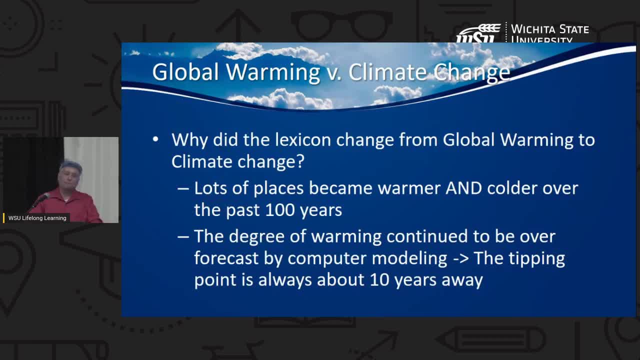 it was global cooling They had. at the very first Earth Day there was thought that the Earth was going to because of all of the industry. it was going to actually cool off and freeze us all, And then it turned out that the next handful of years were pretty warm and it became global warming. 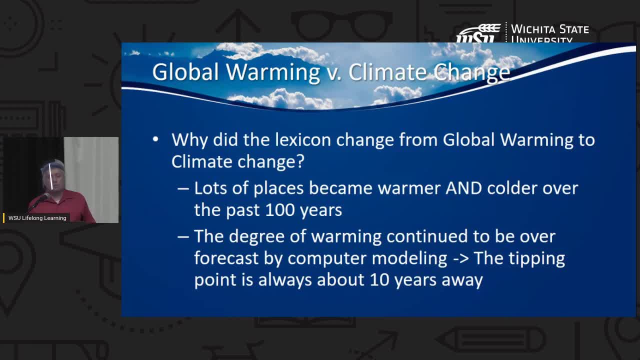 And now it's kind of more along the lines of climate change. There's been a period of time where things have leveled off or shown some evidence of leveling off, particularly during the 90s, 90s into the early 2000s. 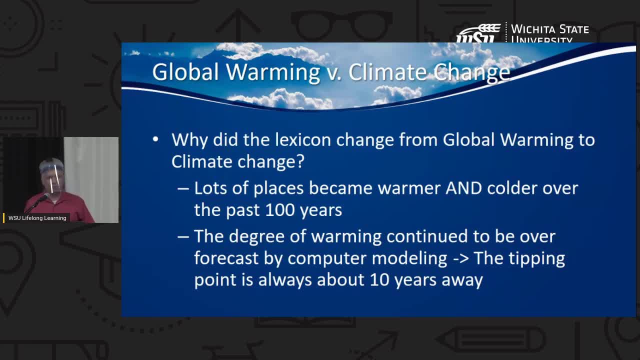 Now it is possible that possible, if not probable, that that period of time has kind of come to an end and we're seeing kind of things spike a little bit again. But the reality is, if we look at a global map, especially if we look in the last 10 to 15 years, 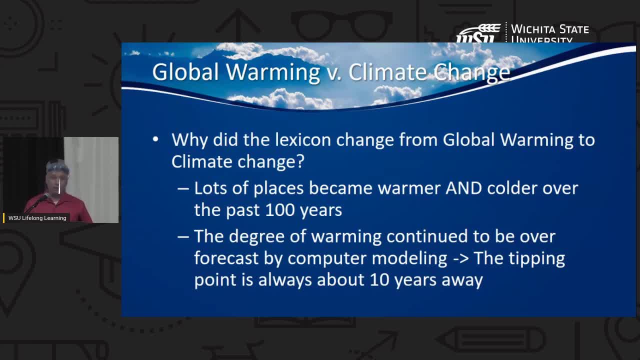 which is in that window where we've got a lot of pretty good observations from our satellites of the surface temperature. over time lots of places become warmer and lots of places become colder over the last 100 years, And so it makes that a lot murkier than what maybe we'd like to see. 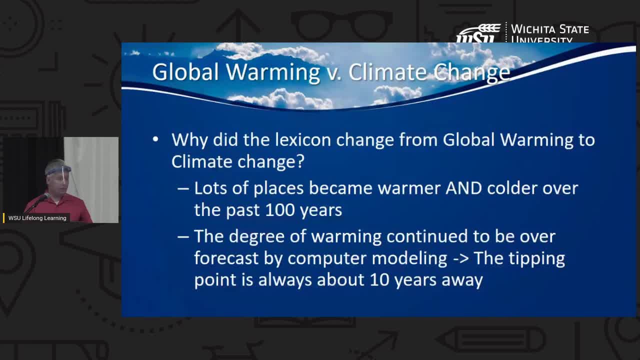 The degree of warming continues to be over forecast by computer models. That's been a problem for as long as I know. I do think that, just like with our modeling for our meteorological models like the ECM and others, because we're able to drop in really, really massive computers- 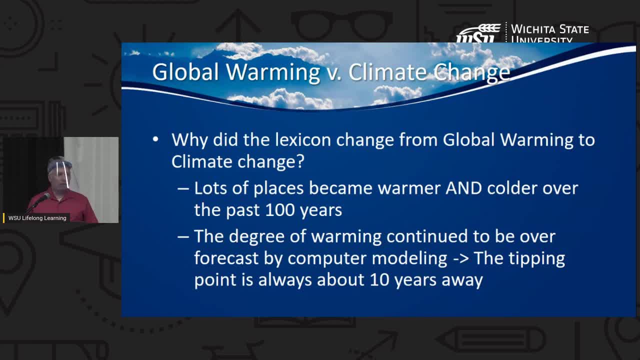 to hack away at data, that those models have a lot more potential to become improved. But the problem is we can't forecast with a whole lot of accuracy seven days out. How can we forecast really accurately 20 years out? And there's some real 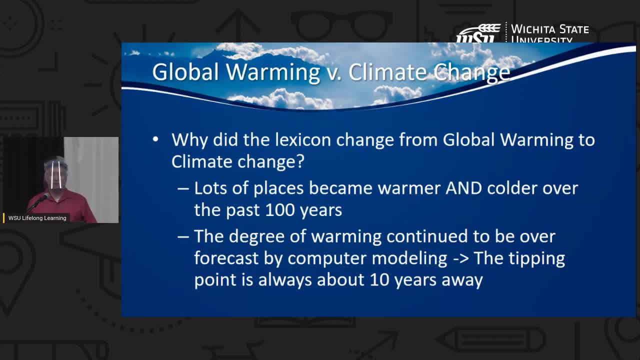 that's a real question to have. If we can't forecast a week out, why can't? why can we forecast years out? In some respects, we can forecast years out because there are certain some of the things that are impacting our weather in the short term. 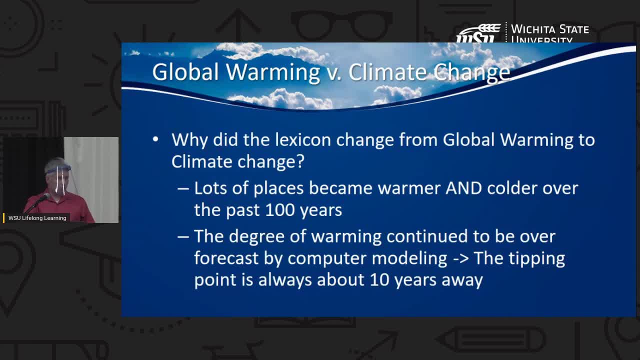 are things we can kind of ignore with those longer term forecasts. Some of the longer term forecasts are based upon, again: what do we have in terms of atmospheric pollution? What do we have going up into the atmosphere and staying in the atmosphere in terms of carbon dioxide? 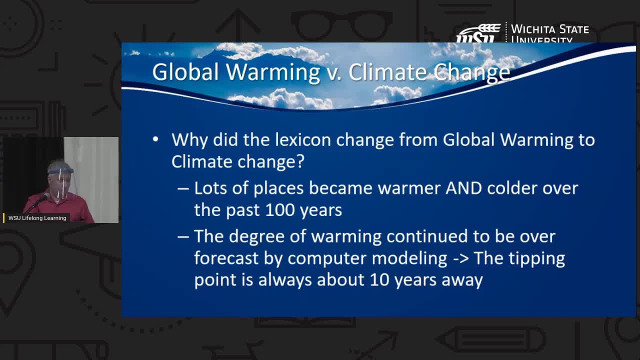 What do we think in terms of mitigation efforts to help offset climate change? Well, I'm continuing down that rat hole that makes climate modeling not really accurate either. That's why you probably always hear- or well, I always hear- that the end is. 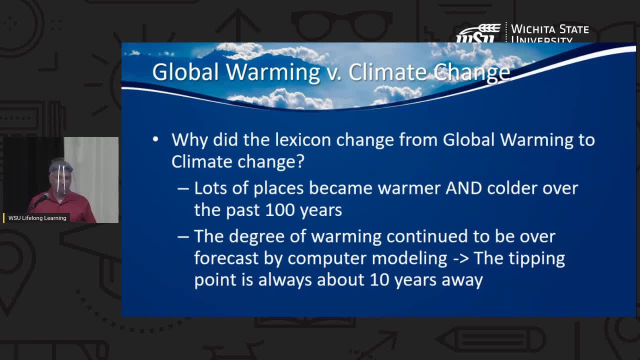 you know, the tipping point is always 10 years away, or five years away, or 15 years away. It's always a little bit away. If we don't do something now, it's over, It's over in another few years. We hear this a lot more during presidential election years as well. 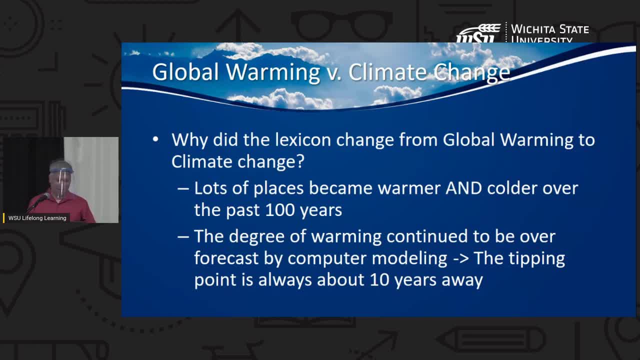 as it turns out. I don't know about anybody else, but I'm ready to have this election cycle done. But you know, like with short-term forecasting, you've got so many different elements that go into these long-term models. It is very. 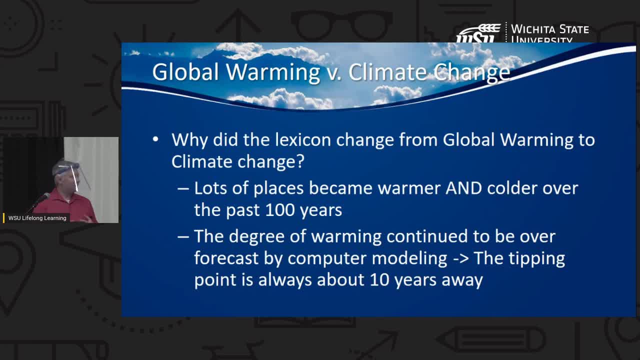 very challenging to come up with anything other than a fairly general guess. In one of our previous class periods, someone brought up the Farmer's Almanac And you know we talked briefly about how the Farmer's Almanac is interesting. 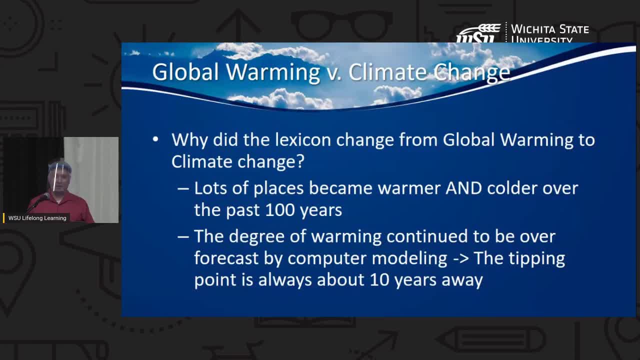 but you know their forecasts are very, very vague if you look at them, And they've also been shown to be pretty inaccurate, even given their vagueness. At best your Farmer's Almanac is maybe 50% correct. 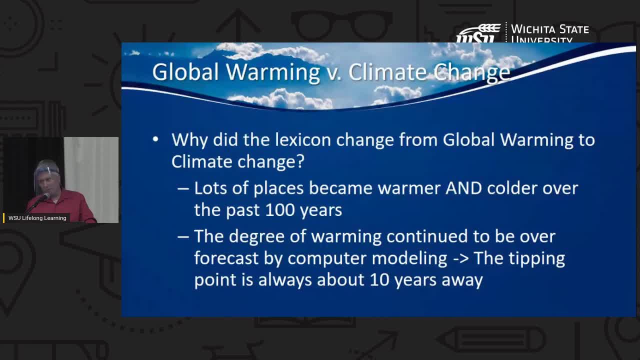 which, given the fact that they say it's going to be dry or wet, basically dry and warm or wet and cold, or you know things like that- it's kind of flipping a coin. Sometimes it feels that same way when we're talking about climate modeling. 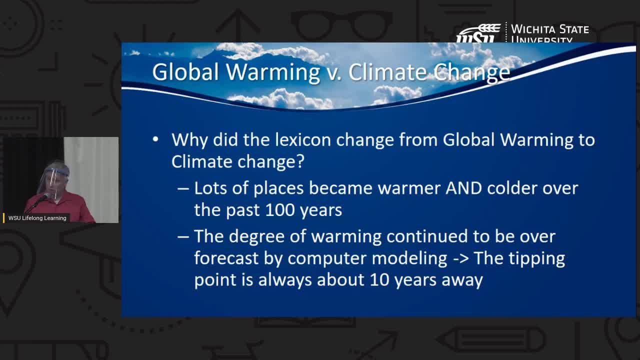 But again, as we move forward we learn more and we make those models a little bit more sophisticated with time- And I you know this is me guessing- but I'm pretty certain that another 50 years from now those models will be a lot more accurate. 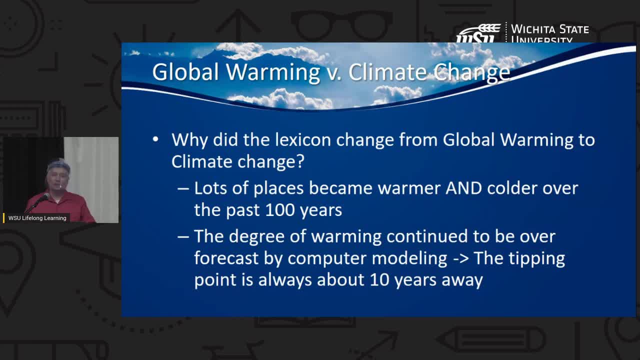 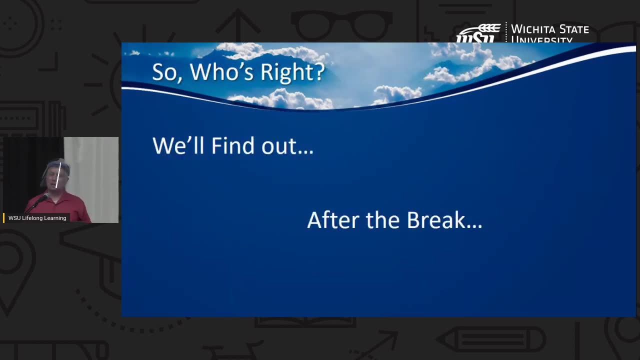 And we hope that at the point that it's more accurate that we haven't gone beyond that tipping point that we keep telling ourselves that is 10 years away. Any questions? Because I got lots of time. I build in lots of time on purpose so that we can talk about these things. 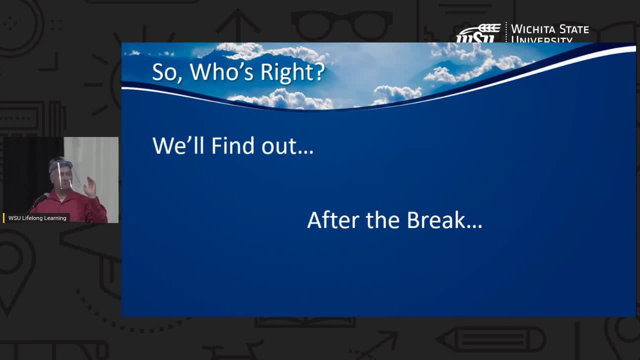 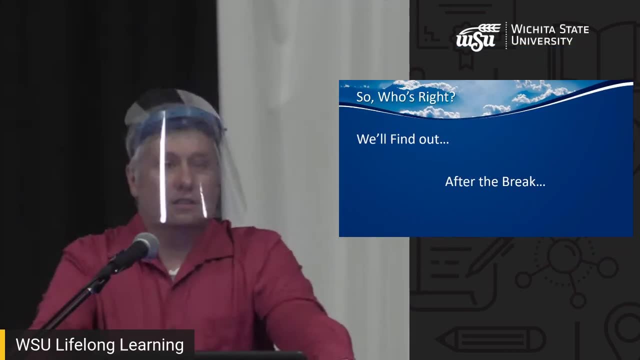 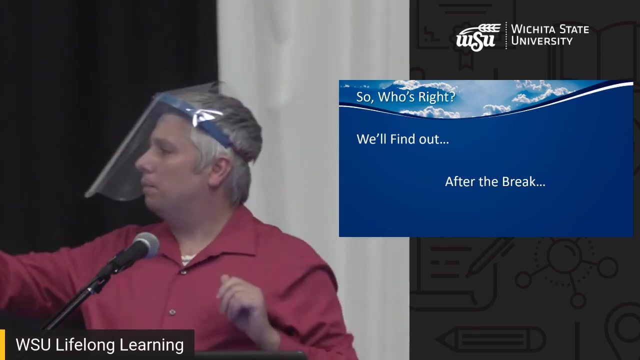 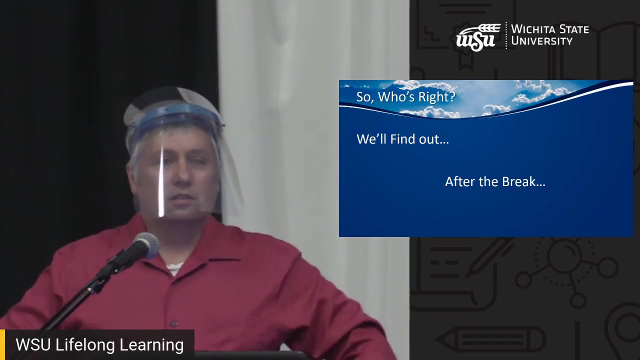 If you want to, if you, if you don't, we're going to fly through this class. Oh yes, Greta. Greta Thunberg, Actually, can you come up and talk into the mic? Oh, okay. 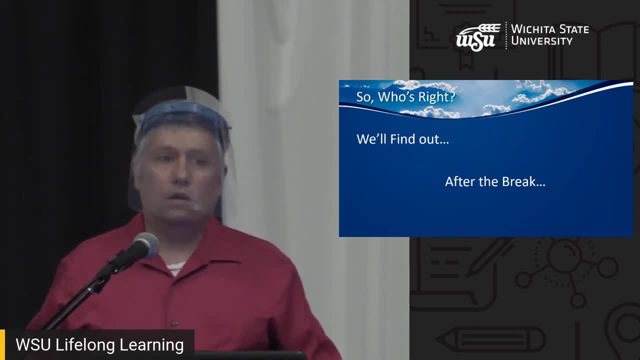 The. the question was: could we do some bad stuff because we're we're freaked out in terms of mitigating global warming, And there was a reference to Greta Thunberg or Thunberg or whatever. I the young, 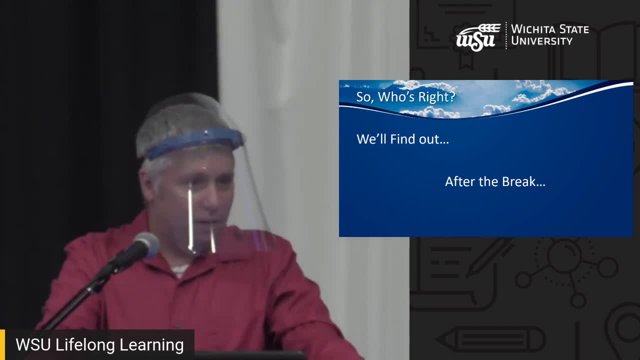 I think 12, maybe 15 year old, something, something like that, The younger kid who's out there getting testing and and telling, being that voice for that next generation of of of children who you know are concerned about. 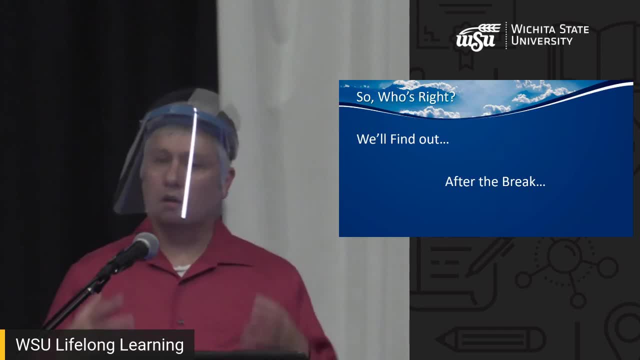 oh my God, all of you old people are ruining everything for us. Everything that that we do has both positive and negative repercussions. It simply does. You're stealing my thunder from the end of the class, but in large measure, yeah. 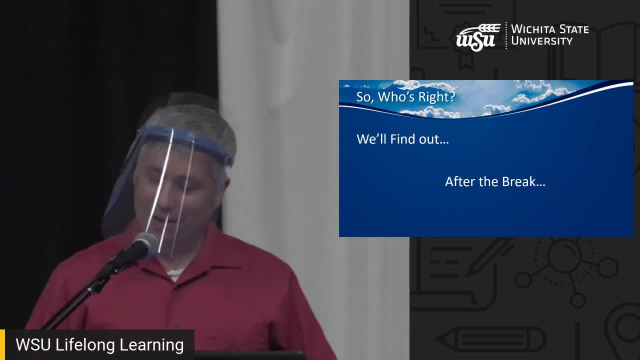 I mean, there are things that we can do that hurt us economically and maybe don't have the payoff in terms of the environment that we're looking for, But then you get into the murky water of at what point you know what, what? 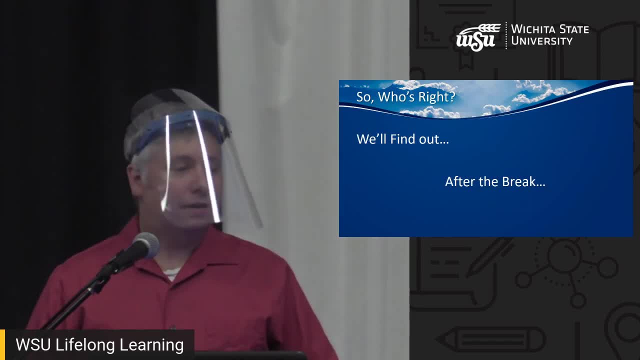 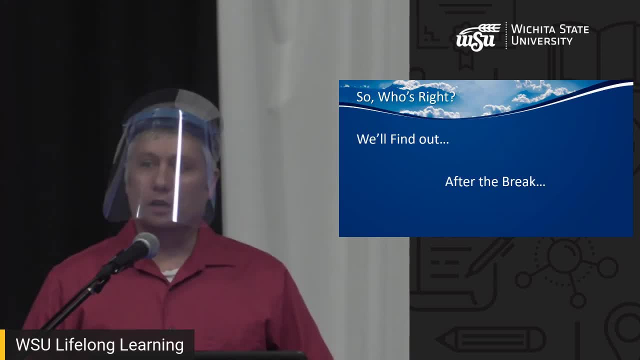 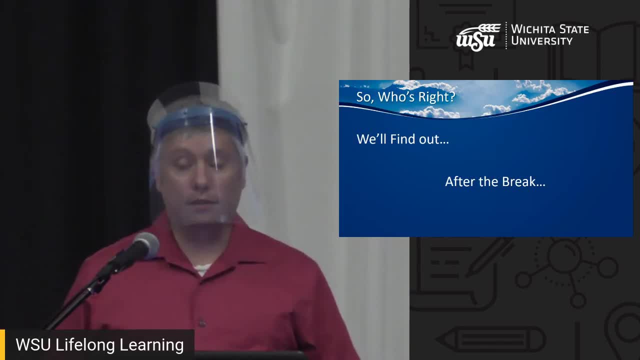 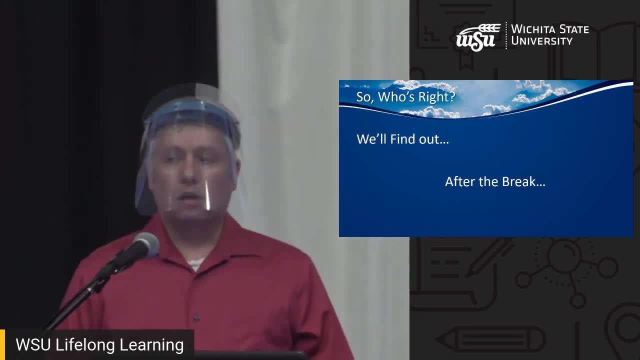 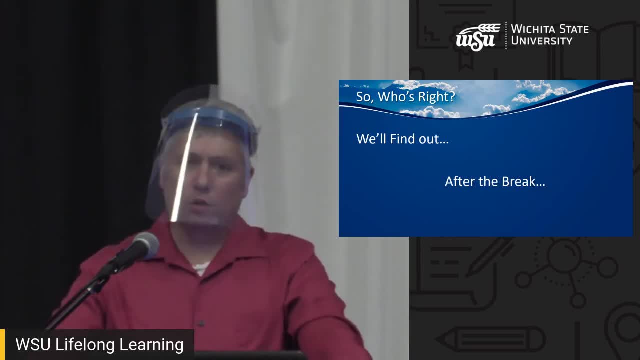 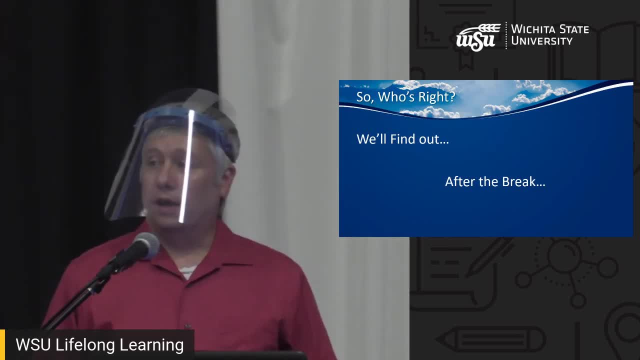 what, what, and for those of you who may not know, El Nino or La Nina, which is the opposite of El Nino, is an oscillation of. it's basically the easy way to describe it is. it is a sloshing sort of. 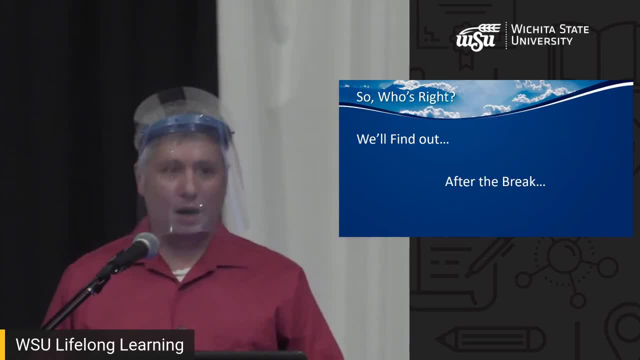 back and forth of oceanic water whereby in an El Nino you have slightly warmer water off of the west coast of the US- west-southwest coast of the US- versus La Nina, where it's actually kind of cooler in that area. Well, just something as simple as 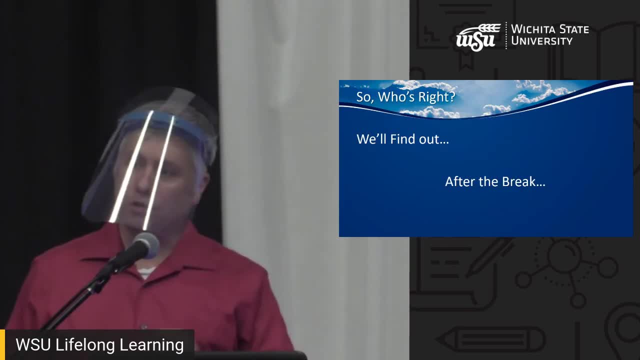 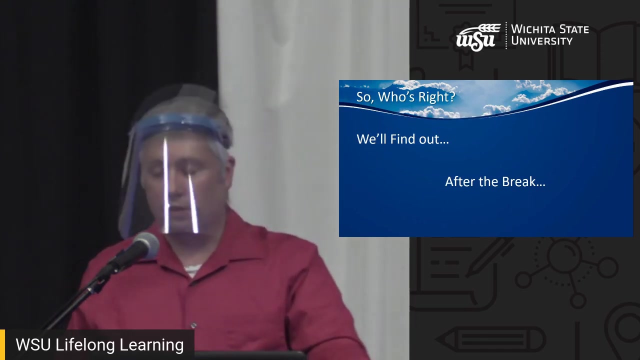 the oceans, shifting their temperatures and their waters back and forth has a dramatic impact on the weather across the US, especially in certain parts of the country And, for example, one of the big storms that somebody remembered from their childhood, that impacted Kansas and up through the upper Midwest and crossed into the northeast. was on Armistice Day in 1940, one of the biggest, biggest snowstorms out there of the 20th century. Well, that happened to be occurring during an El Nino year, where much more moisture was available to that system and it was likely that it was enhancing. 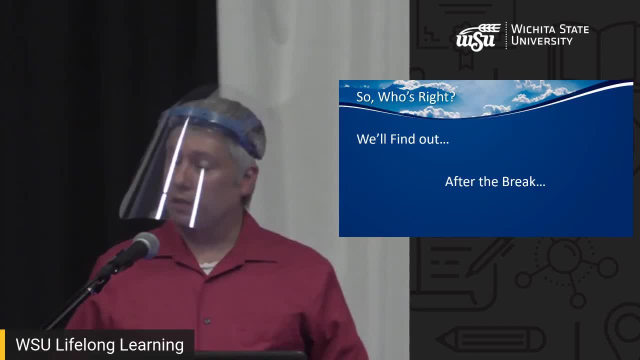 that Now here's where I'm pulling around to the payoff. We really had very little to any idea of what El Nino even was until about 20 years later, and we really didn't know as much as we know now until really about the mid-1980s. And so here you have something that over a short period of time. typically an El Nino. La Nina impacts the weather for about a year or two tops more stronger, one maybe toward the two-year range. But you have these major influencers that we didn't even know about until a handful of years ago. 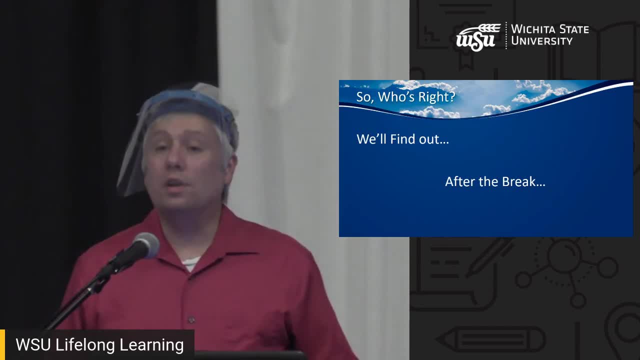 And so what I try to tell people is: you know who knows what influencers on the weather and the climate we still don't know about? We're still in discovery in this science. We do know a lot. We're learning a lot, really. 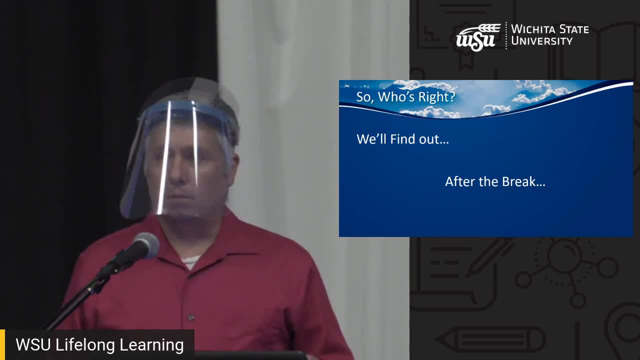 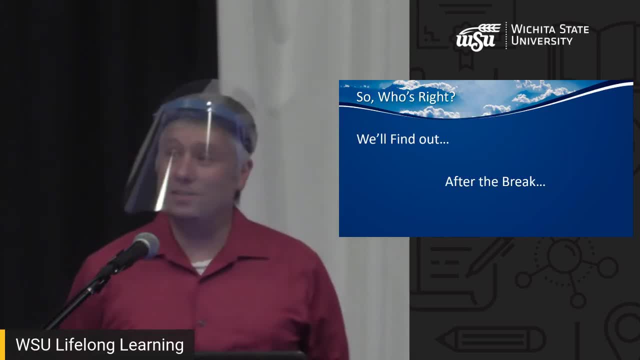 And we don't know what's going on And we don't know what's going on. And we don't know what's going on, We could be kind of offsetting something that we maybe didn't intend to result in some consequences on. So that was a lengthy answer to fill time. 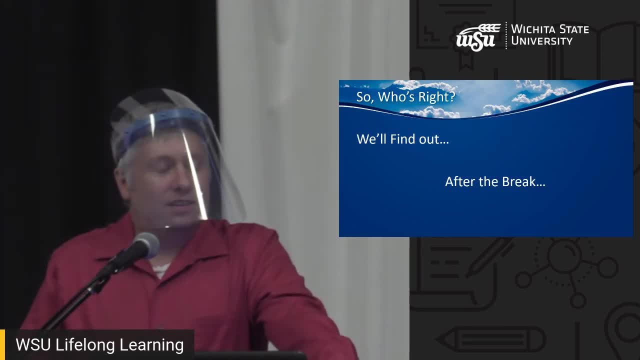 Yeah, You know, there's been a lot of study of it And it's still something that's going to be going on, And I think that's going to be going on that we don't fully understand, you know, and that's that's part of why we have the discussions. 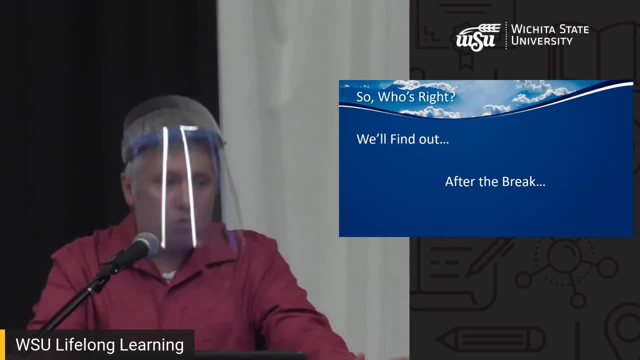 that we have today back and forth is: we know that the atmosphere, that that the climate does go through cycles, um, and we know that those cycles are about a thousand to two thousand years in length. where we're, we'll get warm, then we'll go through an ice age and then we'll warm back up. 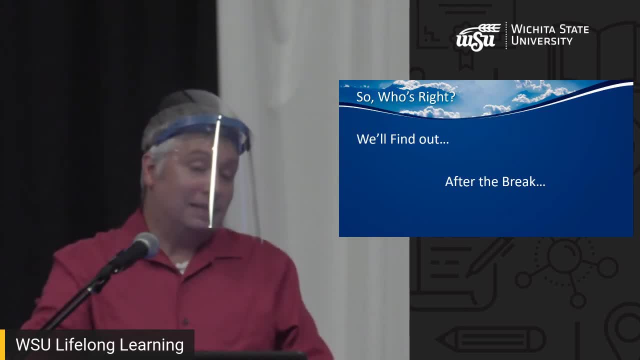 um, do we fully understand? why not fully? um, if we did, we'd probably have a lot better of understanding and ability to um to determine whether what's going on now is an anomaly or not. uh, because we know, yeah, it is about the right time for us to be coming back up toward more of a maximum. uh, and again there are. 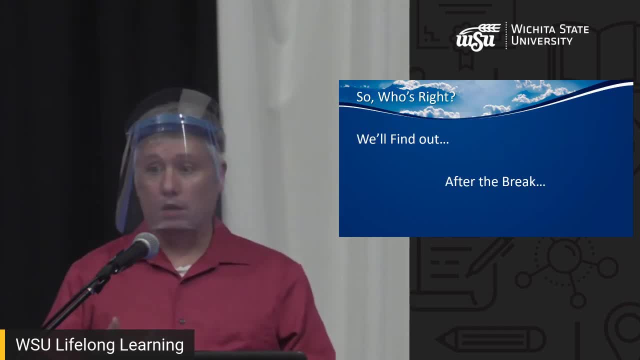 a lot of longer term trends that impact this. um, you know, we know that the sun and the energy the sun produces and how it produces across the- uh, planet changes with time. um, some of that was: you know, the tilt of the earth on its own has an impact on the, the climate. um, and those are of 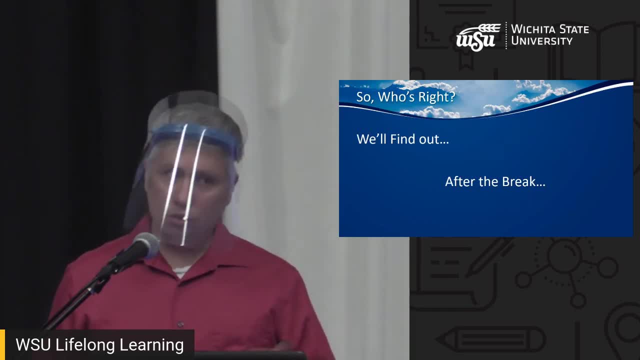 course, are over long periods of time, so they're not a huge role in these shorter thousand year cycles, um. but we know that the sun and the energy the sun produces and how it produces across the, but we know we go through those those warming and cooling periods, so we know we're coming out. 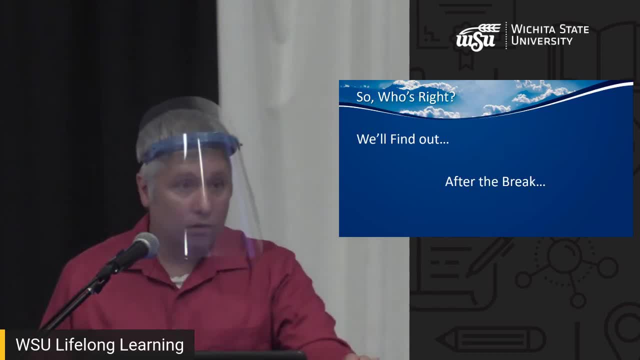 what we do know. we know we're coming out of an ice age. there was an ice age about 400 years ago. we're we're on the out of it now. what we don't know is how much of that is that natural cycle and how much of it is what we're putting into that. uh, there are a lot more humans on the planet. 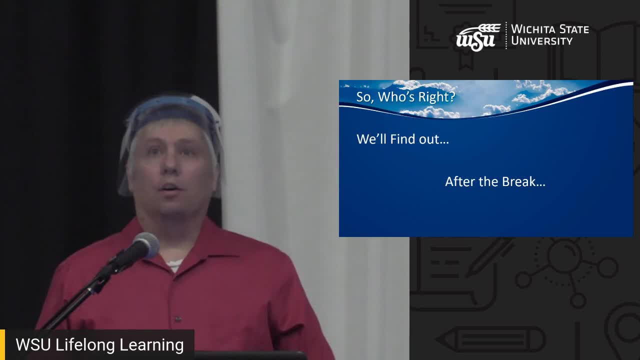 than there were before, and we're not going to be able to figure out how much of that is 400 years ago. there are also a lot more cars on the planet than there were 400 years ago and a lot more factories. i mean, we, we didn't have any of that stuff back then, so that's really where a lot. 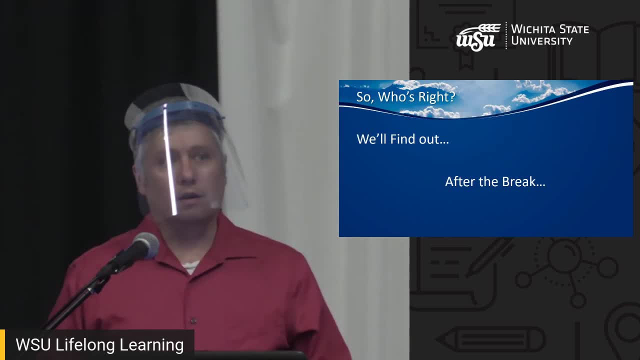 of this debate is: is what is the impact of natural cycles versus what is the impact of human influence? and there's still again, there's a lot that we, that we try to surmise, but don't 100 know in in these areas. anything else? okay, oh, yeah, yeah, go for it. 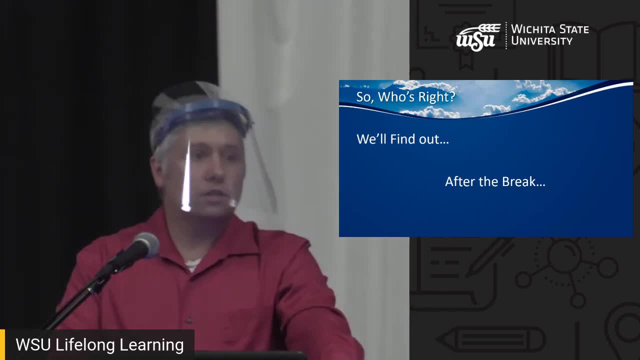 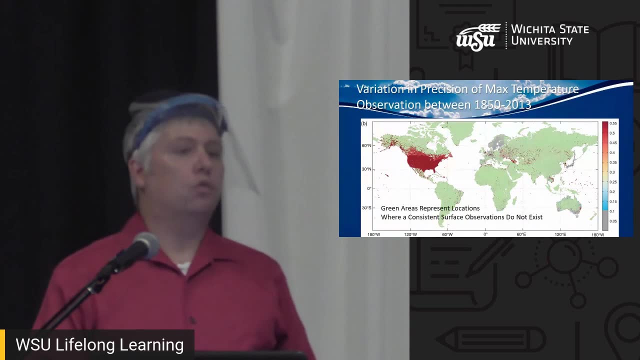 um, yeah, if we were to include the satellites in there, because that, that image- and we're referring to right here, uh, that image is uh looking at the actual physical monitoring locations. those are all those, all those dots are- are a, a, a weather station somewhere on the surface. if we were to look at that with satellites, you would 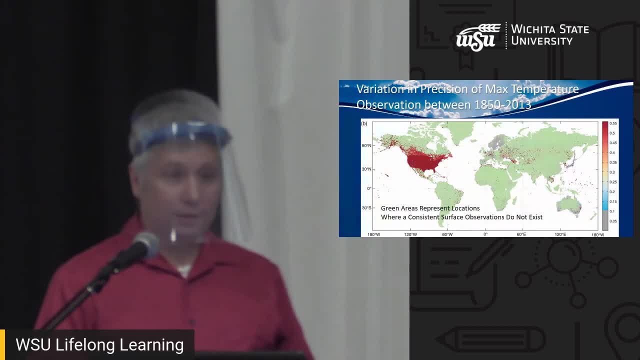 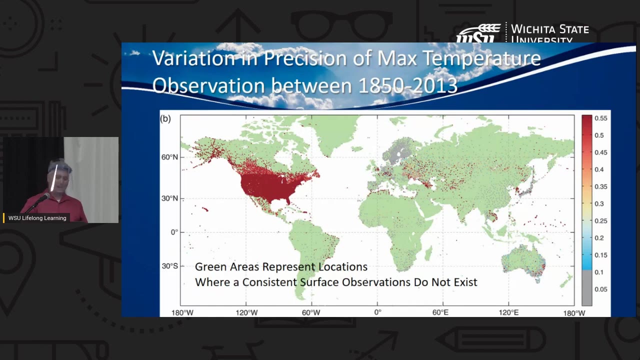 have almost a completely covered map in red today. so uh, yeah, i mean the last 30 years- we can get a pretty good feel for the surface temperature. but even the satellite measurements of the surface have their limitations. it can't get the surface temperature through a cloud. 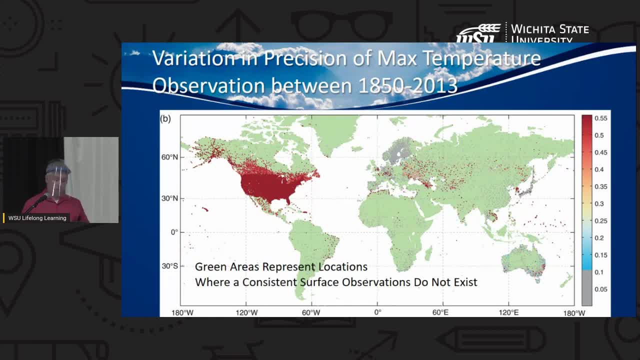 for example. so we can kind of ascertain- uh, well, we can, we can get our cloud top temperatures, which can be very useful for meteorologists as well. uh, but we can only get the actual surface temperatures, or a really good estimate. it's still not perfect, but it's a really good estimate. 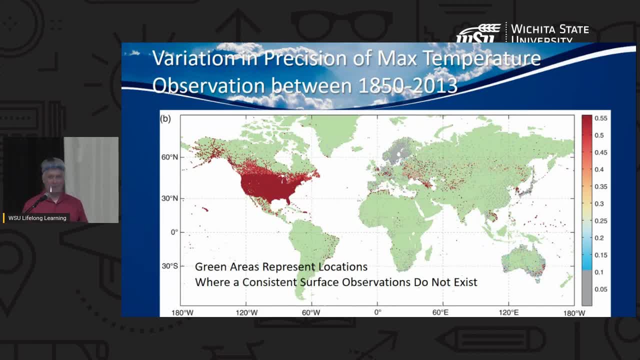 these days of what the actual temperature is at the surface, if it's clear overhead or very close to it, um. but those satellites are constantly taking those measurements up in the uh, up in space, um, and you know, i don't know the exact frequency of it, but basically you can get if there's not. 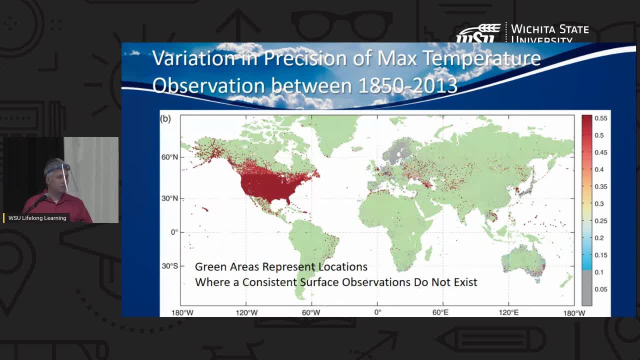 cloud, you can get a pretty good estimate at all times what is going on on the surface within like a degree or something like that. so i think that's a really good estimate. i think that's a really good estimate, so, um, and so that's why the next 50 years, once we start really getting a feel of the 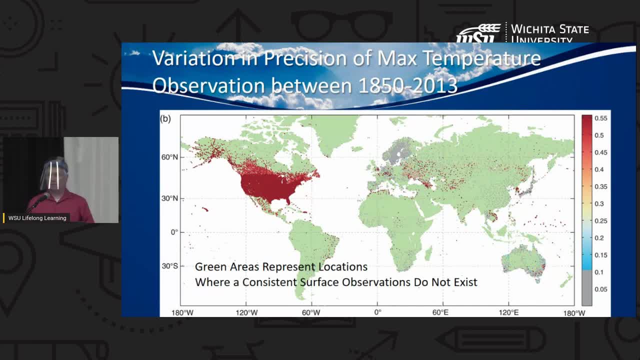 trends. uh from remote sensing is what that? it's a fancy word for the satellites taking uh measurements on the surface. um, once, we get a lot better at processing all of that data, which is going to be much, much greater- and it is already much, much greater- than what we've had for the eon. 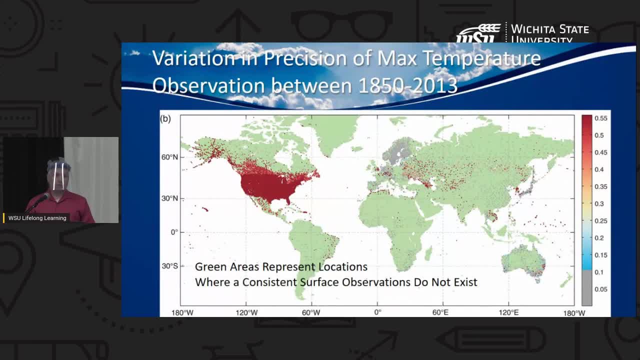 and eons, uh, that we look back on, we'll start to get a much better picture as to where we are and where we're going um, but it's going to be a long time after we're all dead before we probably really know what's going on. 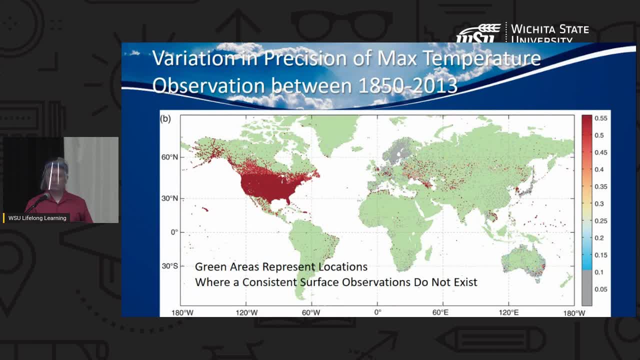 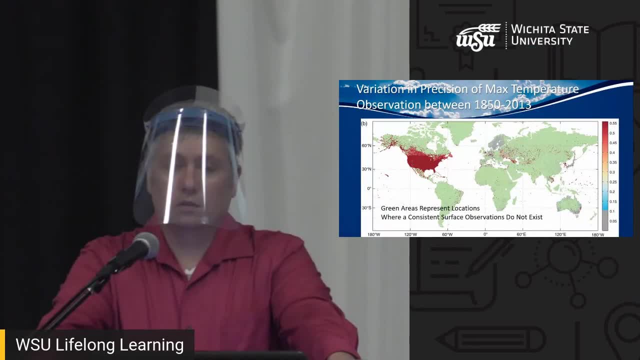 yeah, a lot of uh forest fires out there. uh, as was brought up here, california. uh, probably not from that far. um, by the time it would get to kansas it would be dispersed enough that it would be. you wouldn't probably notice it, uh, but definitely from. 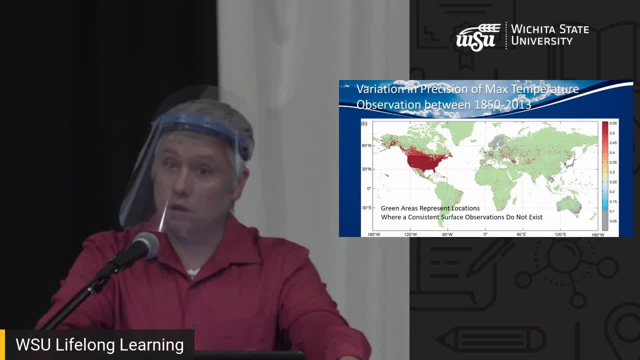 colorado, and if there's major uh forest fires uh in colorado, yeah, we can definitely see them uh in the atmosphere here in kansas. uh, now, of course it depends on what the prevailing winds are and things like that, um, but if you've got a, you know a wind that's coming, you know pointing. 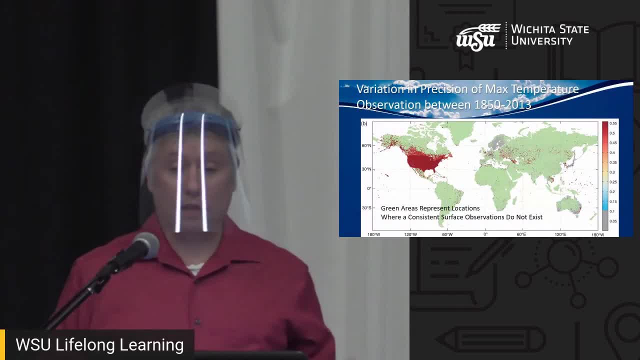 all that, you know, smoke and haze toward us absolutely, um, you would, you would, and and what you see mostly is kind of just a sky that just looks a little murky or murkier, even though it would otherwise be a, you know, a clear, mostly clear kind of day. yeah, 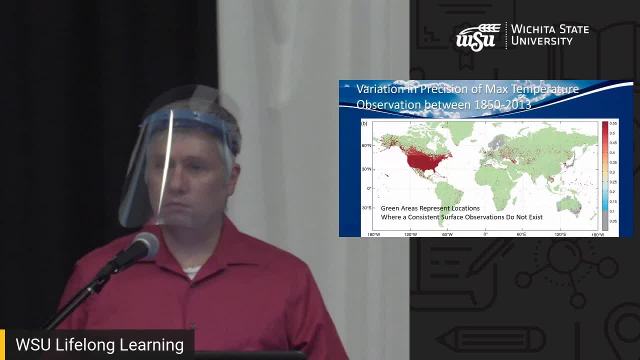 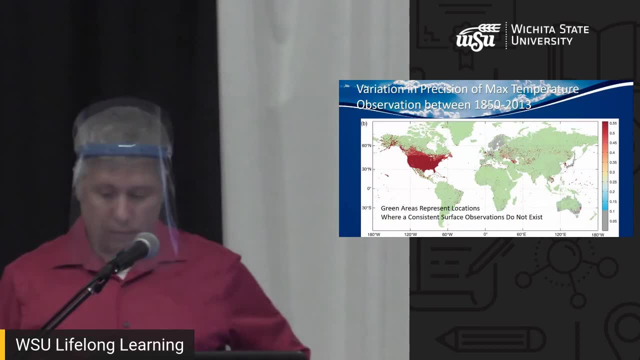 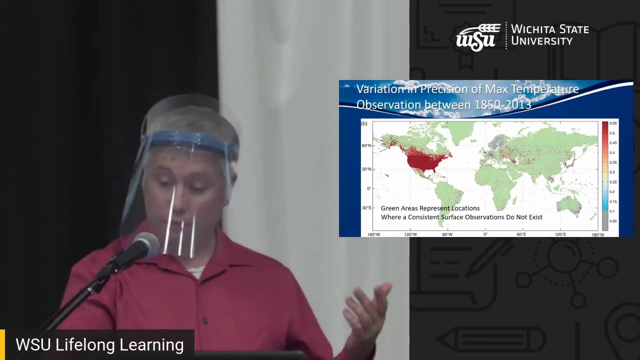 all right. well, if there's nothing else, right now it looks like we are about where we want to be and and i just let's see here, there we go. uh, 153 is what i'm seeing, 154 i just switched over to, so let's say 204. uh, we'll come back and we'll take care of the rest of the class. 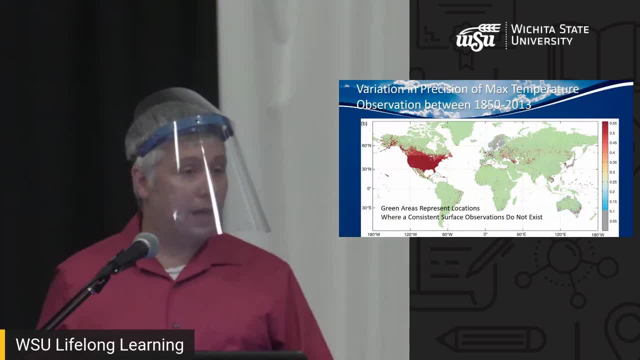 uh, if you have questions, uh, during the break, feel free to come up and ask. uh. and then one more thing. uh, i just like last class, i've got to race back to uh relieve my uh uh, fellow comrade at the wsu west location. but if you do miss me, 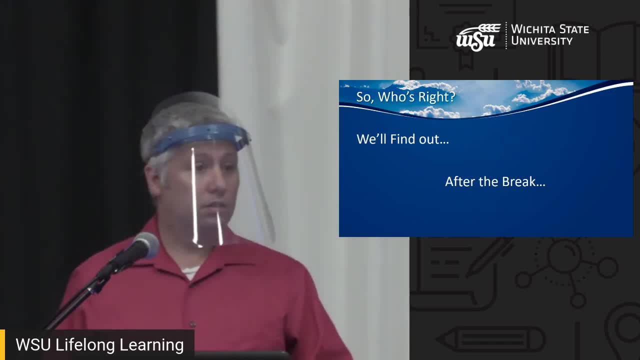 all right, okay. so, uh, uh, first half of the class we were talking about, uh, how there are two sides to this uh debate over, uh climate change and large measure. it's because we only know so much and we have to infer a lot of what we know. um, so, who's right, who's wrong? 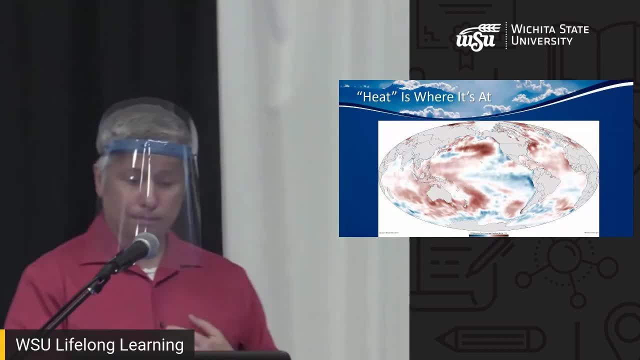 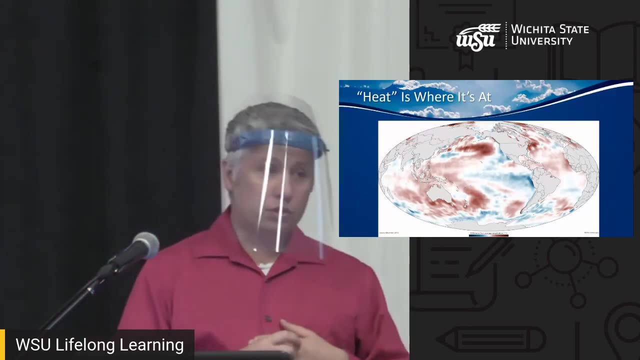 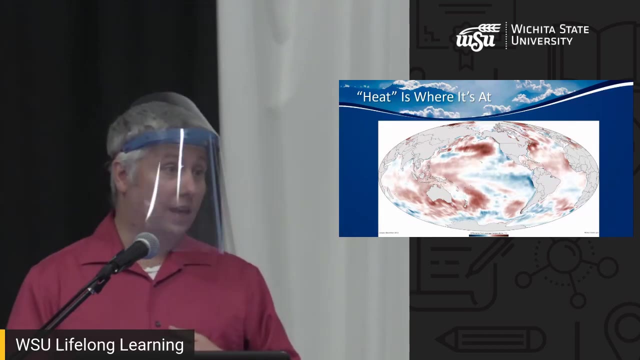 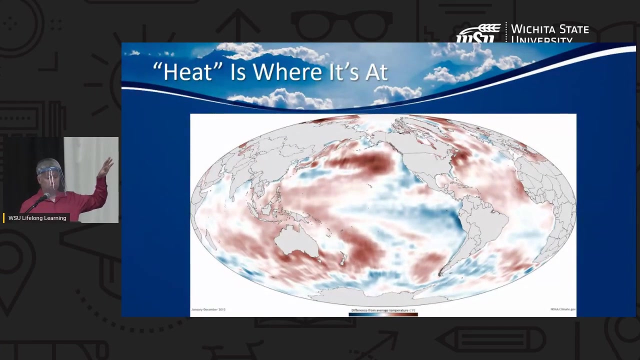 it's oftentimes hard to say- i alluded to this a little bit earlier- um, this is a uh. what we're looking at in this image is the oceans and their departure from their normal temperature. um, this again is one of the advantages that we have of the satellites, of our remote sensing. 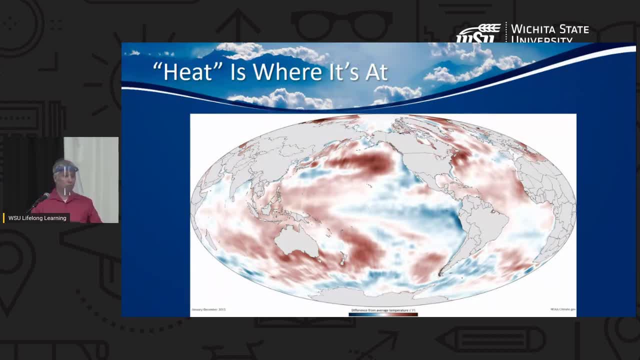 because 30 years ago we wouldn't be able to produce a a very good high resolution picture like this. this is kind of looking at the departure from our average temperature at any given point across the planet. uh, this happens to be from a period of january to december of 2013, is what it says. 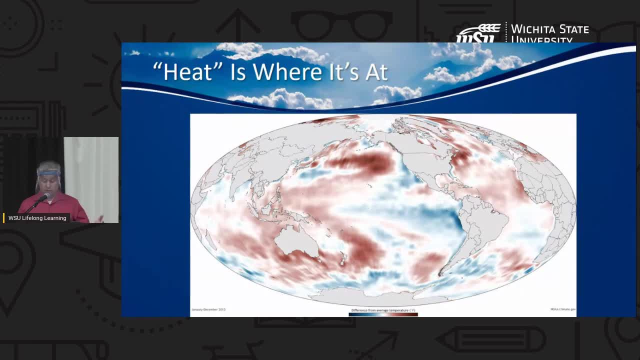 way, way tiny in the corner there, um and so what we're seeing as we look across the uh the globe is we're definitely seeing some warming uh occurring in certain parts, uh fairly large uh difference in average temperature here uh in the northern pacific uh some cooler temperatures here than average along uh some of the uh uh western coastlines. 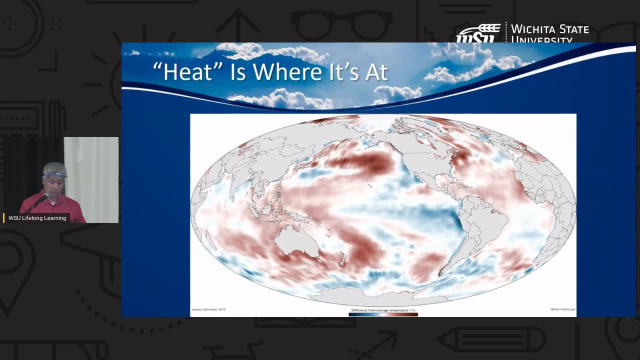 here in north and south america some more warm weather. warm, uh, ocean surface temperatures over here, um real warm again hard to see up there near the equator. so you know what we're seeing here is we are seeing some slight warming in our temperature, uh, at the surface in this image. 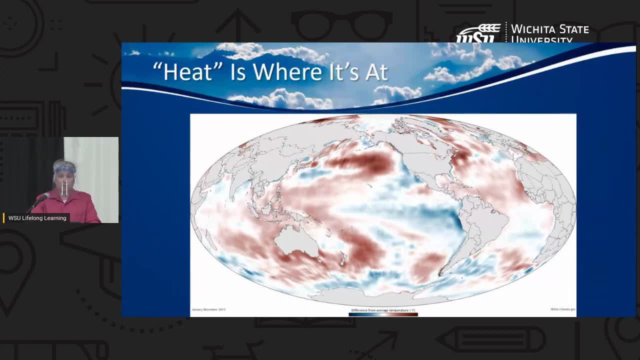 um, but you're not seeing it everywhere, but you are seeing it across a lot of a lot of it. i mean, i, i think the average person would look at an image like this and say, hmm, there's a lot of red there. um, now if we took the red and we made the red blue and the blue red, since our eyes pick up on red more? 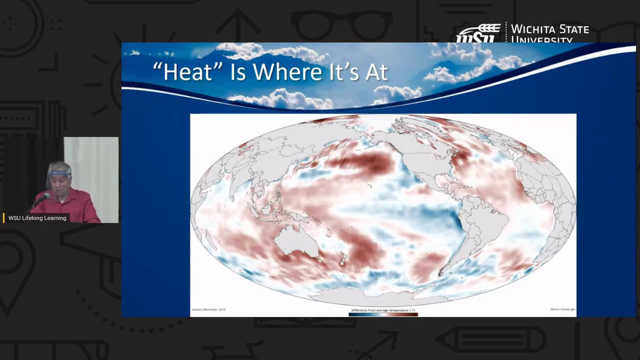 than blue? would we have the opposite jump out on at us? maybe, maybe not, i i'm not sure, but i think, uh, the average person's gonna look at this and say, at least in this year, our oceanic temperatures were definitely a little bit above normal, um, in some cases, a lot above normal. uh, these really deep reds. 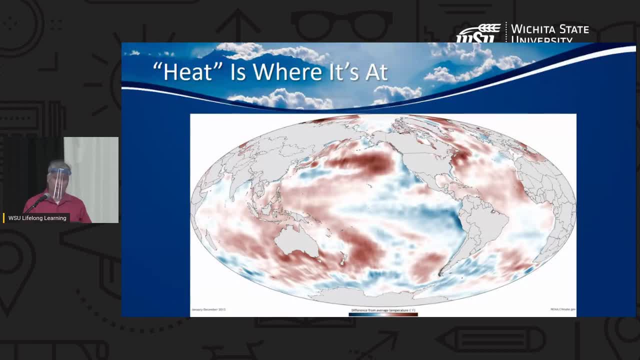 are four degrees fahrenheit warmer, that's. that's a pretty big departure from normal uh over us, uh, single year. uh, these dark blues are the exact opposite. it's about four degrees less, um, and so i mean there's there's heating going on, but there's also oceans constantly moving current around and 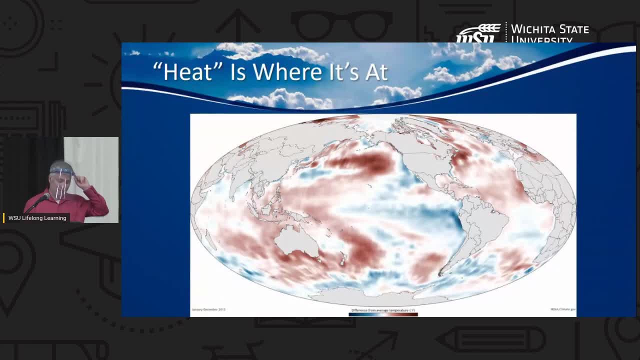 so you're always gonna going to have some warmer areas and some colder areas, and so, um, that's again what makes this whole thing murky, because you can't just take a picture and identify from the picture. but it is very anecdotal that in this period of time we are seeing a warmer ocean. 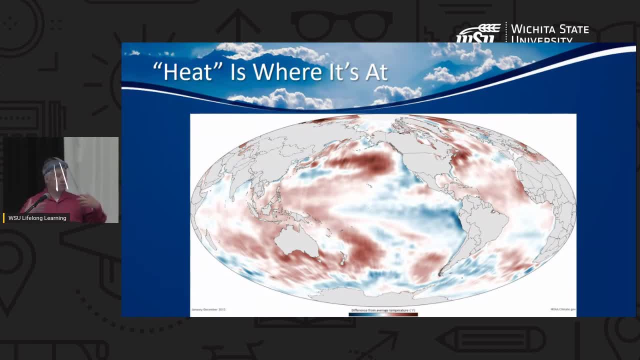 and this would bode with what has been physically observed from our satellites. uh, over the last handful of years, that the oceans are getting a little bit warmer. uh, this is also somewhat verified in some of the observations we've taken of the ph in our oceans. uh, the ph has been, uh. 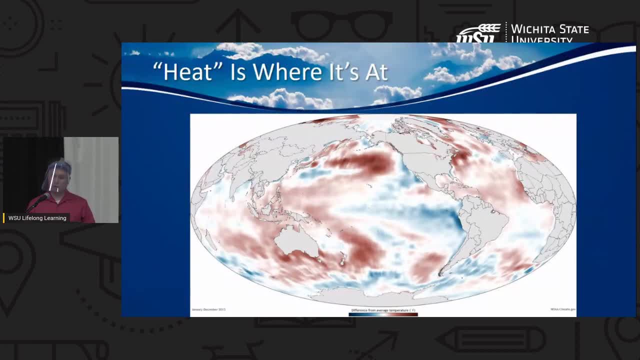 the going down. yeah, ph is going down and as the temperature goes up, uh, which is a natural thing, you could have the same cup of water at one temperature and that ph is actually going to change slightly if you increa, increase or decrease the physical temperature of your. 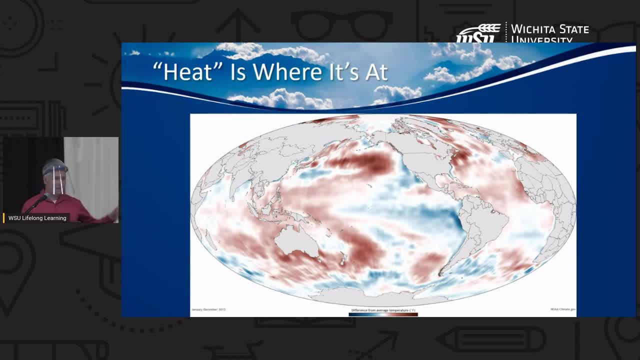 your glass of water. so, in lieu of anything else, if your temperature's changing, your ph of your water is changing, and that's what's also being observed. so we have a good feeling, at least in reach recent times, that our oceans are warming up. that bodes also with some 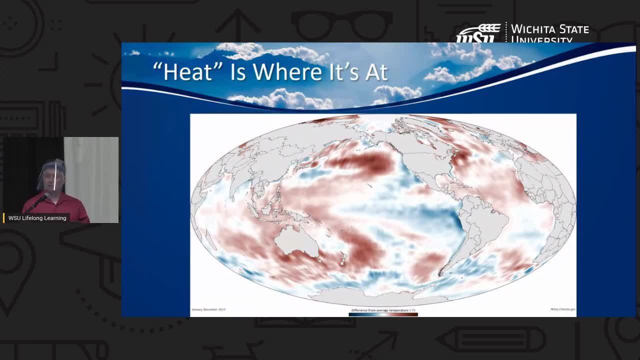 of our uh physical observations that we've had of, uh, uh, you know, you see every now and then a iceberg breaking off, or a chunk of an iceberg breaking off into the ocean. that would uh, observationally at least, in lieu of anything else, uh point toward possibly warmer water. 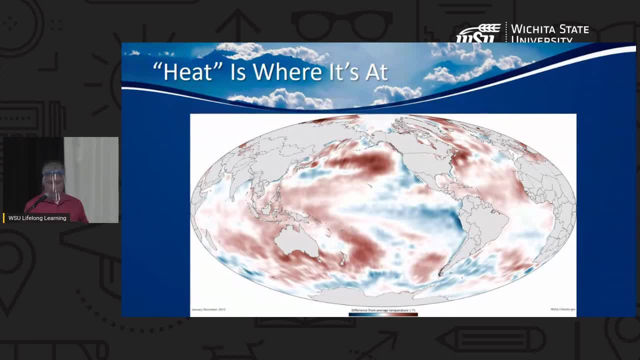 now the thing about one more one, one last thing on this thing, about this too, is that our water, our bodies of water, as i said earlier in the class period, can hold a tremendous amount of heat in them, a tremendous amount of energy. atmosphere only holds so much energy, but the oceans can hold a lot of energy, um, and. 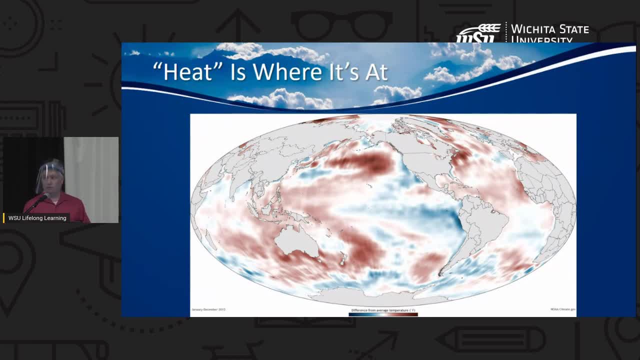 we see small changes in the ocean versus the atmosphere, there is a lot more cause for alarm. the atmosphere is not changing a whole lot, depending on who you ask. uh, in the bigger picture of things, yeah, we're talking, maybe a degree here or there, but the oceans are. 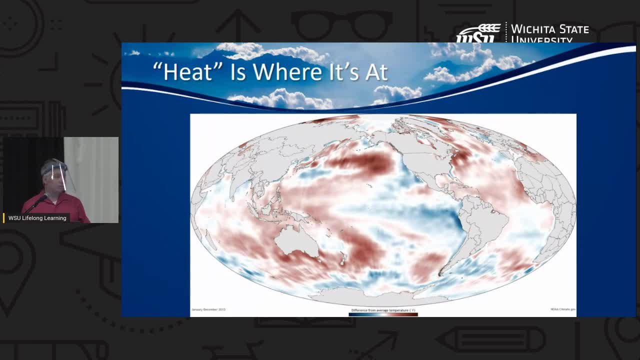 showing some fairly significant changes, and so that's where a lot of this um study right now is in terms of climate change is not so much watching the atmosphere but watching the oceans and how the oceans are changing, because there is some evidence of fairly rapid change in the oceanic temperatures. so if there's global warming, why is it colder? 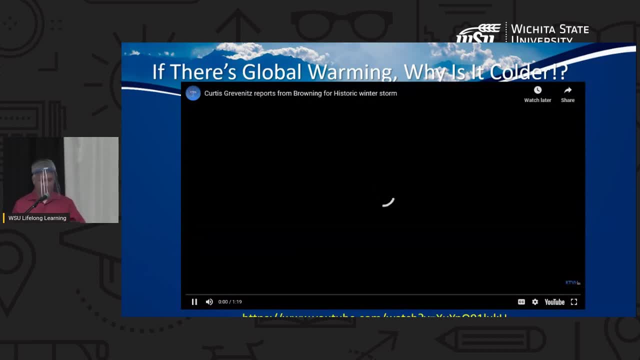 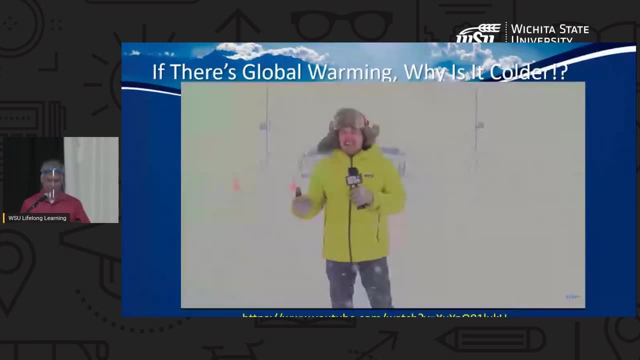 this is actually from uh, last november. um in, a major snowstorm continues to hit montana, here i'm. We're currently up just west of Browning on the High Line. Highway 2 west of Browning over to East Glacier is closed. Now I have been told that there are two snowplows that actually got stuck. 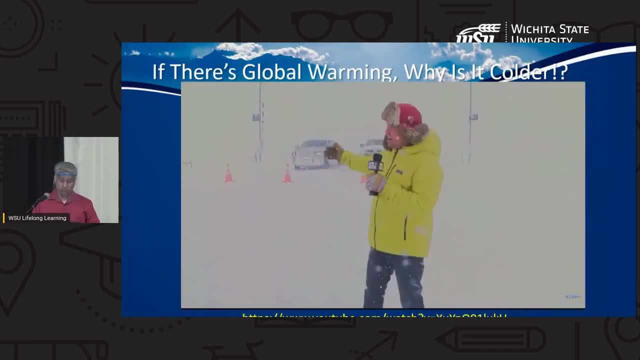 and a highway patrol car that is stuck here west of Browning, east of Glacier. The road is closed and there is no anticipated opening just yet of the road And, as you can see, blizzard conditions here up along the east side of the Rocky Mountain Front. 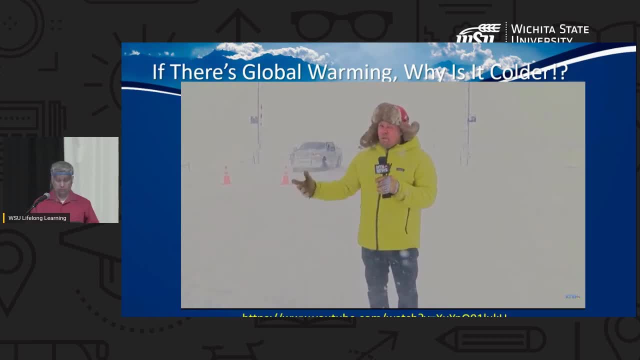 It's cold. Temperatures are about 25 degrees, wind 30, 35 miles per hour. That puts the wind chill down near zero and visibility is down near zero here as well. So it's advised to stay off the roads, and there may be more roads, like Highway 2 here. 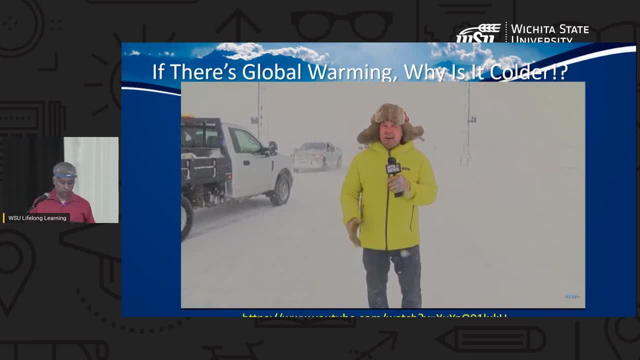 along the High Line here that gets closed down Because of these really bad weather conditions. We will continue to bring you updates from a major winter storm up here on the High Line. For now, I'm meteorologist Curtis Grevin. It's MTN News. 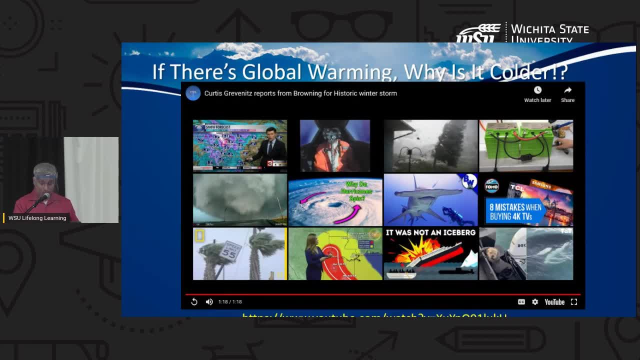 So yeah, that was from. how was it November of 2019?? I think so. It feels like that would be a decade ago the way this year has gone. That was actually a really major winter storm, Set a lot of low temperature records across the northern plains and everything like that. 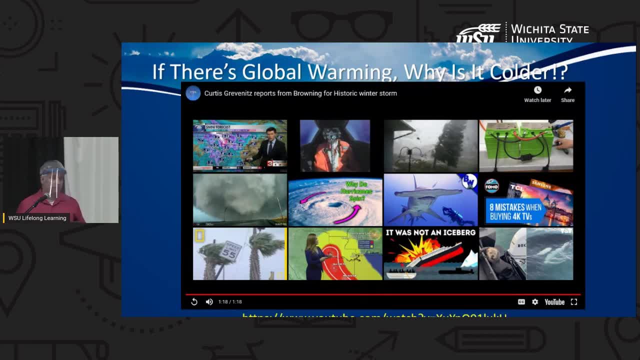 Yeah, He was in Montana And lots and lots of snow came out of it, And so you always hear from the climate change people when it gets really, really hot, We have a just massive heat wave. you hear from the- uh, you know- climate people who's to uh, uh, don't buy into, you know significant. 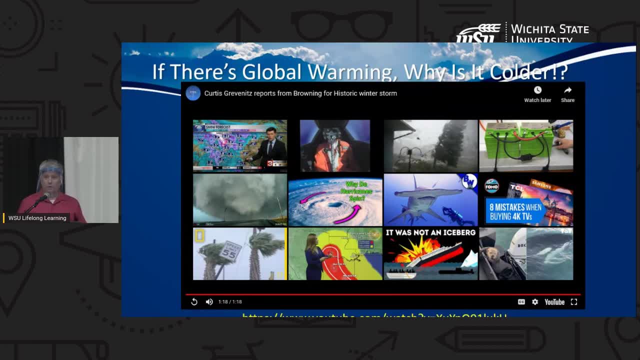 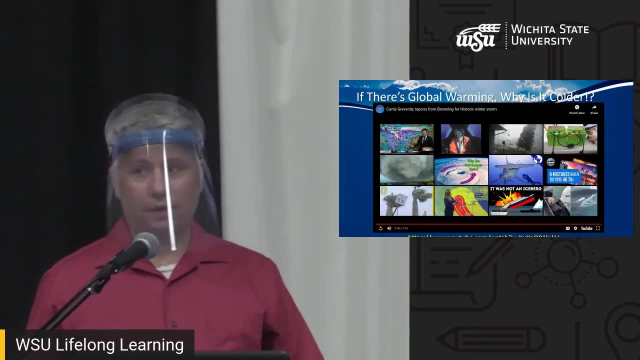 change, or at least significant change, from humans who come out of the woodwork when it does something like that. so i mean who's right, who's wrong? i mean we would like to cherry pick the, uh, the data that suits what we want it to be, uh, or the outcome that we've come up with, um, 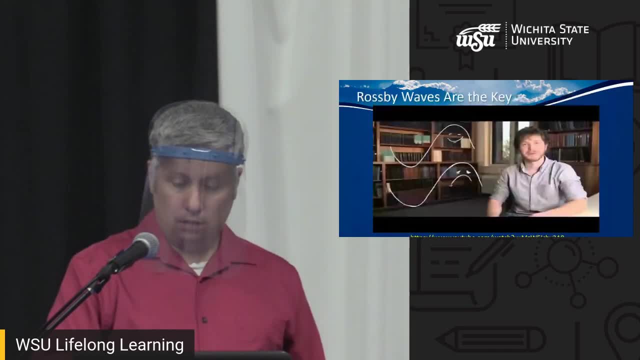 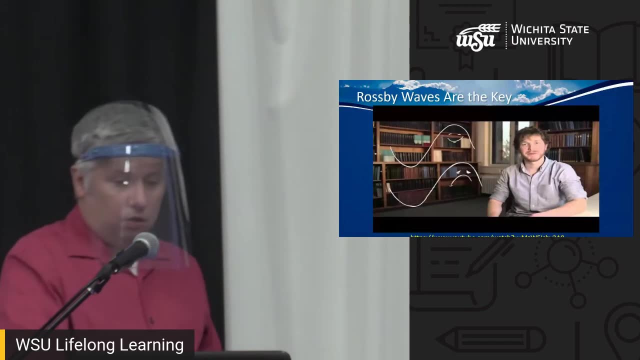 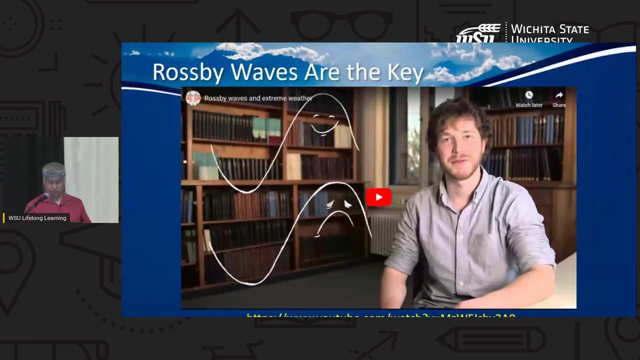 so let's dive a little bit deeper. oh, there we go. ah, i can get to the right slide. there we go. there's something called, and i think i may have actually brought this up a little bit earlier in the class- uh, not this class, but earlier in the the. uh, one of the early sessions these long. 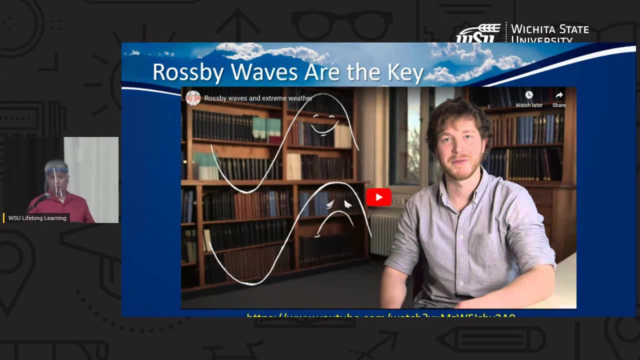 waves, uh, which are also called raspy waves. uh, this guy is, uh. he's got a pretty thick accent, um, and i'll try to reiterate a little bit uh, of what he's getting at here, but he also does it kind of graphically. so this is a really good uh discussion as to something that can start occurring. 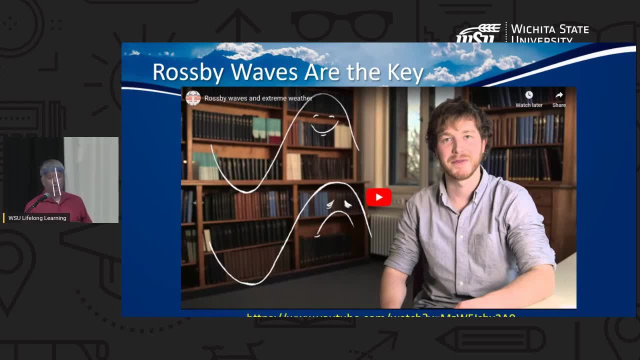 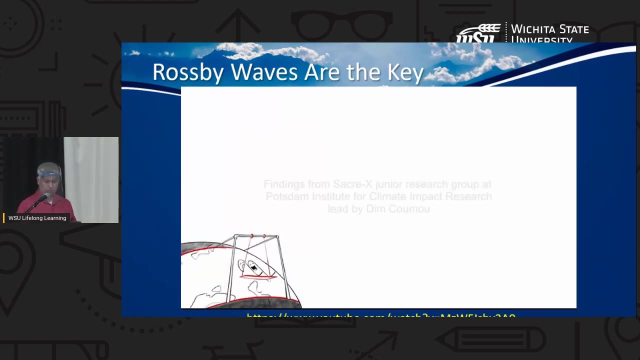 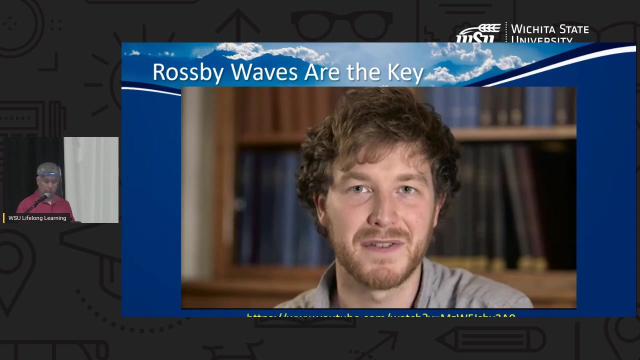 that helps us understand why, when you add heat into a system, you can get both hotter weather as well as colder weather. so let's take a look at the extreme weather in the northern hemisphere, such as the pakistani floods and the russian heat wave in 2010. 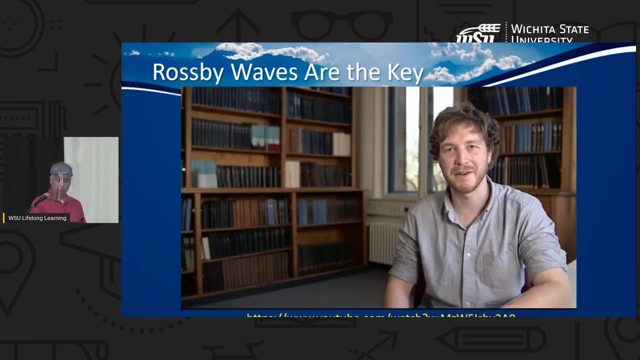 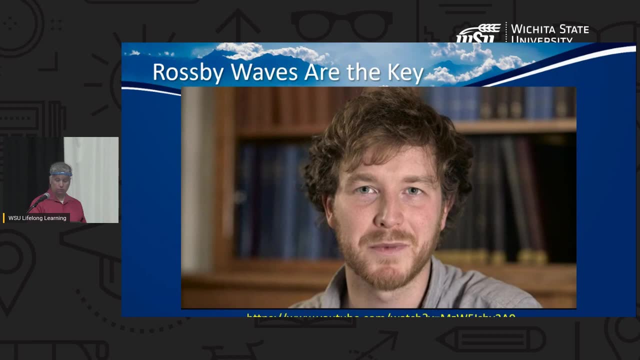 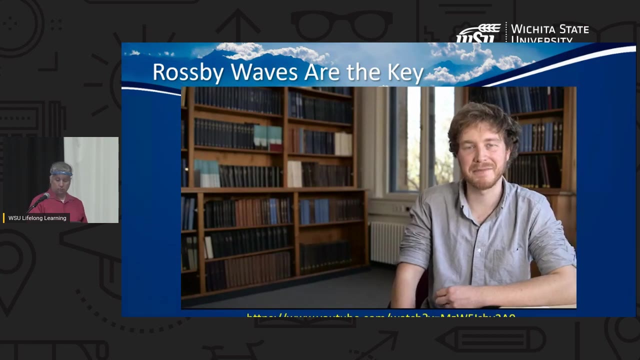 affect millions. since the turn of the century, the number of such extremes has greatly increased. part of this increase can be explained by simple thermodynamic arguments. if the world gets warmer, then more extreme rainfall and heat waves are to be expected. however, the magnitude and duration of some heat waves and floods that we 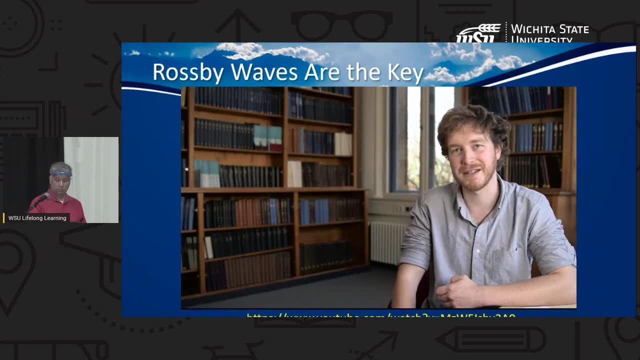 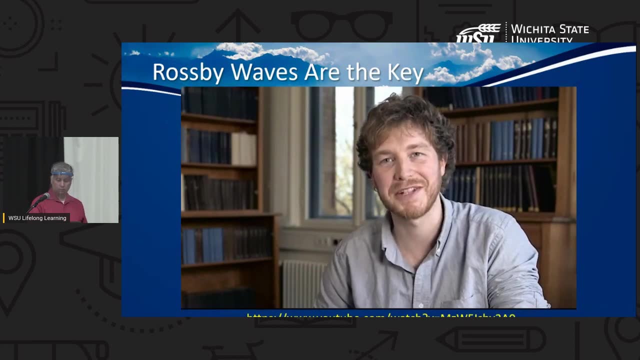 have seen in recent summers are disproportionate, and this puzzled us. vladimir petukhov then made a surprising observation: when searching the atmosphere for recent changes in circulation patterns, he saw quasi-stationary synoptic raspy waves with high amplitude during these extreme events that persisted in the northern hemisphere for a long period of time. in the northern hemisphere. 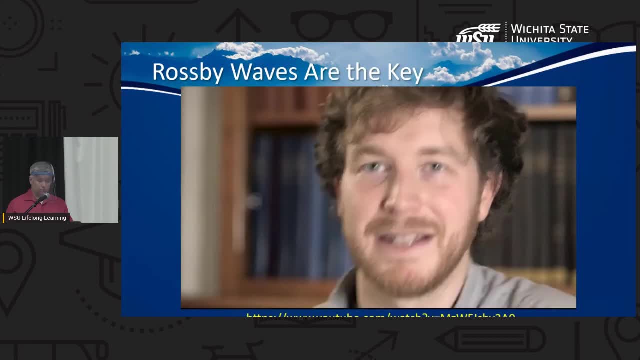 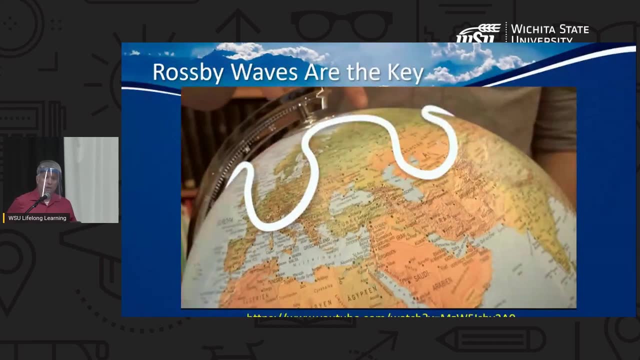 for weeks. let me explain. raspy waves are giant meanders in high altitude winds in the middle latitudes. you can think of those. when the winds of the west, they carry warm air from the tropics to the north, and when they swing down they carry cold air from the arctic to the south. some raspy waves are especially. 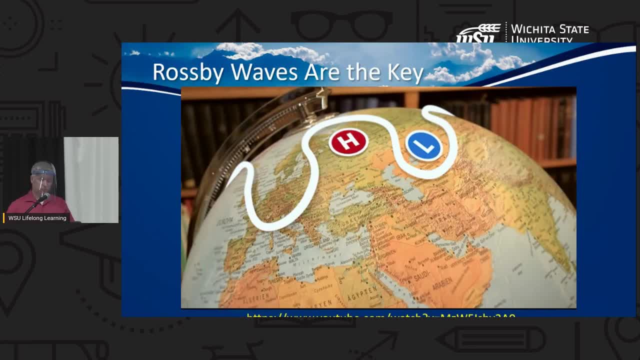 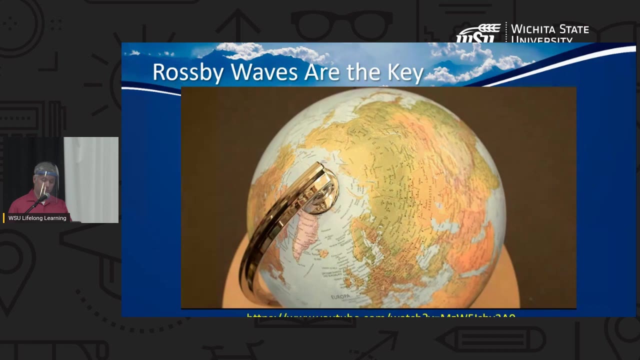 influential on our weather because they create the high and low pressure areas on the ground as seen on weather maps. raspy waves have a specific horizontal length scale of around a thousand kilometers and are called synoptic waves. their wave number is about six to eight, meaning that six to eight wave cycles. 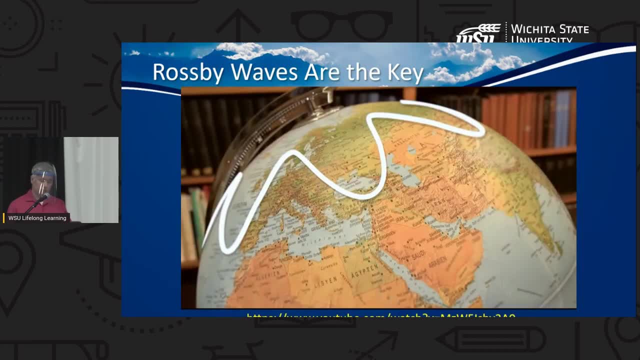 fit around the globe. normally, these waves move eastward, which means that weather systems move too. sometimes, however, that eastward movement slows down or even freezes. in this case, high and low pressure areas persist over specific regions, and that's why the waves move in different directions, and that's why the waves move in different directions. and that's why the waves move in different directions. 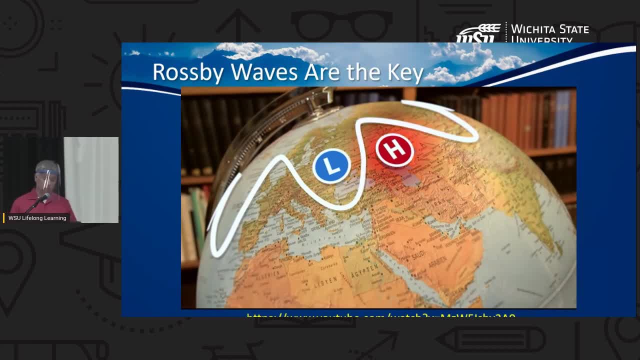 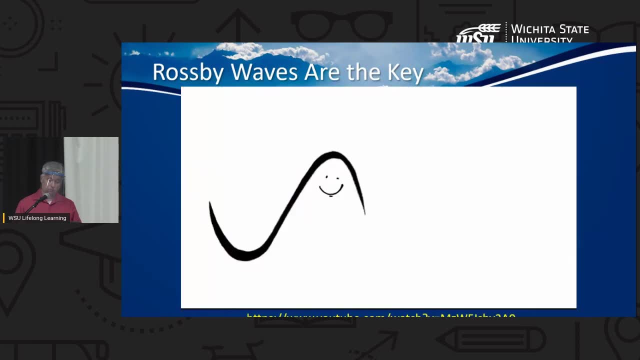 for longer than normal. That leads to extreme weather events. Raspberry waves can be decomposed into freely traveling waves and forced waves. Freely traveling synoptic waves normally move quickly. Consequently, their stationary components are small. Free waves would exist even if our planet had no surface structure. 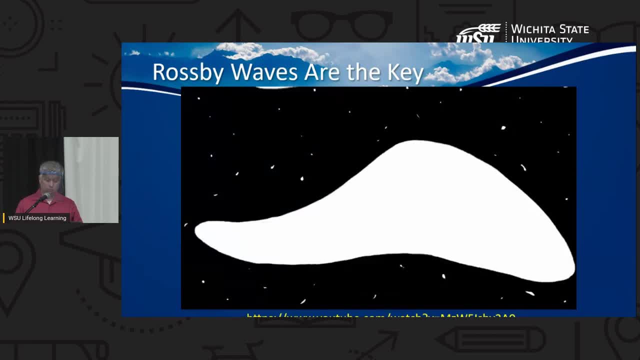 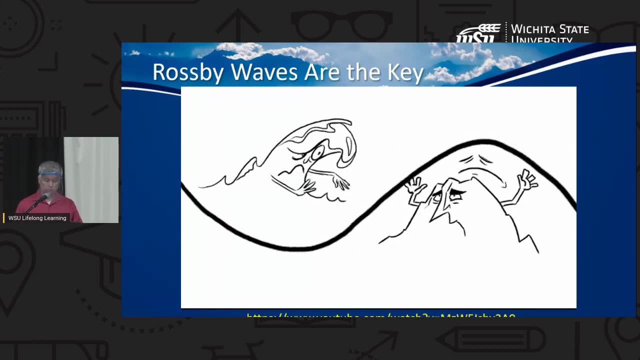 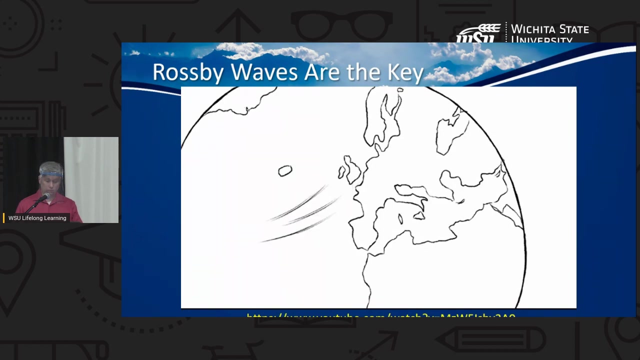 They form purely due to the instability of the atmosphere. The second component, on the other hand, is forced into its shape by high mountain ranges and temperature differences between oceans and continents. They are inherently mostly stationary and their synoptic components are weak. Under normal conditions, synoptic waves lose energy toward the poles and the equator. 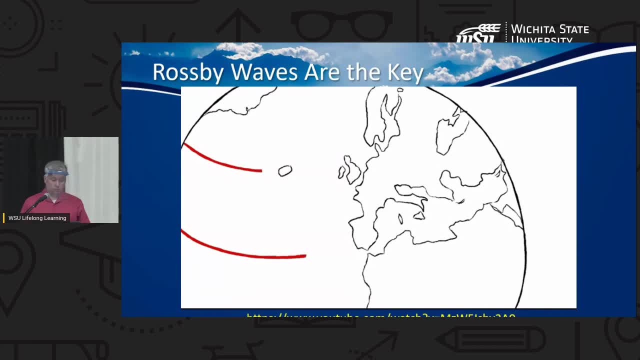 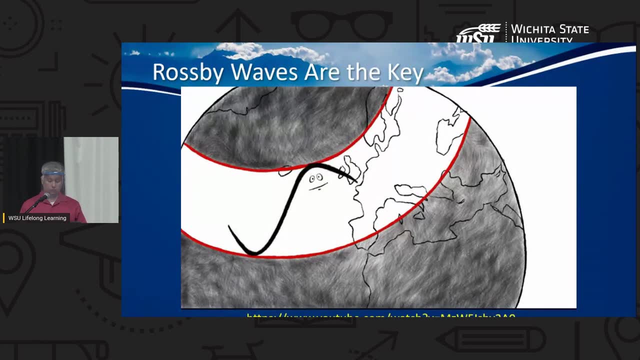 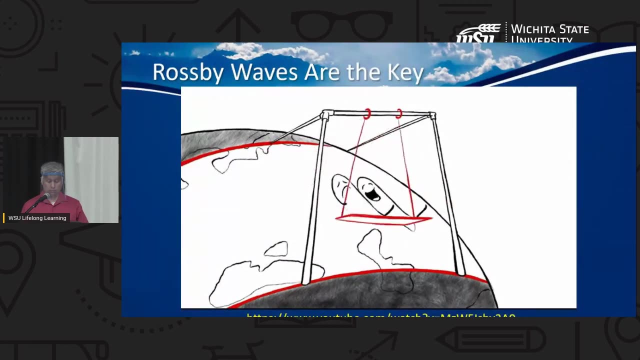 Under specific conditions, however, the averaged west-to-east wind forms a confining channel called a waveguide. The waveguide, on the other hand, is not always stable. The waveguide stops this energy loss. When the wave is trapped, the forced wave can resonate with the stationary components of the free wave. 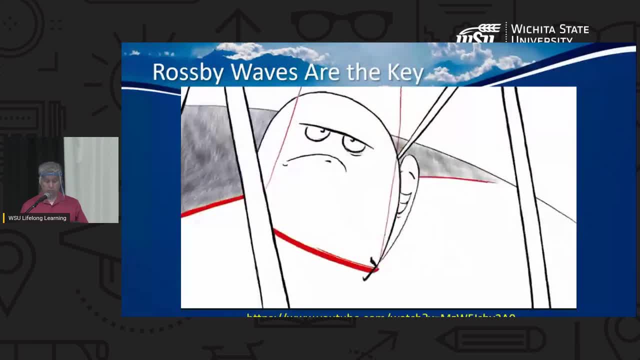 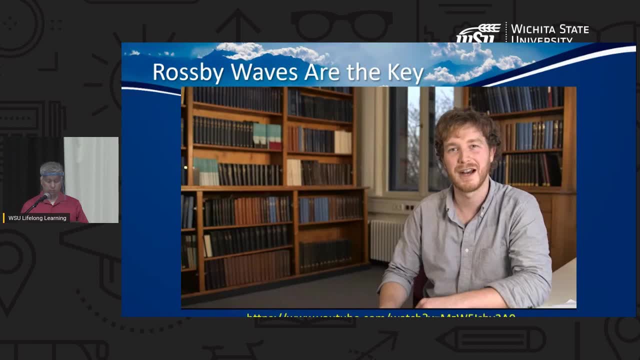 This greatly magnifies the amplitude Only if they have the same wave number. of course This is called wave resonance. As I said before, high amplitude quasi-stationary Rossby waves cause extreme surface weather. So this is an important mechanism and we have seen it more often in recent summers. 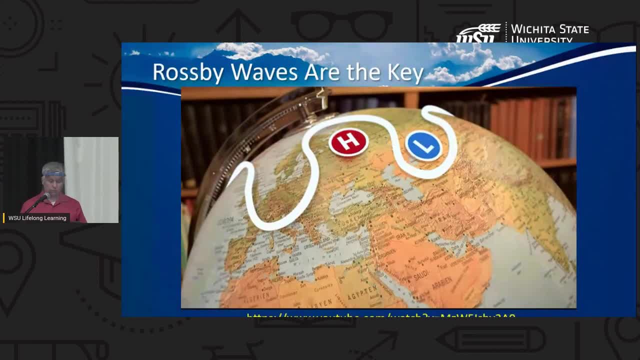 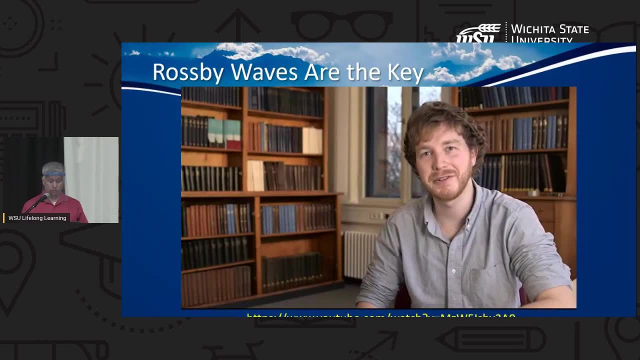 The Pakistani flood and the Russian heat waves, for instance, were caused by the same wave. The resonance mechanism shows how delicate the interlinkages are between the components in the Earth system and how little changes in the dynamics can have big impacts on extreme weather and the society. 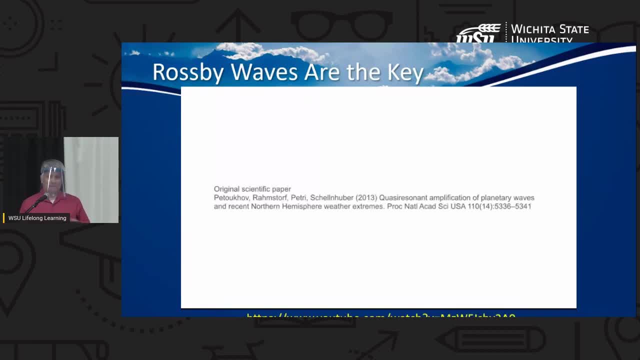 It's okay Thick accent and going fast on some stuff, So I'm going to dissect that a little bit. as to what he's getting at, You've got these, in short, the waves that are going across the globe. Those waves are the Rossby wave, in general, It isn't perfect, but if you're ever looking at a jet stream chart, your main jet stream as it goes up and dives down and goes up- that's your Rossby wave- is what's being referred to as That wave is how we basically mix and try to get the atmosphere back to an equilibrium point. Remember, the atmosphere wants to get everything to the same temperature. It's just like mixing hot and cold water in your bathtub. Eventually it's going to. if you add hot water out of the faucet into a cold tub, it's going to start heating right near where it goes in. 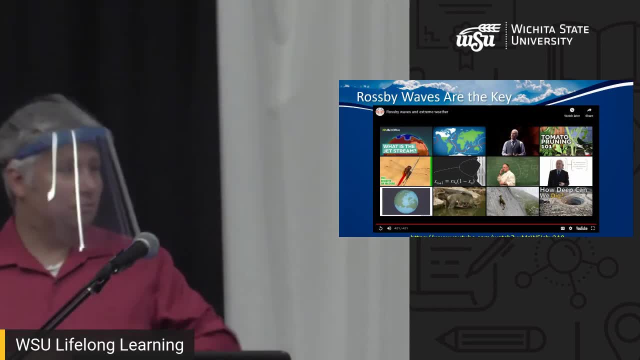 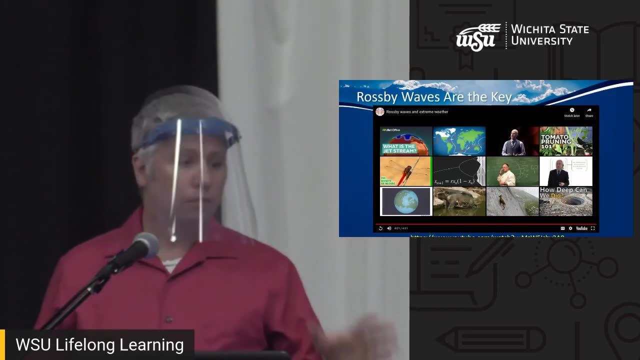 but ultimately the tub wants to mix it in and by the time everything's mixed across, it winds up all being about the same temperature, Same idea of what the Rossby waves are trying to do. But here's the thing, and this is something I don't know why it doesn't get. 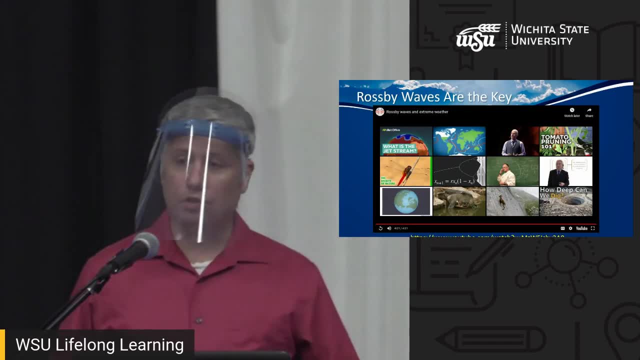 described in this sense nearly as much as it should. probably because of the people who are out there trying to push it one way or the other. Probably because of the people who are out there trying to push it one way or the other. Probably because of the people who are out there trying to push it one way or the other. 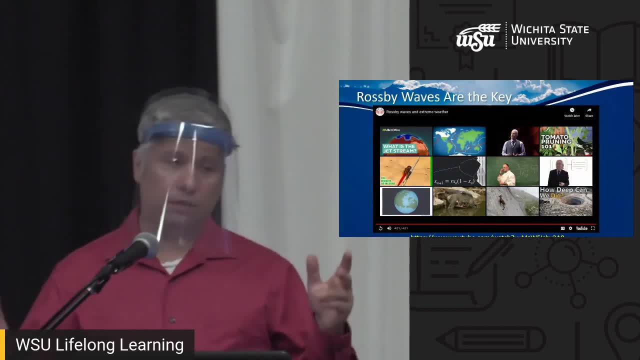 In terms of talking about climate change, because oftentimes it goes, oh yes, it's definitely happening and we need to do all these things. What's missing in all of that, in terms of trying to conceptualize the changing of climates, and is a climate warming when we're having snowstorms. Well, it can be, because the more heat that we are applying near the equator and the more heat that's getting trapped near the equator, the more the atmosphere is trying to horizontally- in this case not vertically- mix everything out and get everything back to an equilibrium. 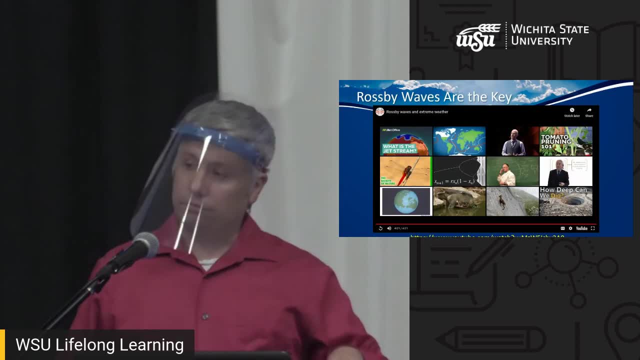 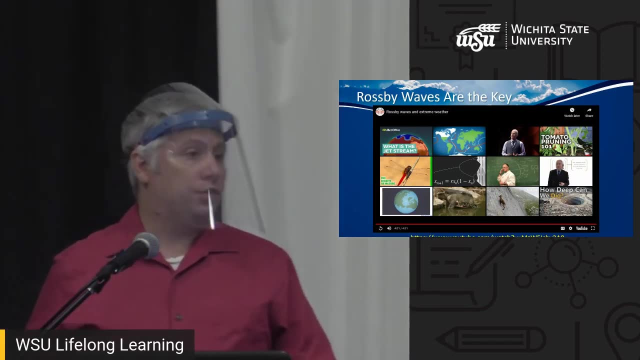 Well, if you've got more heat near the equator, that has to get mixed out. you need more extreme waves to mix those out And as those waves across the globe get larger, they start to move slower. A small wave is going to move around the world without stopping. But those big, massive waves of air pulling up warm air from the tropics and cold air from the Arctic. as you warm more at the equator, those waves naturally get larger because they're trying to do more to get the atmosphere back into balance. 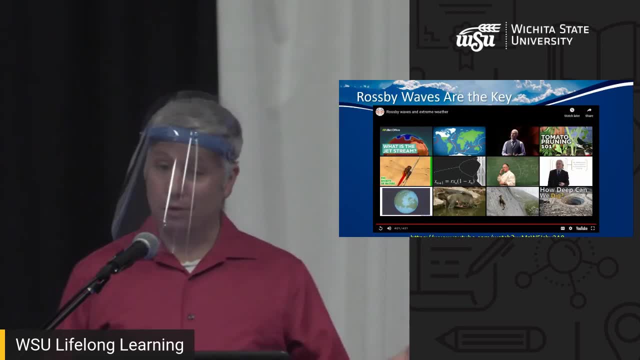 And so that I don't know why there are more people trying to explain it that way, but at least for me that's what you know if you're trying to conceptualize why I would have this massive snowstorm in an environment that is heating more. well, that is one such argument for why that would actually be the case, And that's also why yeah, okay, maybe you're cold in your location, but if you're really cold in your location, somebody else is real warm in another location. 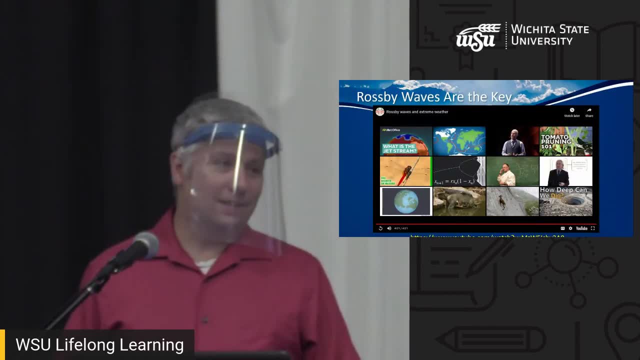 You know it's like I tell some people it. you know, the averages are born of the extremes And so, if you look, the average temperature doesn't move much, but boy, it feels like we're always having the extreme weather. 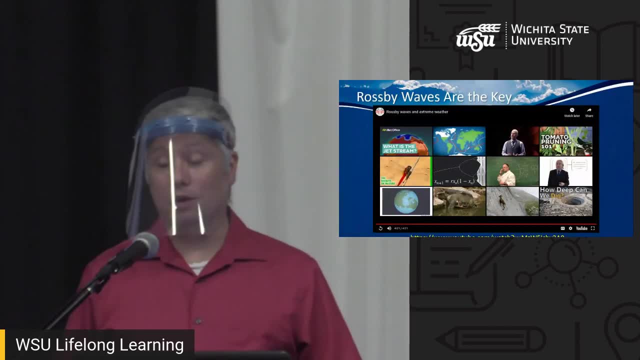 Well, there's always been extreme weather and there will always be extreme weather, But the fact that these Rossby waves are increasing, the fact that the oceans are getting warmer, do tend to lend themselves to a fact that there is additional heat in the atmosphere that is not getting back out. 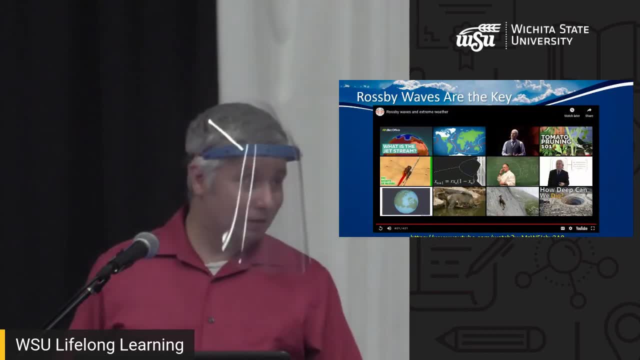 Now how much of that is a human fault and how much is natural occurrence. Well, that's why we have fights every two and four years between the Republicans and the Democrats in this country over climate change, because we really don't know, And we know that there's almost certainly some impact from humans. 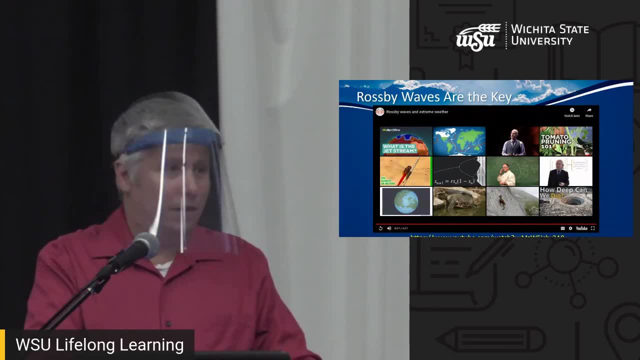 because anytime you have a variable in the system- and we are a variable in the atmospheric system as just in our existence- you're going to have some impact. We just don't fully know how big that impact is, But we also know that, as the world's population continues to increase, 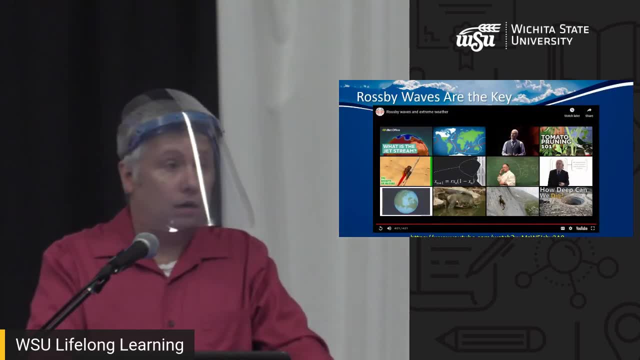 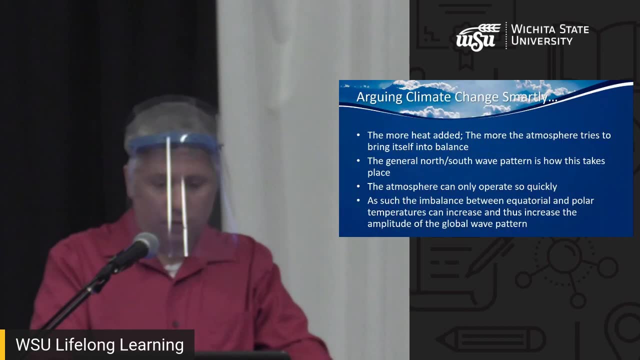 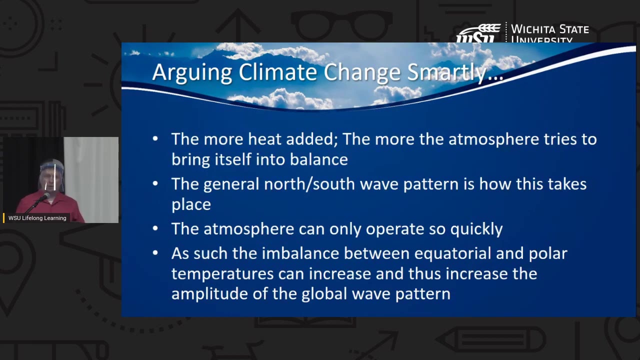 that input will also seemingly increase. So what's a good person to do in terms of trying to talk to other people about climate change and try to rationalize our own views on this issue? Well, there are definitely smart ways to argue both sides of climate change in terms of arguing for it. 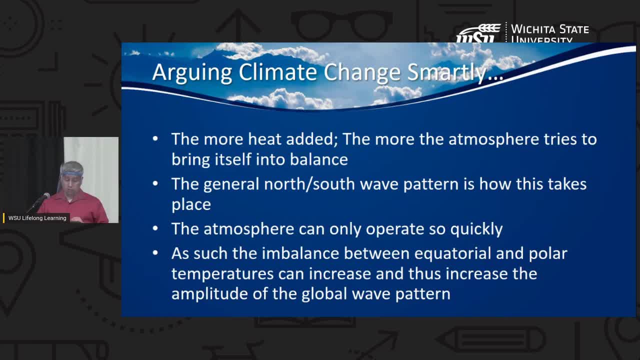 and that we're just huge contributors to what's going on. Well, naturally, you know, the more heat that gets added, whether that heat be from just our physical existence on the planet, the kicking out of planet Earth of pollutants from our vehicles. 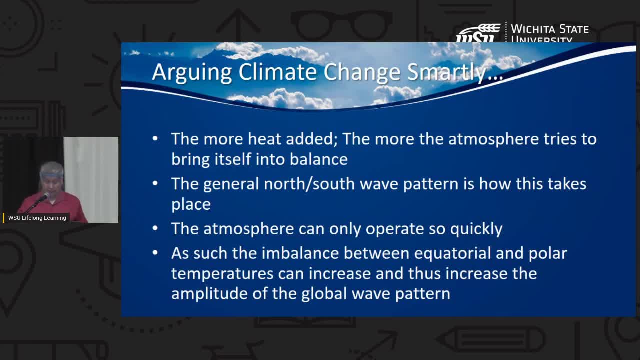 from our factories, things like that. all of these things are adding heat to the atmosphere, And the more heat that we add, the more the atmosphere tries to bring itself into a sense of balance. And the more heat we add, the harder it has to work to try to bring us into balance. 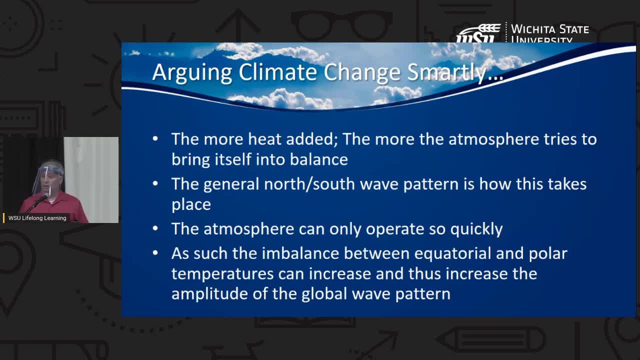 And hence, as I just mentioned, the more likely you're going to get those slower, higher amplitude Rossby waves setting up across the Northern Hemisphere- And this also happens in the Southern Hemisphere as well- And so the atmosphere, in terms of trying to bring itself into balance. 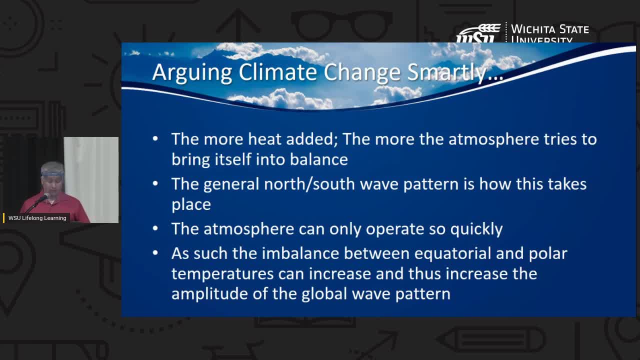 it's only able to operate so quickly, And so that imbalance between the equator and the poles can increase, And as it increases, things get more extreme and more extreme and more extreme. At least, that's the argument that is made on this. 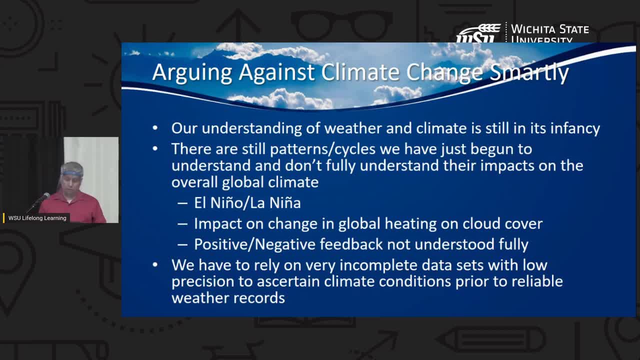 So let's flip it around and talk about the other side arguing against the climate change smartly. Our understanding, as I've tried to spell out over the course of the last four weeks that we've been together- our understanding of atmospheric change. 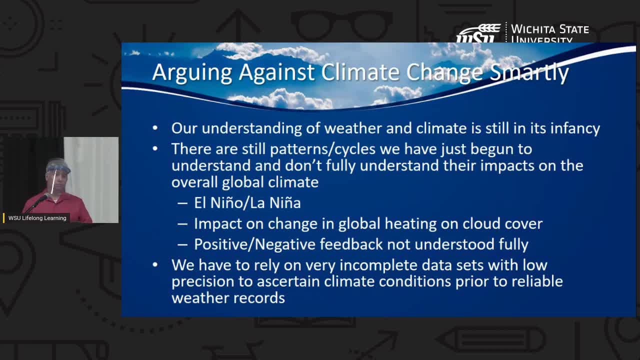 of what's really going on around us really, in a lot of respects of physical sciences in general, is truly in its infancy. We are living in probably the most amazing time to be alive. We're making new discoveries, New technology is being developed on a yearly basis. 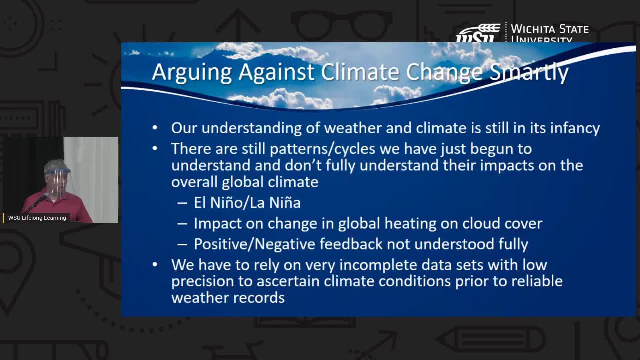 even less than that. sometimes, Even during a coronavirus outbreak. we're still pushing forward, Learning new things and inventing new things, growing in our understanding. That's probably only going to get faster as we continue to move forward, And so we are learning. 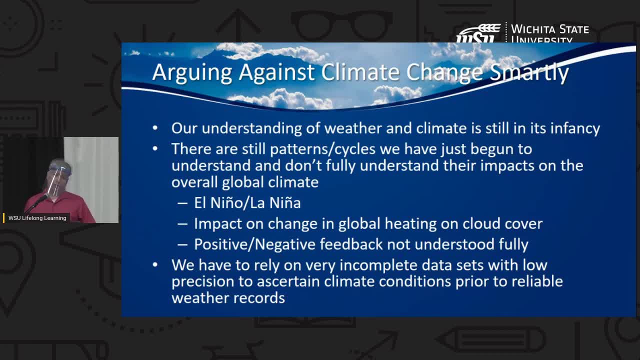 yes, but we have a lot to learn. There's a lot of cycles and patterns that we simply don't understand Because we haven't discovered them yet. We've got huge influencers on the weather from the oceans that we've only discovered in the last 50 years. 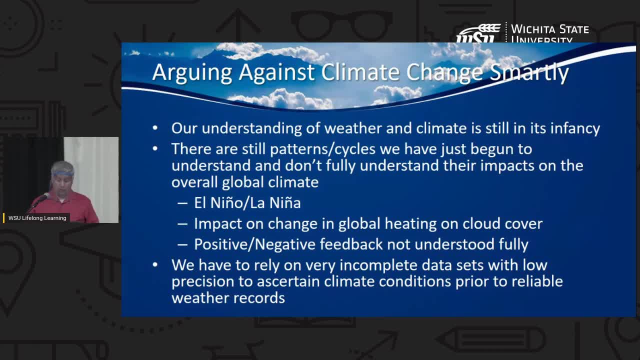 El Niño, La Niña. I talked about that earlier. We have no idea what the impact on any changes in terms of global heating have on actual cloud cover. There's talk of, oh well, all of these icebergs will melt. 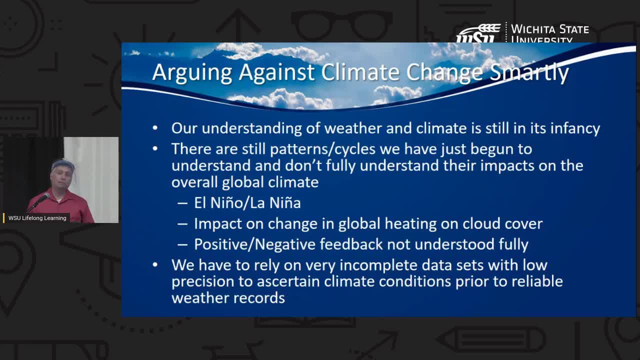 and then the oceans will rise and everything like that. But there's an offsetting element there, because as the atmosphere warms, remember- the atmosphere can hold more moisture. So there is an offset of the atmosphere getting warmer and then evaporating more into the atmosphere. 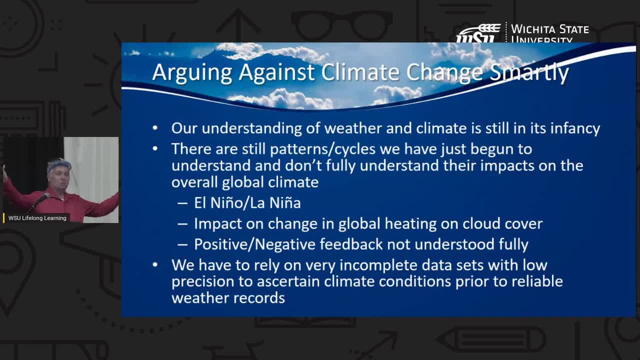 And if it evaporates more into the atmosphere, eventually what goes up must come down, And so that is another mechanism that the atmosphere is using to help bring itself into balance, to help cool things down that we still don't totally. I mean, we know about the hydrologic cycle and things like that. 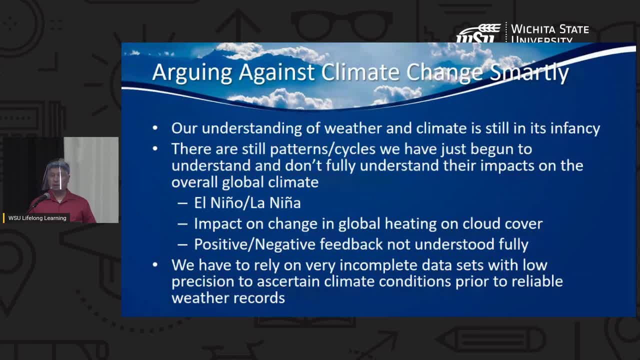 but how heating or cooling impacts that hydrologic cycle and the amount of moisture that's actually trapped in our atmosphere. we're not sure. Our number one contributor, by the way, in terms of being a greenhouse gas, is not CO2.. It's not even chlorofluorocarbons. 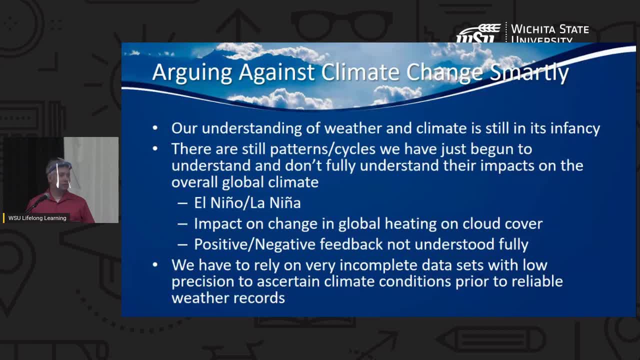 It's water vapor which naturally occurs in the atmosphere. So as the atmosphere warms and we get more water vapor in the atmosphere, well then you also get more warming, But at some point that water comes back out of the atmosphere and balances itself out. 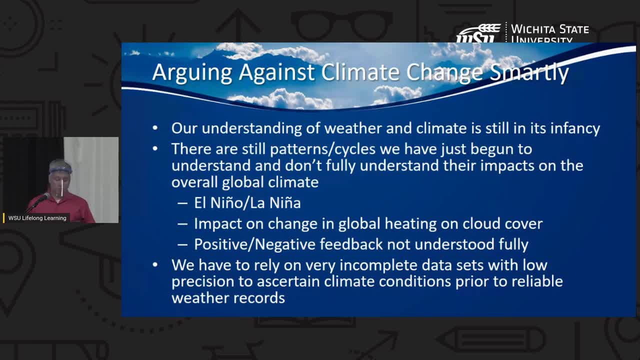 We don't know exactly how that works itself out. We also don't know about these positive and negative feedbacks. Positive feedback would be a feedback that would enhance the effects of climate change, in particular the warming aspect of climate change, versus negative feedback would not. 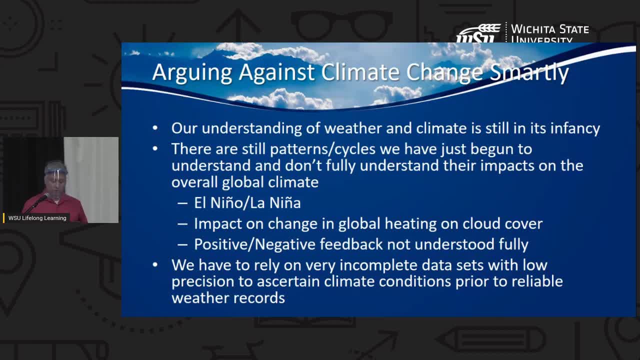 would negate the warming that would occur, And there's still a lot of inputs that we don't fully understand. We also have to rely on very incomplete data sets- as we've talked about throughout the course- with pretty low precision to ascertain what the climate conditions were prior to our reliable weather records. 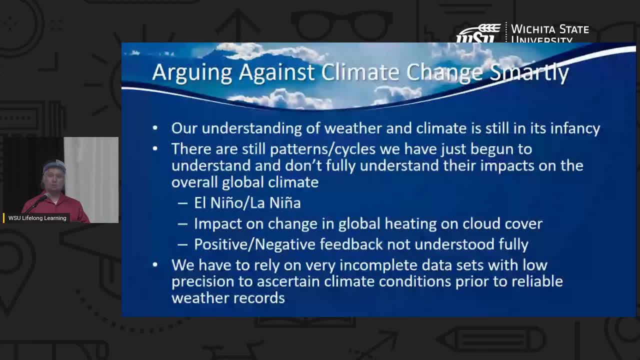 I mean even when you're looking. remember, when we're talking about ice cores, there's only certain parts of the globe that you can get an ice core, So you're not you know when you're looking back and you're trying to get that data. 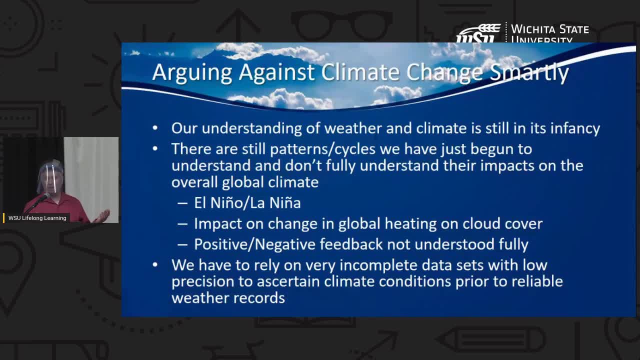 you're only getting a couple of points across the entire planet When you're finding fossil records. well, we don't get those all the time. We do have some pretty good dating mechanics on that carbon dating on those fossils And you know that can give us some understanding. 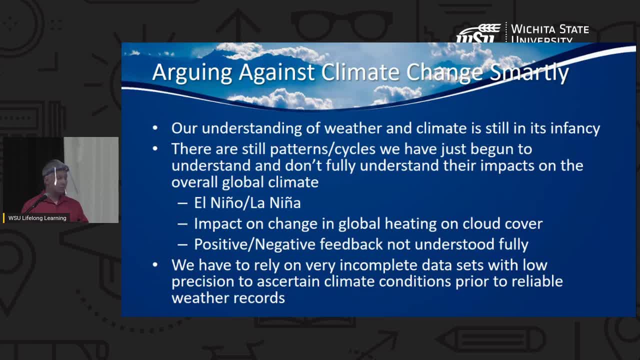 but it's pretty general information, to be honest, And so there is a lot that we've ascertained about our climate over time in general. But again it comes back to if we didn't have our nice fancy instrumentation in the ground. 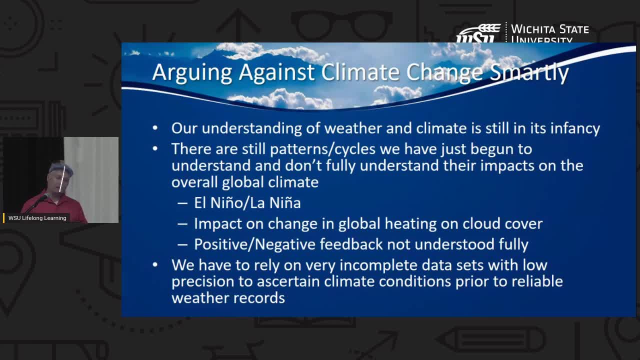 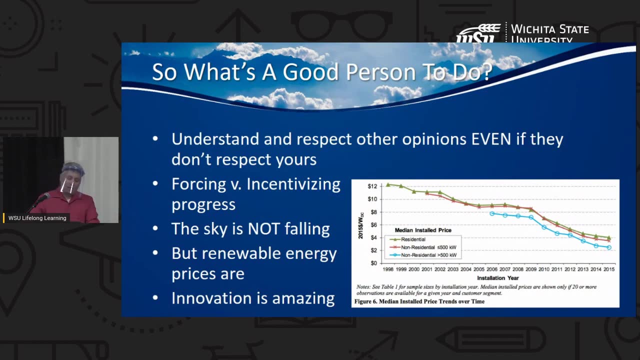 how do we really know what the weather was like back 1,000 years, 1,500 years further back than that? We may not. So what's a good person to do? Hopefully, we're all good people in this room. Here's my take on it. 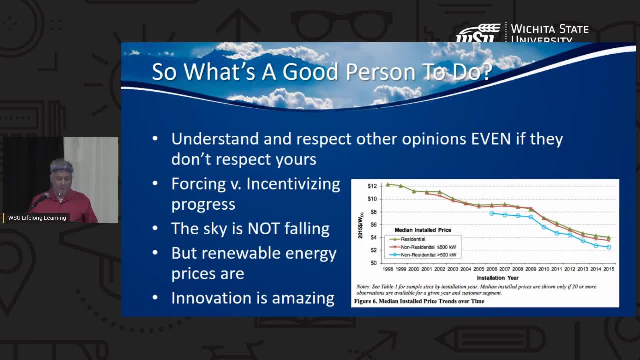 You can agree with it. You can disagree with it. You know it's important that we in this whole. you know there's so much yelling back and forth that happens on global warming and climate change. Oh my God, we're ruining the planet. 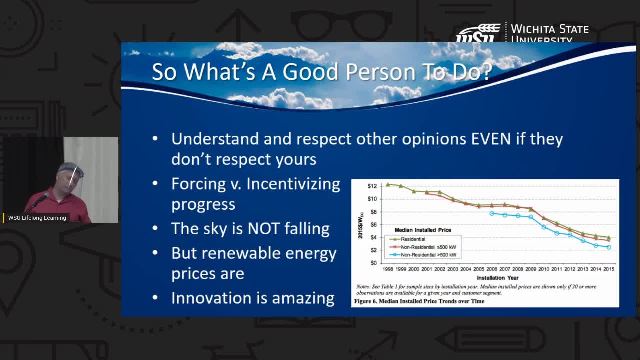 We've got to shut everything down? Oh no, we're going to ruin the economy. We've got to, you know, push, push, push on innovation. The reality is there's no right or wrong extreme there. We have to continue to move innovation forward. 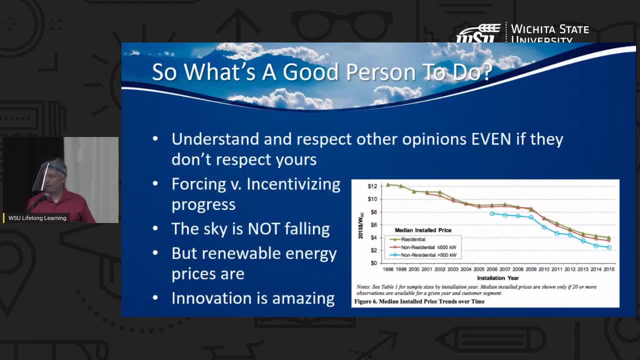 If we don't move innovation forward, well, guess what? We're not going to come up with the technologies that we need to combat real issues of changing climate, things of that nature. We've got to protect and help companies innovate. We should never be stifling that. 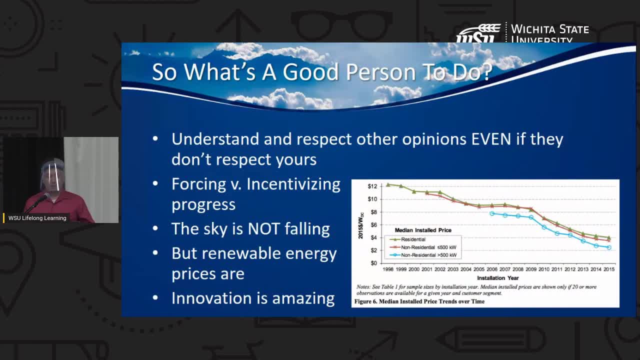 And you know whether government is the best source to do that, whether it's the private sector, well, that gets above my pay grade, but it's probably a combination. I think either extreme is probably too extreme. So there's a lot of talk about you know, either you know forcing people. 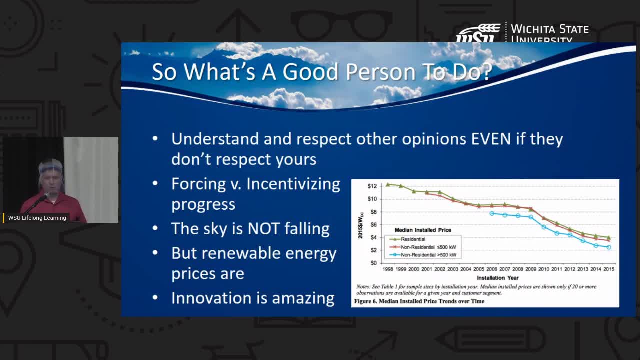 especially with some of this Green New Deal proposals out there, kind of pushing people. It's kind of forcing the hand of us and causing us to have to change the way we live and change the way our industries work versus incentivizing progress. You know that's the other extreme. 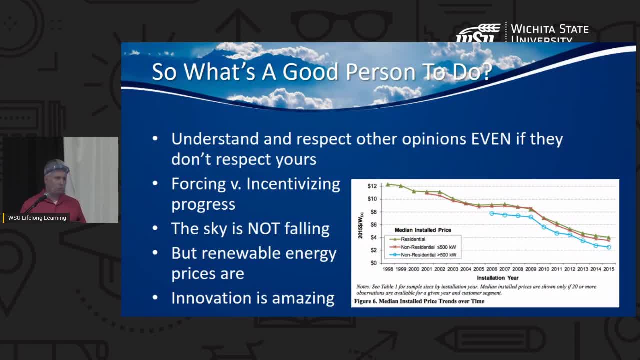 One of the things that I love kind of watching is it's been a little while since I've paid attention to too much of what they do. You've got the X project, the X Prize- Excuse me, That's out there- And the X Prize started first with trying to get the first private group. 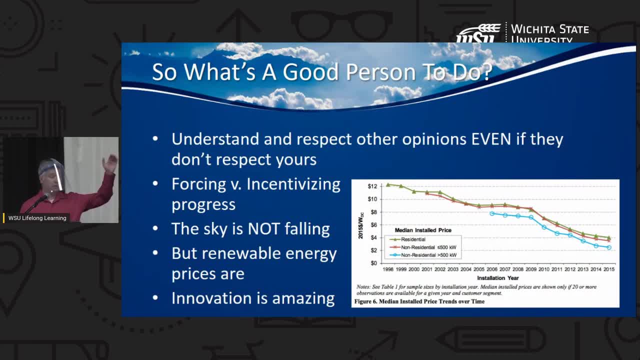 to get a you know shuttle into sub-orbit, And that was a privately funded prize that eventually led to some of the developments that we have in Virgin Galactic. Elon Musk's- yeah, thank you, SpaceX. I watch them all the time blanking up here. 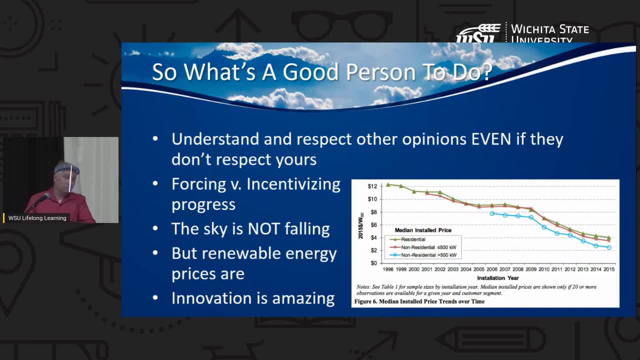 You know, and some of these other innovations that were actually born out of the private sector and you know, educational and even some government agencies coming together, all contributing to something that you won if you completed a task faster than anyone else. I kind of like that idea personally. 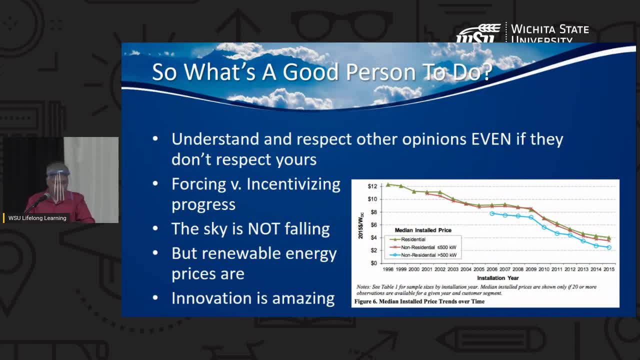 That's just my opinion. I think this third point is really important. You know, when we watch the news, when we watch the talking heads, you know, I don't care if you're watching something that's decidedly biased right or biased to left- the sky is always falling. 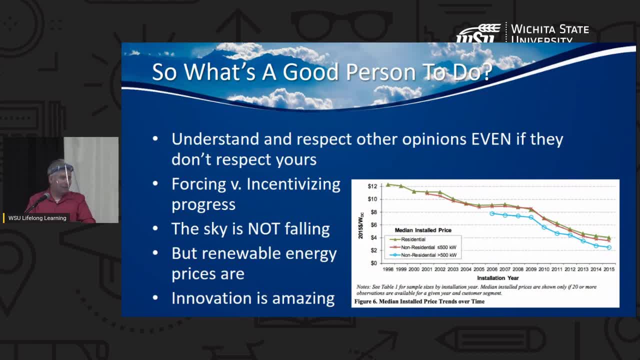 We're going to hear that for the next two months. you know that everything is falling apart. The sky is not falling. Let me repeat that: The sky is not falling, Chicken Little. The things that are going on are going on over long periods of time. 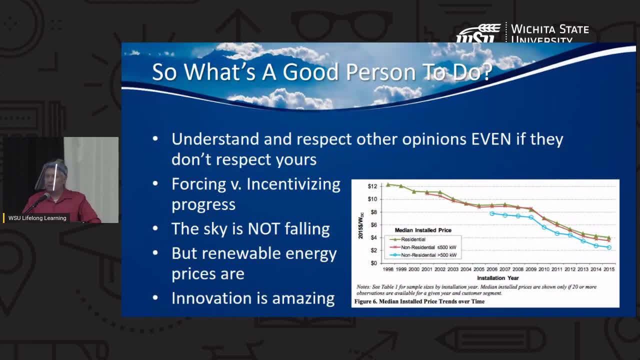 If we are warming the planet drastically- and it is humans that is the main contributor- I can virtually guarantee that by the end of the century we are not going to ruin the planet, Because we are. we can only do so much. The atmosphere has an amazing innate ability to correct itself. 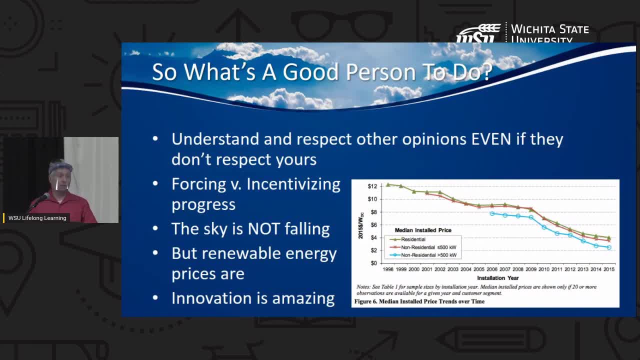 Now, some of that correction is violent. Some of that correction is heat waves, cold periods, But it is far more powerful than we are, And to think otherwise is probably a little bit arrogant on our part. The good news is, though, our ways of mitigating the atmosphere. 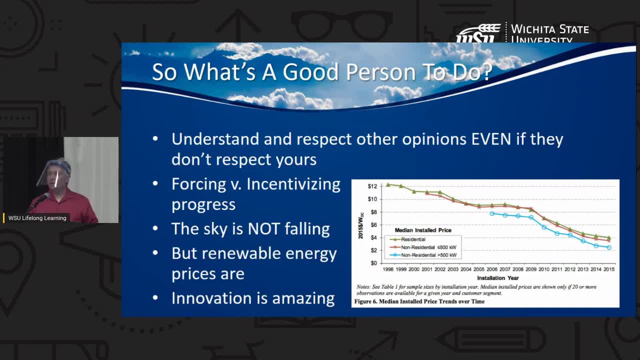 of recapturing carbon dioxide and other pollutants in the atmosphere is getting better. Our technologies as they relate to renewable energy- whether that be solar or wind and hydrologic, many others- is becoming less and less expensive. It is a supply-demand curve. 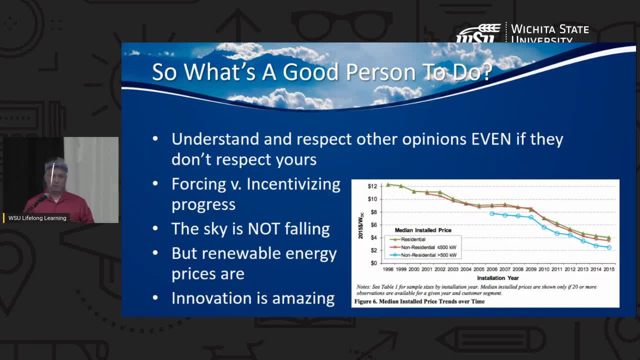 Once you start producing more, the prices start coming down And our ability to produce energy that is renewable at cheaper and cheaper prices. it is getting better and better. And it is getting better and better fairly quickly, And that did require, in some cases, some incentives from government or other institutions. 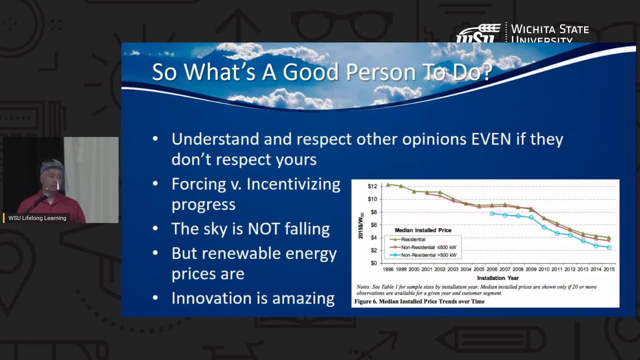 But the need for some of those incentives is decreasing because the technology in these areas are getting better. So really, what we want to do is continue to monitor, continue to innovate, continue to support the next generation and the things that they are able to come up with the best that we can. 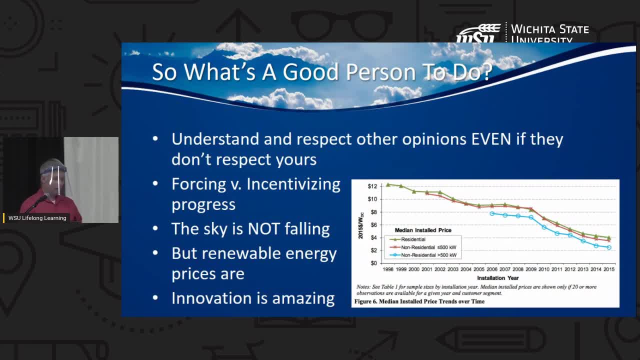 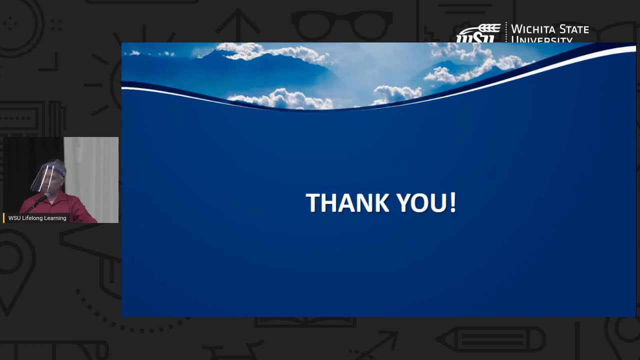 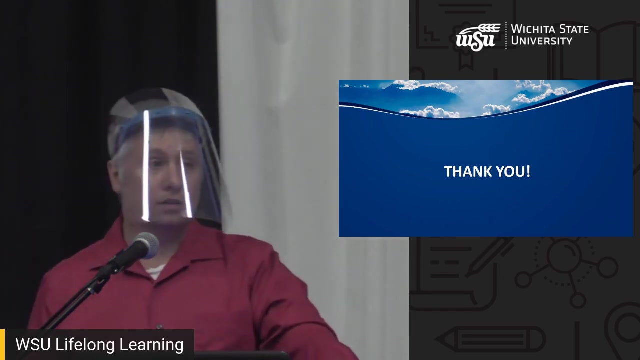 And I think that the dire outcomes are just going to be fantasies that are put into movies. So with that I am pretty much done and open to questions over the course of the rest of the class. We are done a little bit early, But I would be happy to stick around and talk to any of you. 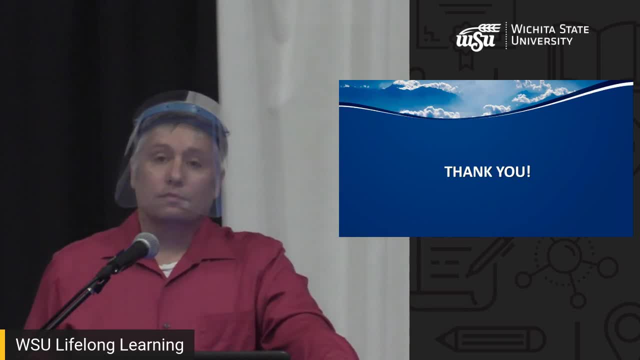 Yes, I missed the first class. Has there been discussion about how the moon impacts the weather? You know the moon has a lot more of an impact on the tides. There isn't as much impact on the weather by movement of the moon. Where you do run into the moon impacting the weather. that can definitely be a case with hurricanes, Because, depending on where your tide is, including you know, because the tide you know you've got your tide cycles and sometimes they're higher tides. 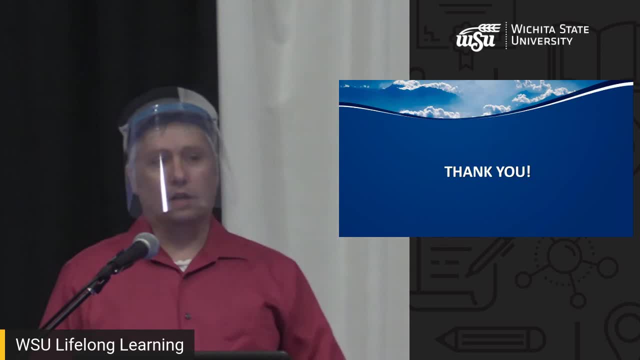 and sometimes they're not as high, of high tides, And I don't know exactly how they calculate all of the tides, All of the tidal cycles. I'm not as knowledgeable in that area, But there's definitely an examination as hurricanes come in. 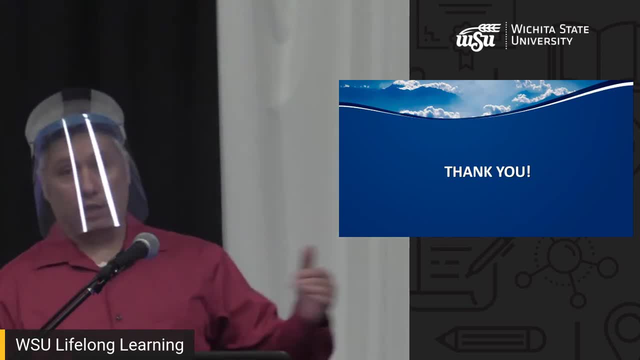 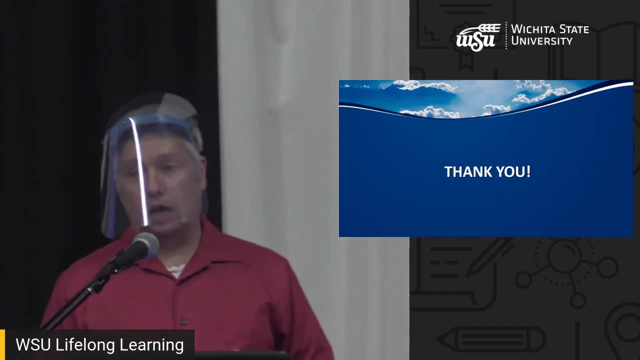 to determine how you know is it coming in on a high tide or a low tide, Because if the eyewall is coming on and when the eyewall comes on, you know pretty much right ahead of the eyewall. that you've got your storm surge, that comes in as well. Well, if that storm surge is being enhanced by a high tide, you know that can lead to your storm surge being several feet higher than it would normally be, And so that's the main area in which we generally look at the moon. 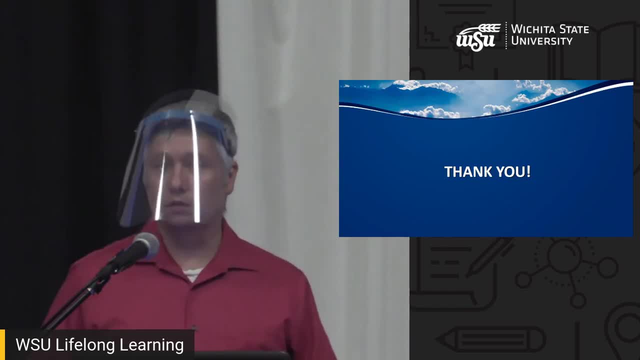 in terms of its influence on the weather, really with the tides? Other questions: Yeah, Pretty much, Yeah. I mean there can be escape of moisture from the atmosphere, but that is very limited. The nice thing is we have an atmosphere that is built in such a way. 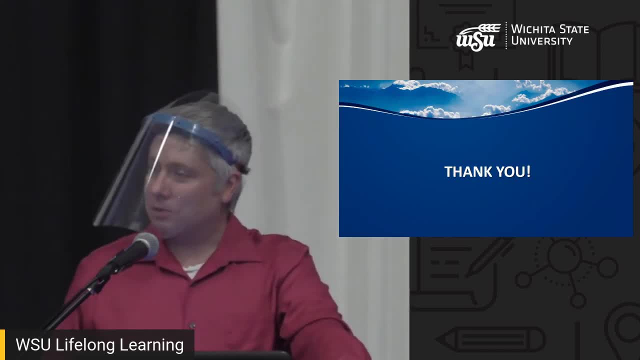 that it discourages the departure of moisture from it. you know, because everything that we have here in this lowest level of the atmosphere- I'll try to keep from walking back and forth- all the things that we have in this lowest level of our atmosphere. the troposphere. as moisture is pushed up and just atmosphere in general pushed up, it hits what's called the tropopause. Now, the tropopause what it really is is a significant temperature inversion And where we have temperatures dropping really rapidly. 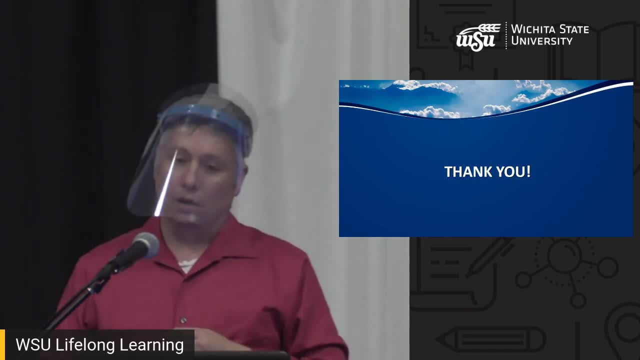 as happens above the tropopause. you are well, for a period of time above the tropopause, to be more exact, you have kind of a cap on anything moving higher. So the atmosphere and the moisture and everything that we have down in the troposphere. 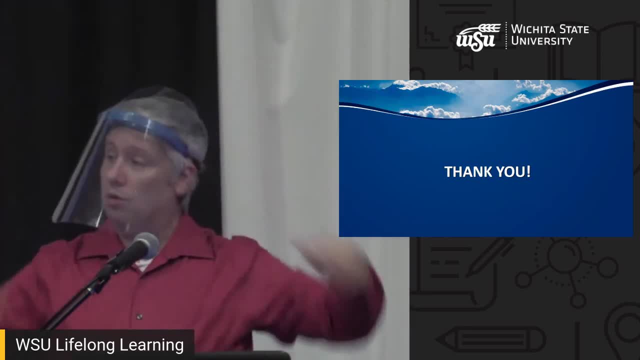 is inhibited from really getting beyond the troposphere. So the moisture that's here is the moisture that's here. Now, you know, you've got all of us take up some moisture. The oceans have moisture, The atmosphere has moisture, It's all around us. 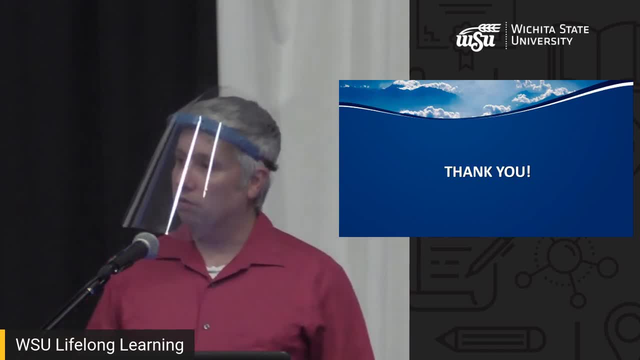 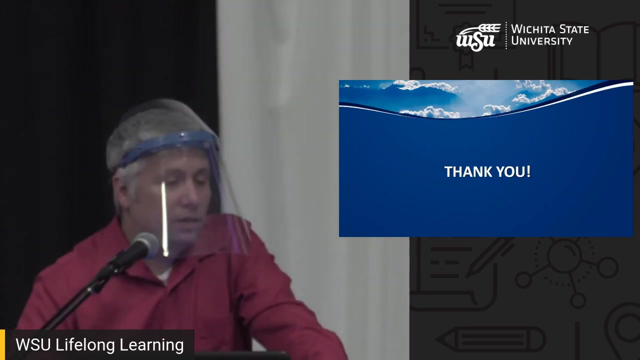 But it is a net neutral as a whole. Yes, And it just occurred to me. I haven't been repeating questions, so sorry. What was the question again? Do we have enough data? The question was: do we have enough data to determine? 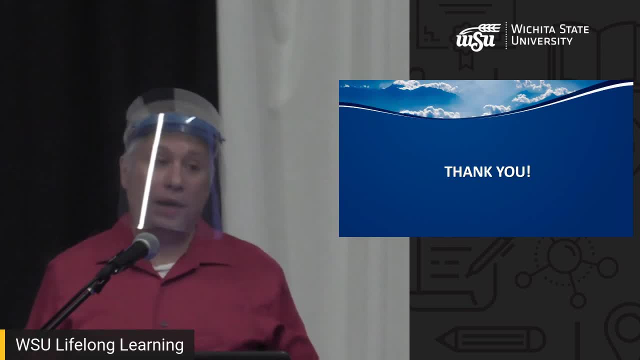 if climate change has had an impact on the number of tornadoes, I think on a large scale, it's hard to say that we do. Now. there is, you know, we got into this a little bit- There has been, you know, significant observation. 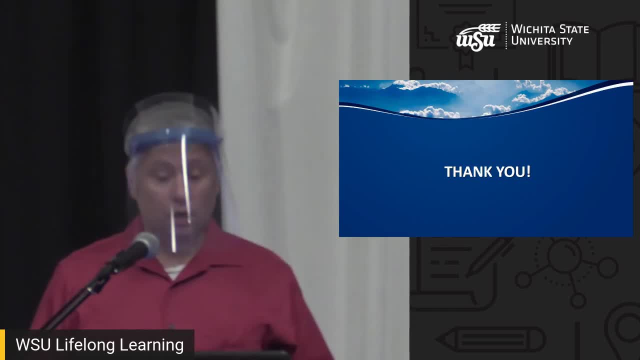 especially over the last probably about 15 years or so, across the plains It's been really really quiet seemingly- And actually not just seemingly, It's the number- the tornadic activity across the central plains has been down a lot. Now what we don't know is: is this actually related to climate change? 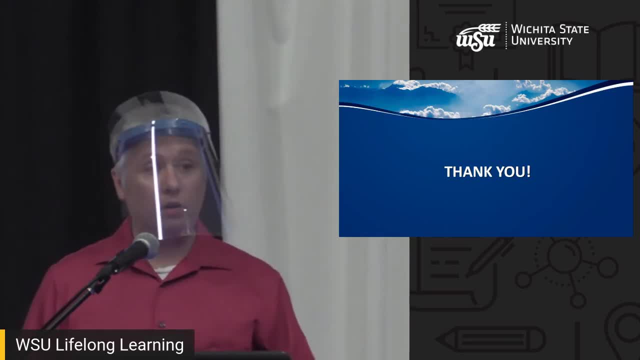 or is it a natural? you know cycle that we've got going on. Time will wind up telling if in another 10,, 20 years things pick up and we've got tornadoes all over the place again. But you know, it's definitely a quieter period in this part of the country. 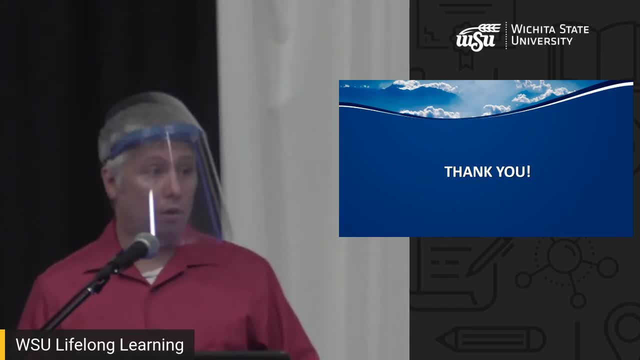 Now it's heated up more in the southeast. You know there's been a lot of very notable tornado outbreaks over the last 20 years across Tennessee, Tennessee, Kentucky, you know points a little bit further south. That's where a lot of the activity has been occurring. 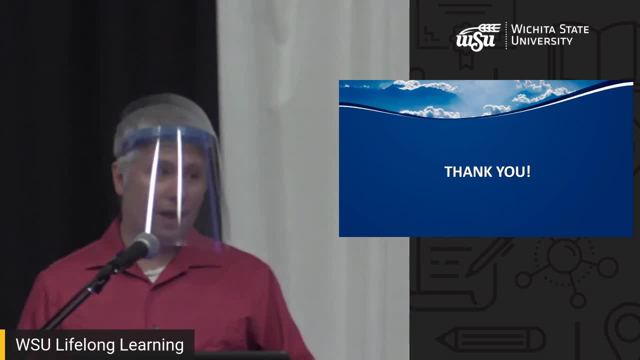 But the traditional areas of Tornado Alley. well, you know you're still getting tornadoes in Oklahoma, Our center points it's. you're not seeing, or at least we haven't seen, the significance in tornado outbreaks across this part of the knock on wood, across this part of the country. 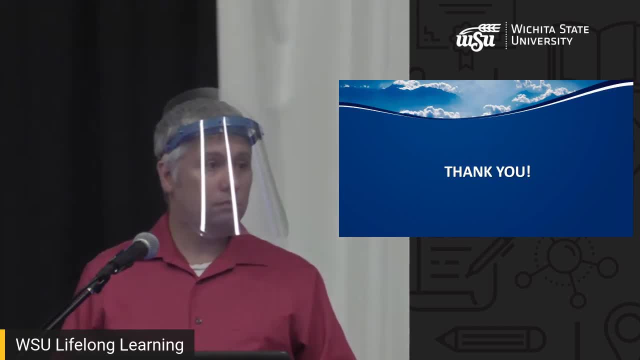 as maybe we have in previous decades, Hurricanes. you know that jury is still out as well. I mean some of this big talk about you know what's going on. you know some of this big talk about climate change and everything like that. 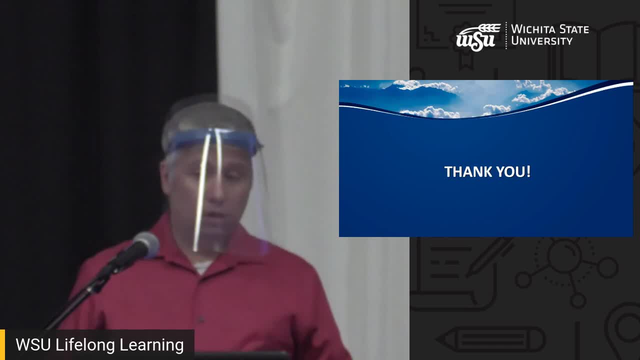 especially all of the oh my God, we've got to do stuff now came right after Katrina. You know that's when everybody started waking up and because that was a very that year and then the year following it were very, very active hurricane seasons. 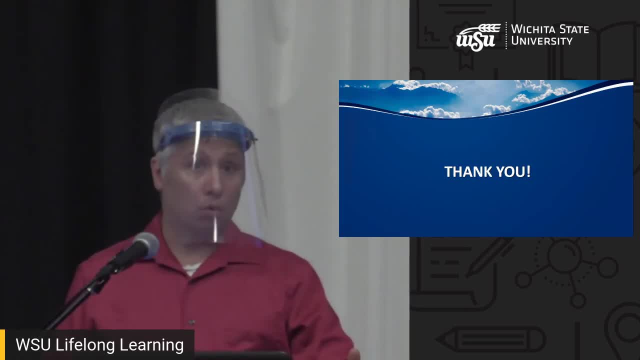 And actually it was the year after Katrina that was even more active. That was the season that you know. we actually got entirely through the alphabet and, I think, two or three named storms into beyond the alphabet in terms of named storms for the Atlantic. 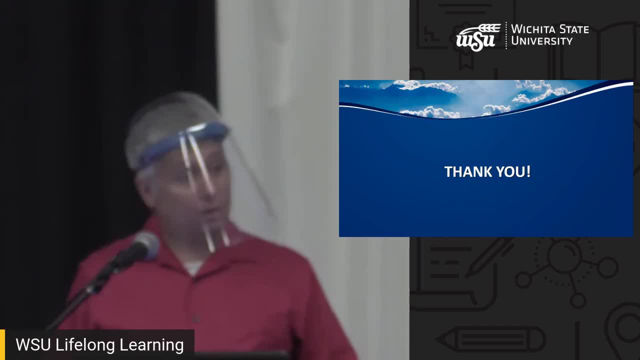 But again we've quieted off quite a bit there too. I mean, we've got two storms right now that have been coming through, But as a general whole, several of the last handful of years have been has certainly not been like those. 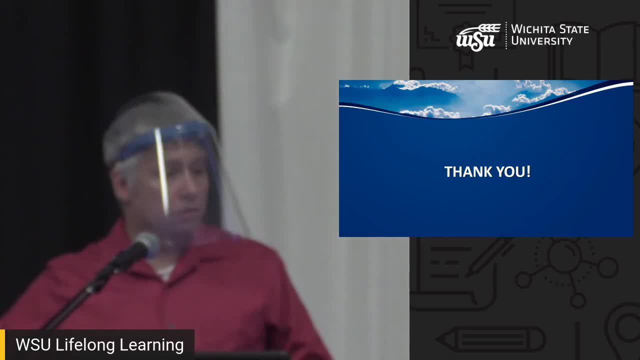 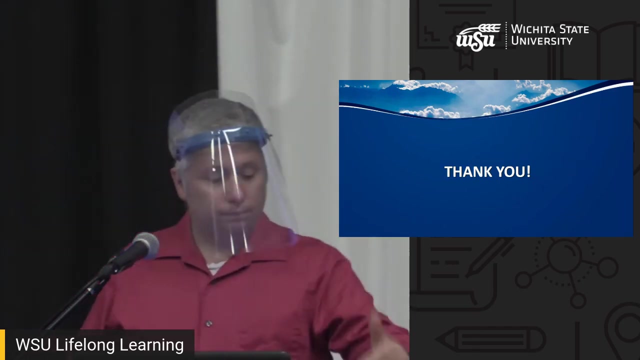 years in the 2000s, where we had a couple of really, really active years. So I don't know that there's really anything that can truly be determined from that. Now, if we follow the logic of the, you know, increased heating. heating the oceans. first, you get the oceans up to a certain threshold, which generally is about 80 degrees surface temperature. That is starting. you know. that's the point at which you're going to start fueling hurricanes in the right part of the oceans, that is. I mean you're not going to get a hurricane too far north of the equator, at least initializing. So as you increase that surface temperature you may not actually really be increasing the number of, but you certainly would increase the likelihood that they would become more significant storms. 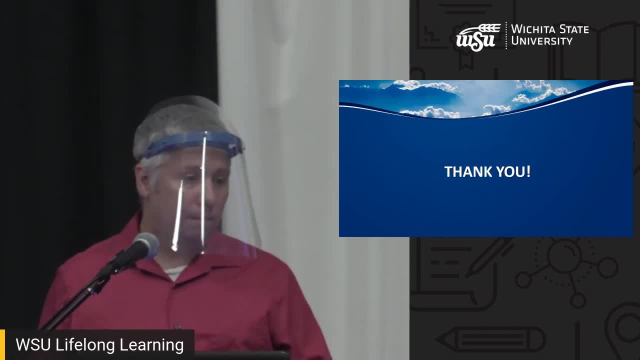 And that's the thing that has, you know, your hurricane meteorologists the most concerned is: are we going to get maybe not more storms, but the ones that we get are going to be stronger storms, And you know that's just something that we're going to have to continue to watch. But then you get the setup where you've got kind of a sister storms almost, And as a result, you know they're both, you know, popping up, But you know I mean they're not both monster. you know category five hurricanes either. 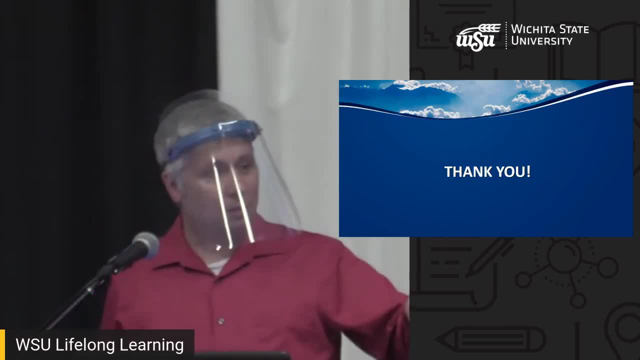 So do you wind up getting a lot of storms that are weaker, or do you get fewer storms that are really strong? We don't know. So I mean I wish I could give you guys great answers and be the smartest person ever. 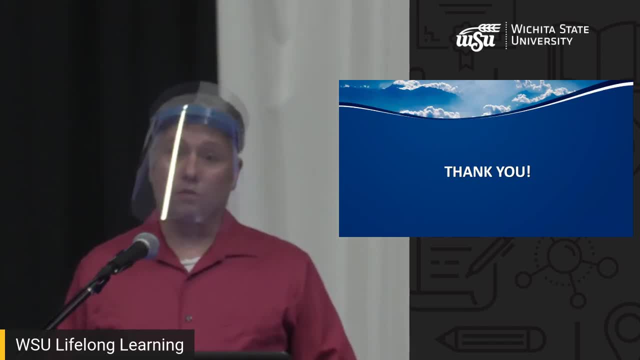 But it is a young science And there just is so much that we are studying actively but we just don't have a true answer that I can just hand out and end all of the constant political debating over global warming and climate change and all of this. 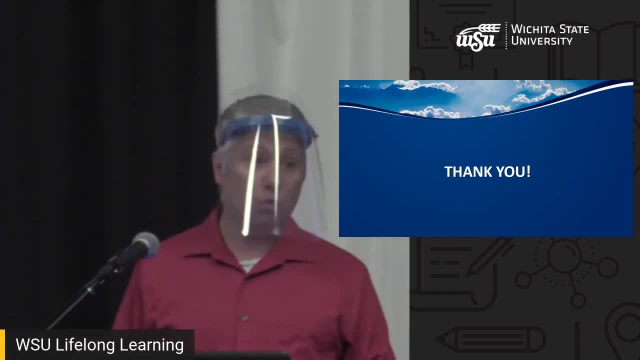 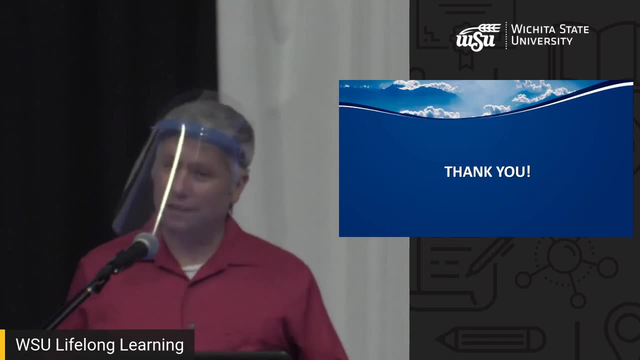 because we really just don't know exactly what the inputs are and what the outputs wind up being. Other things, Anything from online, Any emails, Oh my gosh. Yeah, Are you talking about like the dust winds? Those are dust devils. 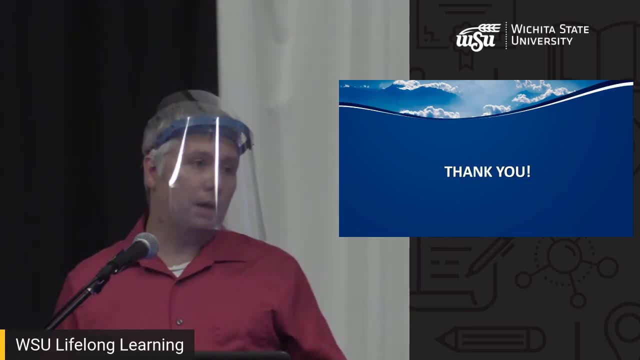 Dust devils are formed by just kind of unequal heating of the Earth's surface And it just kind of creates a just really small scale circulation. Most dust devils, you know you're talking a couple of meters in width, maybe going up 20 to 50 feet. 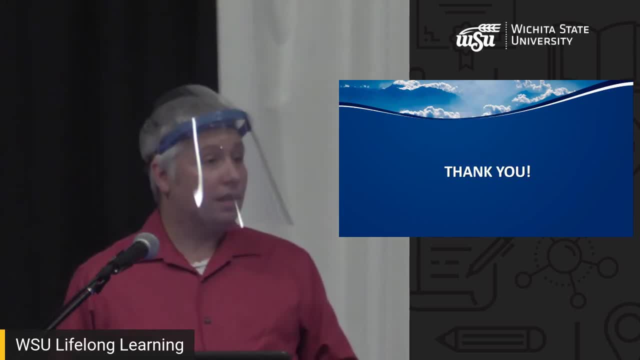 But in more extreme cases they can get. you know, they could get as strong as a F0 tornado, But that would be pretty extreme cases. But it has happened And in those more extreme cases that circulation probably gets a little bit wider than you know. 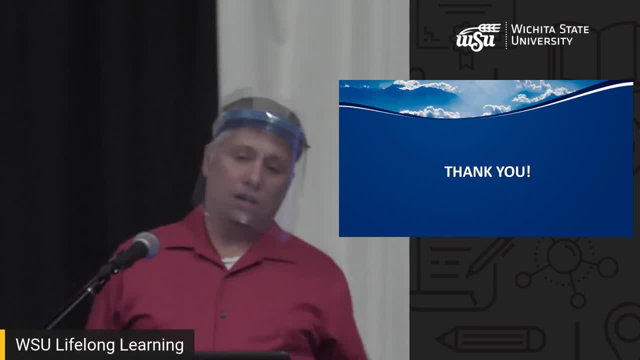 maybe the area kind of around me, out to the front tables, things like that- But goes up, you know, can go up a couple hundred feet, But usually with dust devils they pop up and they're pretty short lived. They're going to rotate counterclockwise. Now, in most cases, if they are in the vicinity of something that could throw off of their rotation, their circulation, they can actually rotate the other way. It's very, very rare. Another true thing is tornadoes can reverse their circulation too. But it is also very rare. It's less than 1%. I believe those are also going to be your counterclockwise turn. So yeah, you've got and I've been tornado. Those are especially a larger actual tornado tornado. 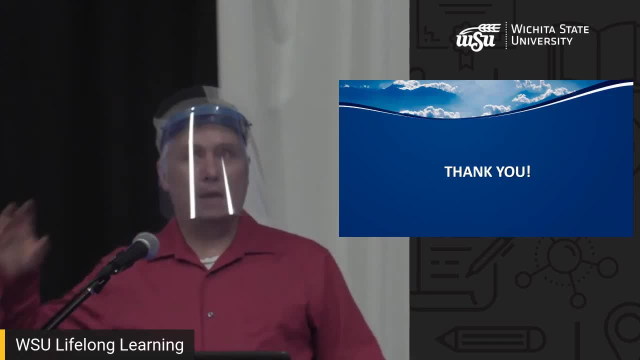 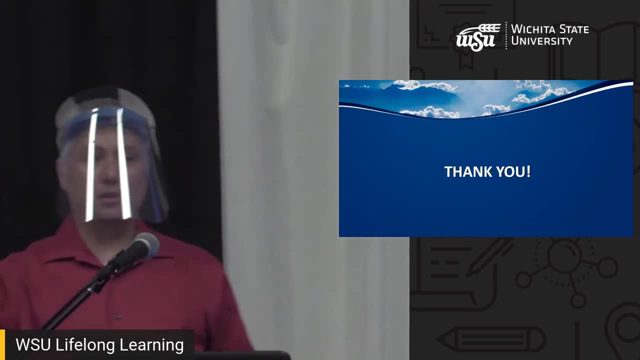 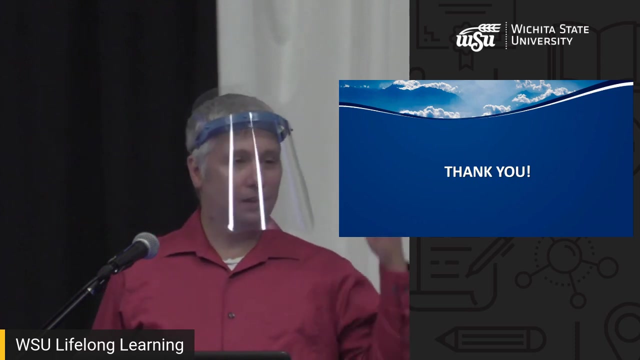 You'll. those are called suction vortices, And so you'll have your larger circulation of the main tornado And then within that tornado you kind of you turn up smaller, Not really tornadoes, but it creates additional circulations. And those circulations? will they turn counterclockwise the circulation itself And then they'll rotate around the tornado counterclockwise? Yes, There are. there's definitely some variants. That's another one of those items that does get measured and monitored. 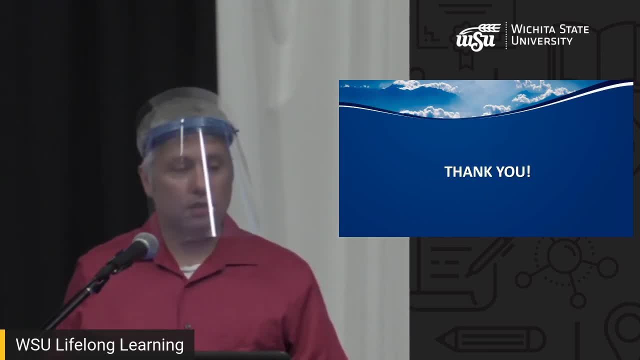 At least some of them do. via remote sensing, The satellites are able to measure some of that concentration. They also are measuring the thickness of the ozone layer and those concentrations And it- and just like with the ozone, you have it- the thickest around the equator. 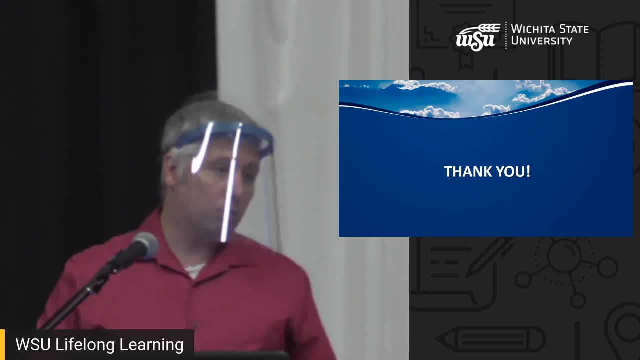 and it kind of gets thinner toward the North and South poles. You know there's concentrations, I mean. I mean all you need to do kind of is look at some of our more polluted cities across the globe to know that there is definitely places on the planet. 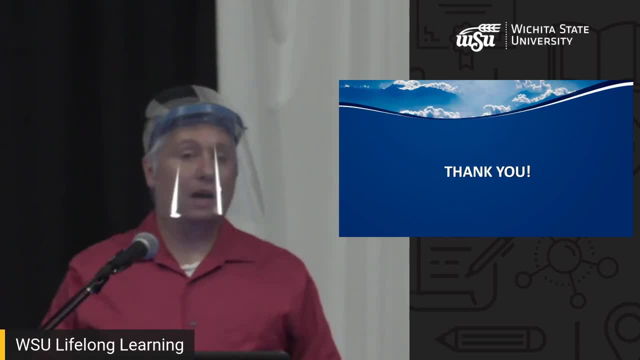 that are have a higher concentration of of atmospheric chemicals and pollutants that are definitely known Not good in terms of greenhouse gases. But again, as you move away from those points of higher pollution, you know it gets mixed in a little bit more. a little bit more, a little bit more. So the further you get from these- you know larger metropolitan cities and things like that- it it decreases in its concentration. I think I believe that that's primarily how it's done. 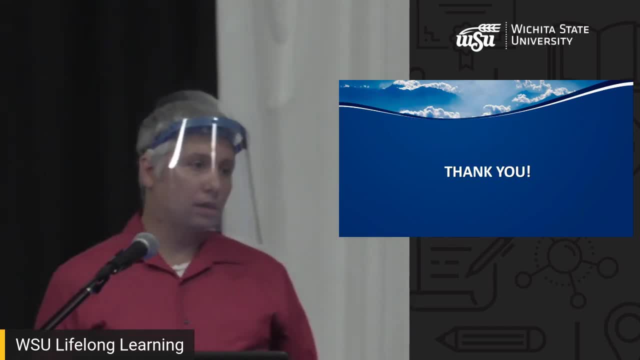 I mean, you have also point single point observations in terms of: I mean, you'll, if you look in your various weather apps, most of them have an air quality measure, which that's. that's not taking into account necessarily any one thing. 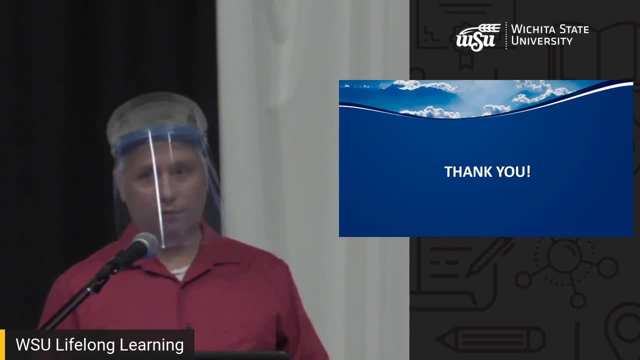 A lot of those are kind of aggregates from everything from you know, smog, pollution, things like that that may be in the air at the specific time They take into account. you know maybe how much you know what the pollen is in the air. Although a lot of times they'll do that as a separate index And then they'll also look at that in terms of how much mixing is there in the lower atmospheric layer? is you know there may be the same amount of you know. in your average city, you're going to be producing, at least Monday through Friday, about the same amount of pollution every day, But if there's enough wind circulation in the area, it mixes out more on some days than it would on other days. 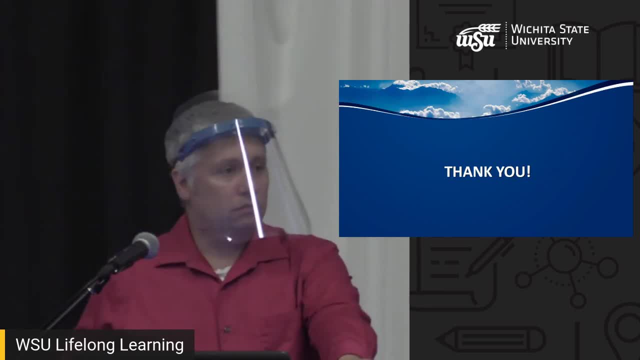 Other things, Yeah, All over the place, You know. yeah, When we were talking about the history on during the first class, we found that actually the US was not the first to set up a meteorological service. We were close, but we weren't the first. 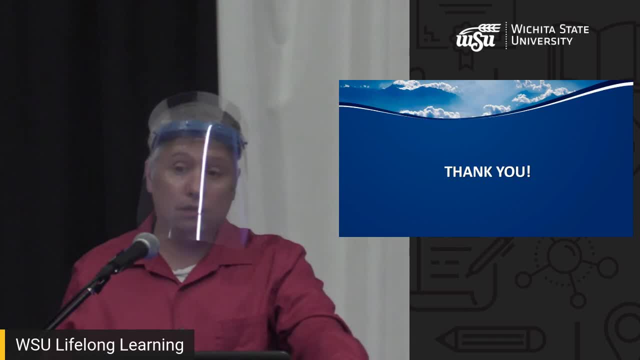 But we were probably the most ambitious here in the US And that's the reason why We have a very, very concentrated network of observing stations. Another reason for that, for the concentration of observation stations, kind of, goes to the development of numerical modeling. 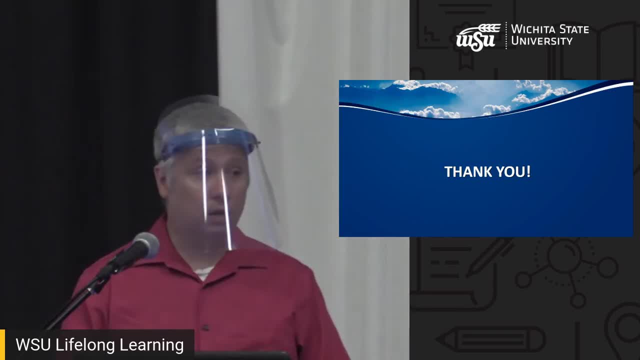 which, not exclusively but in large part, kind of started here in the US. Well, you know, one of the more famous- you know we brought his name up in that first class researchers in the early 20th century- was Richardson. 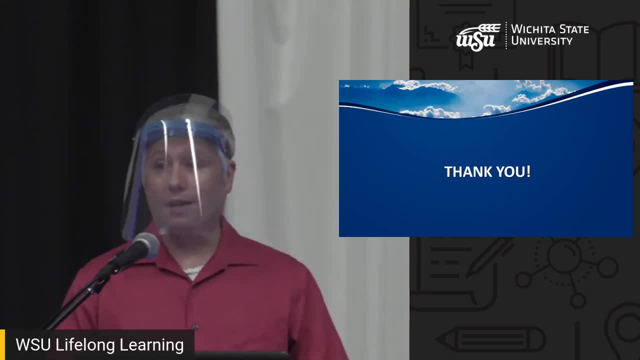 And Richardson was the first one that basically said: hey, if we have enough data, if we have enough physical numbers, we can put it into a model and just crunch all these calculations and figure out what's going to happen in the atmosphere. Well, that led to. 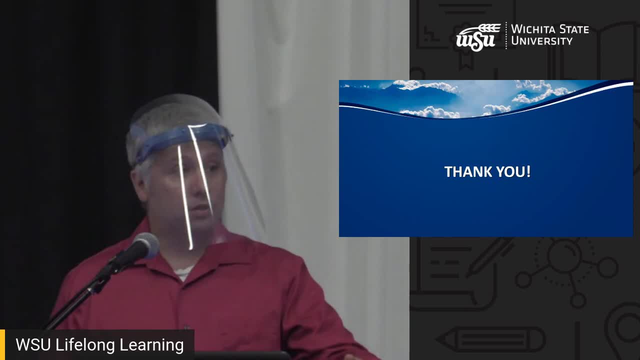 or helped to lead toward a push to install as much- you know- weather equipment as possible, to get it, as you know, concentrated and focused as much as we could so that we could get enough data in. Now, of course, we're just now kind of getting over the last about 30, 40 years, into the window in which we have computing power strong enough to actually crunch those numbers in an amount of time that is reasonable for forecasting Other parts of the world, even other parts of the industrialized world. 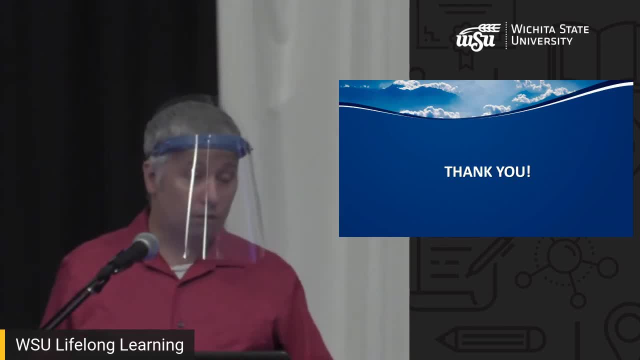 they don't. I mean, they're there And in some respects they're even better than we are. Like good example is the ECM, the European computer. their model is considered. out of all the numerical models out there, it's the best one. 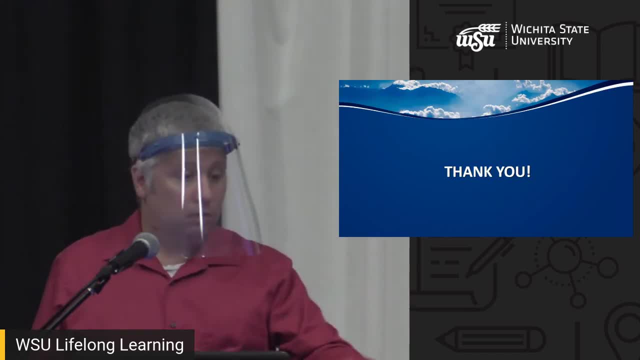 But you know they're still behind where we are in terms of having the same level of concentration, in terms of monitoring the Earth's surface with physical equipment. Other parts of the world fall even further behind, but we're able to make that up now with the. 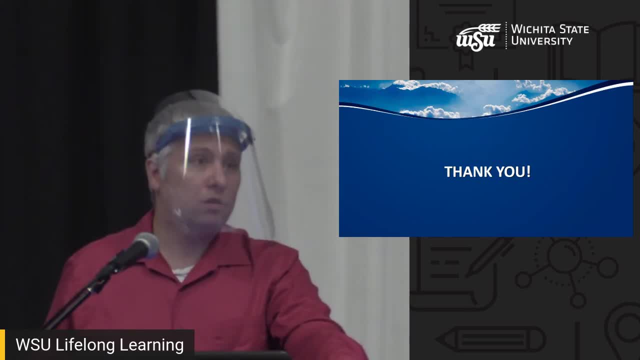 with the weather satellites that are up there. I mean that helps quite a bit in terms of being able to get us better data that we can process into those numerical models and just really increase our overall understanding of what's going on at the surface and in the atmosphere at any given time. 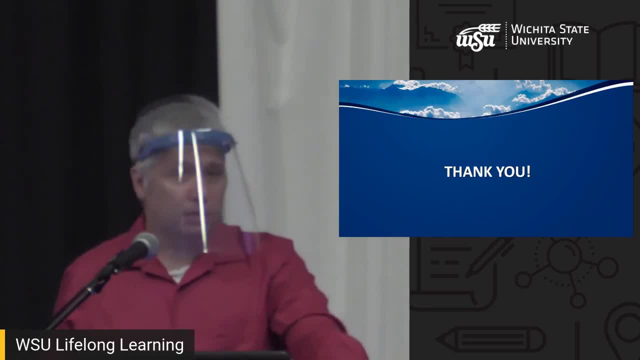 across the entire planet relatively at the same time. Other questions: Well, you guys have been a pleasure. I do have about five, seven minutes that I can stick around, and then I'm going to have to jet out, as I indicated, pretty quickly. 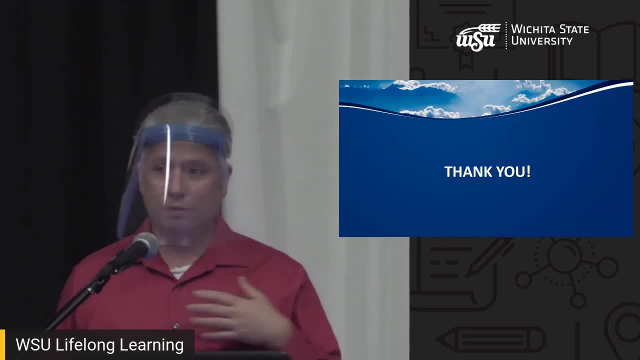 If you don't get, aren't able to touch base with me, you know, send a follow-up question or whatever into the Lifelong Learning email and I will get to that as quickly as I can. And then, for those of you who are thirsty, 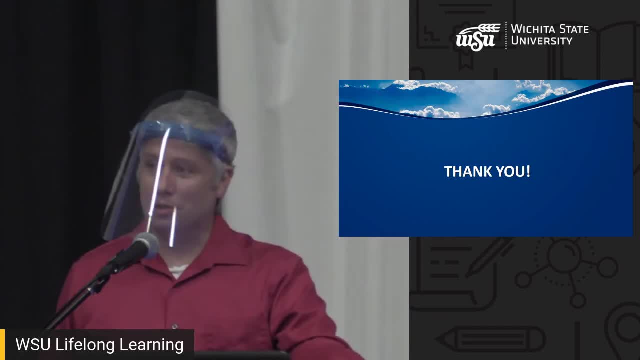 my day doesn't end when my work at Wichita State gets over, because my bartender tonight isn't going to be there, So I'll be working the bar at Augustino Brewing tonight too, So if you've got questions, you can find me there as well. 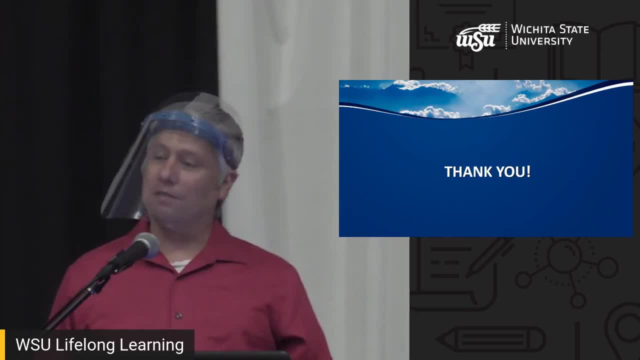 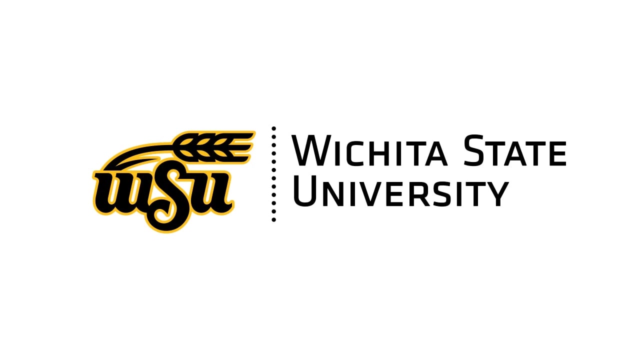 So thanks a lot. You've been a pleasure And I encourage you to continue learning about this and many other topics which the university has quite a few of in this program. So thanks, Thank you.